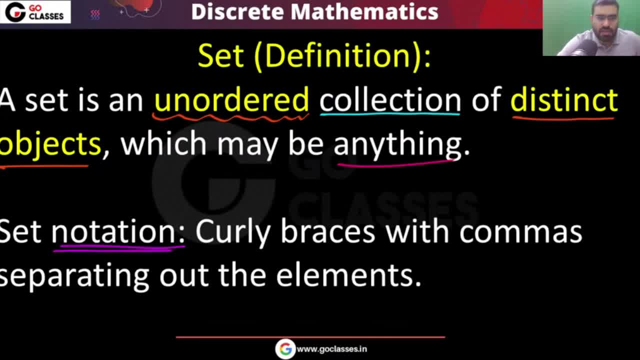 What is the notation? What is the notation we use for set? For the set, we use the notation where we put all the elements in the curly braces and they are separated by the comma. Okay, so this is what we do: all the elements that you have in this collection, you put them in curly 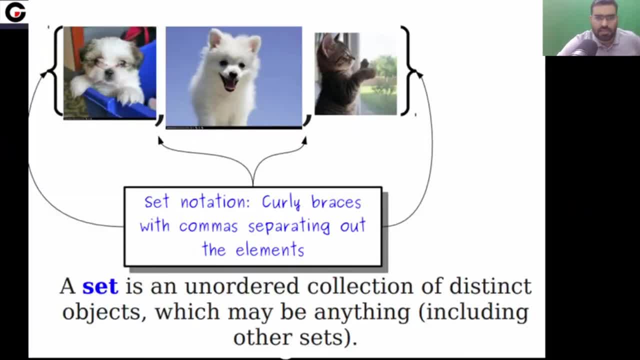 braces and separate by comma. So let's take example. See, you can see this example. This is a set in which you have three elements: There is a cat, there is a puppy and there is another. whatever, this is another puppy. So you can notice there is a cat and two dogs. So this is a set in which you 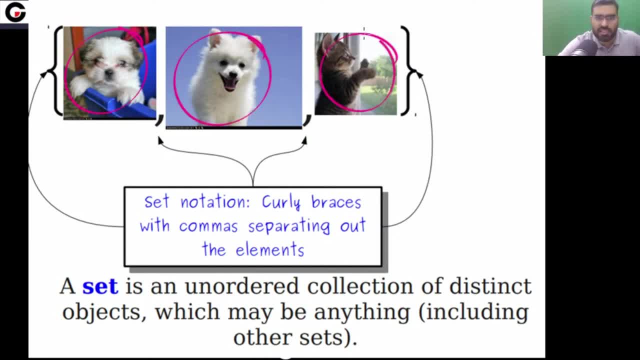 have three elements And you can notice all the elements. These are the elements, These are separated by comma And these elements we put in the curly braces. So this is how we represent a set. Okay, so very simple. set is an unordered collection of distinct elements, means the. 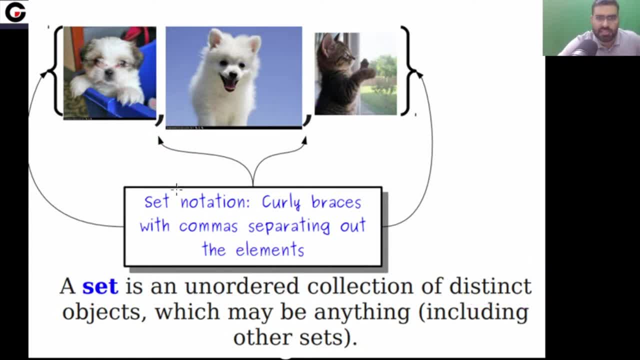 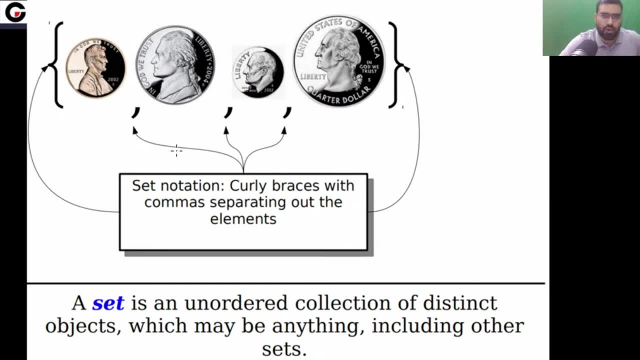 elements cannot repeat like here. You can notice there are three distinct elements, three different elements. We put them in a curly braces and we separate them by comma. This is another set in which you have four elements. You can check. all the four elements are different. So this for this. 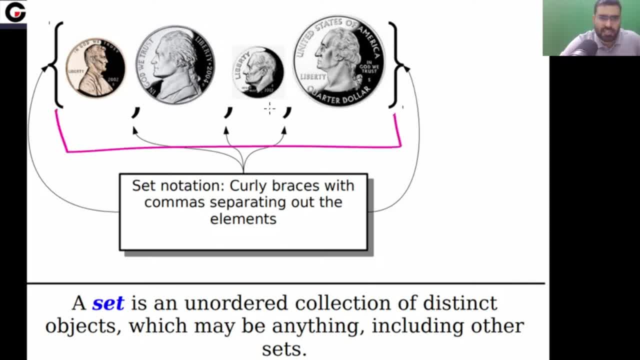 set the cardinality is four because there are four elements in this set. So we say that cardinality of a finite set this is a finite set because only four elements are there, So this is a finite set. Cardinality of a finite set is number of elements in that set. So you can see these are the elements. 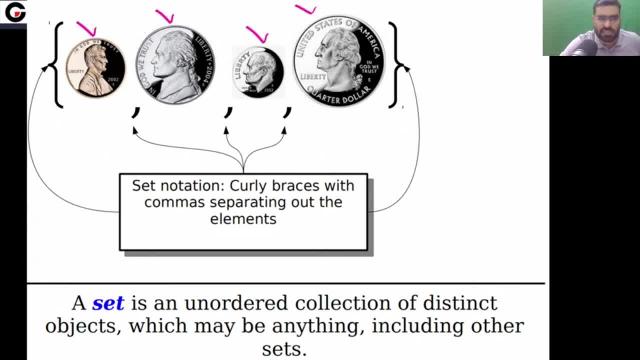 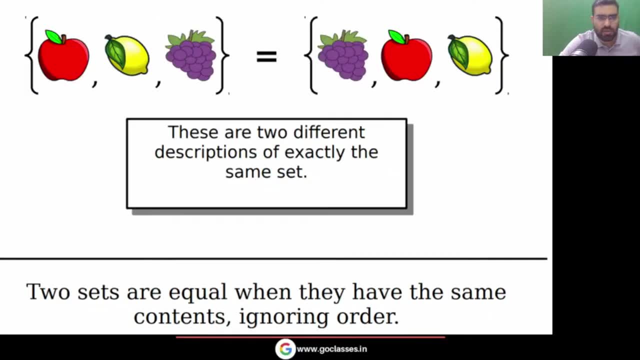 This is element, element, element, element. So there are total four elements in this set. They are separated by comma and we put them in the curly braces. This is the notation. This is the set notation. Now, let's see this. As I told you, that in a set order does not matter. 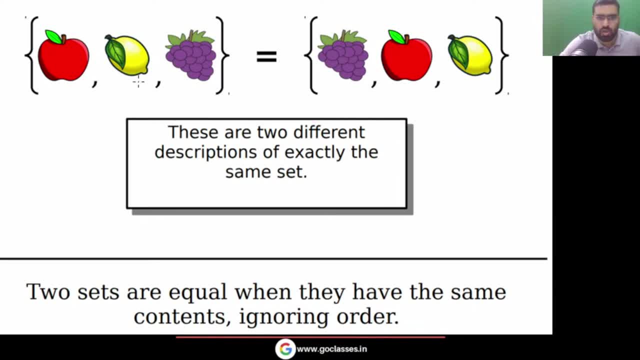 So this set is exactly same as this set, because order does not matter In this order, in this set, order does not matter. also, you have the same three elements, those, those same three elements you have here. so remember, in these two set, in this set, in this set, you, you have the exactly same elements, exactly same number of. 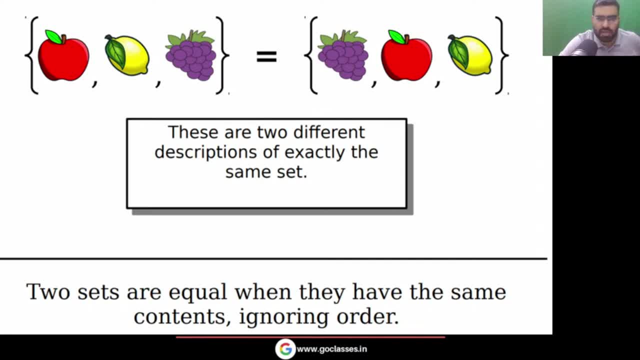 elements. so these two set are basically same. order does not matter in which order you put these elements, that does not matter. you can put the apple here, you can put the apple here. that does not matter, because set is a collection of unordered elements. so you can see, these two sets are: 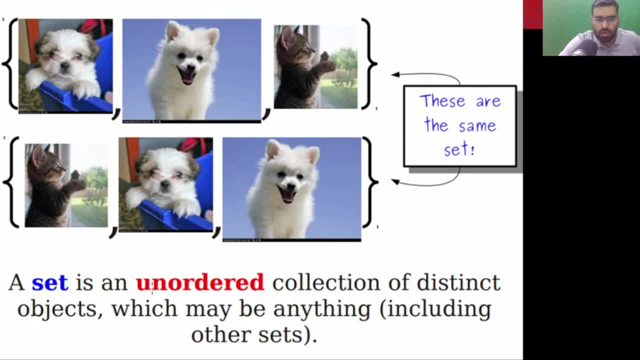 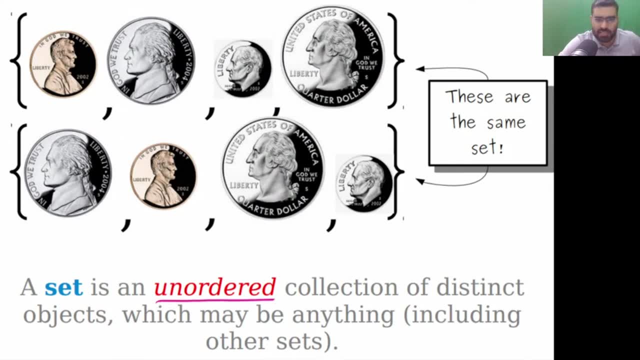 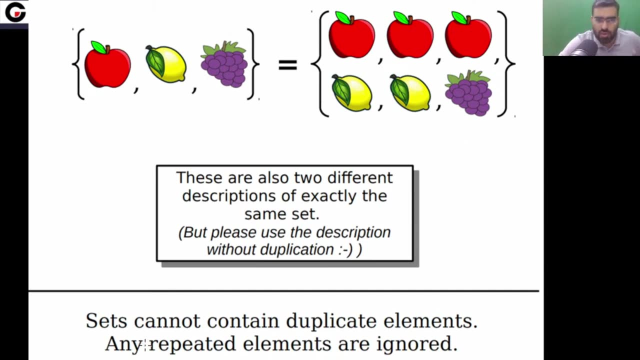 basically same because order does not matter, so unordered, as I told you, this is a important point. another point: you can see these two set are same because set is collection of unordered elements. next, you can see these two set are same because we ignore the duplicate. duplicate is not allowed, okay, remember. 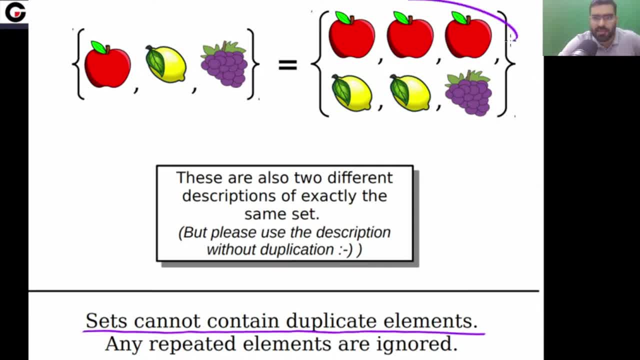 set cannot contain duplicates. so these duplicate elements that you have, these are ignored. you can ignore them. so, basically, this set and this set are basically same. remember, these two set are same. so here, one thing, one point. I want to ask: if I give you this set, what is the cardinality, what is the? 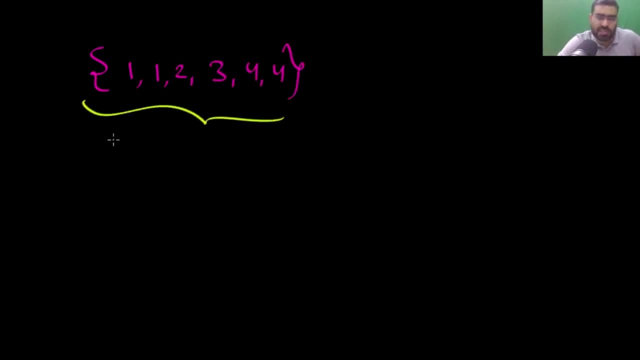 cardinality of this set, for this set. how many elements are there? tell me in this set, how many elements? I have given you a set in which you have some elements, how many elements you have in this set total, how many elements so you can see in this. 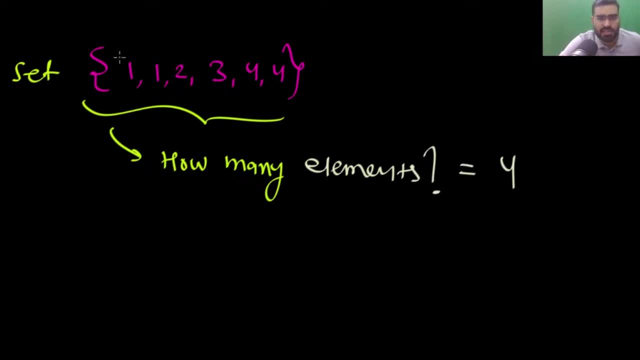 set total only four elements. we have. remember we have because, as I told you, we ignore the duplicate. you are not allowed. this set is at this set and this set. they are basically same. so this set is exactly same as this set because we ignore the elements. so number 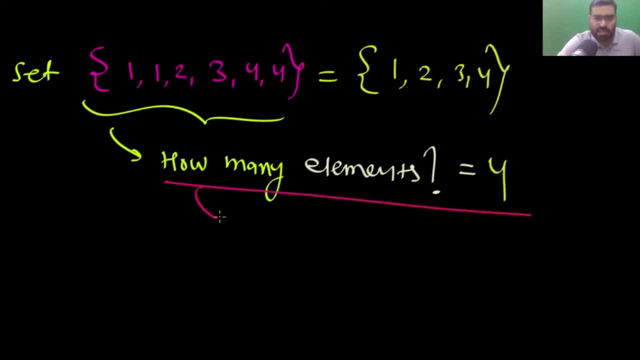 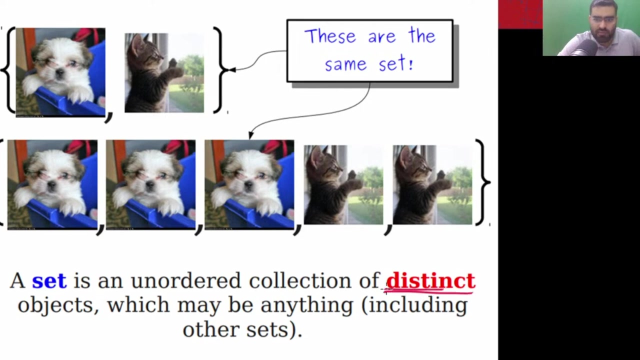 of elements is only four and this number of elements in a finite set. this is called cardinality. so the cardinality of this set, that is basically for for this set, the cardinality is for now, let's move on. you can see these two set are same because duplicates do not matter. set is a collection of distinct elements. 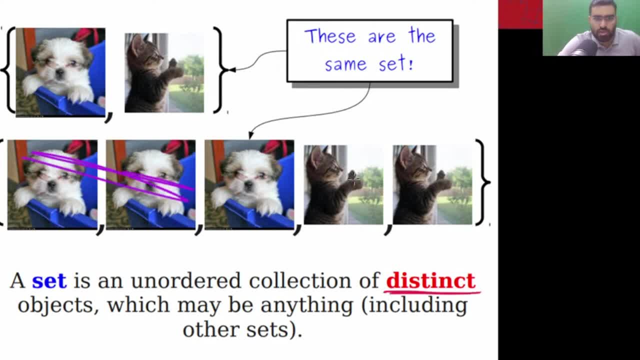 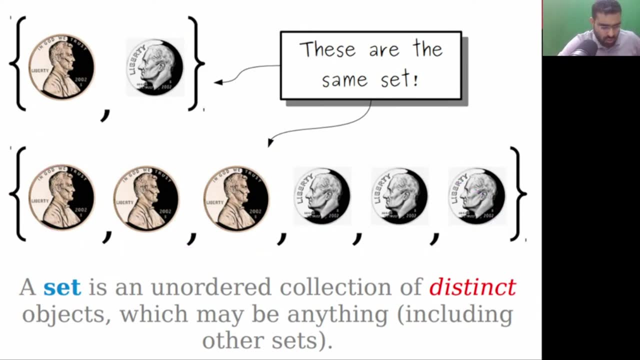 so duplicate duplicates. we ignore all these duplicates you can ignore. okay, so these two set are basically same and the cardinality of this set is to remember only two elements we have in this set. now let's move on. these two set are same. in this set, only two elements you have. ignore the duplicates. we ignore the. 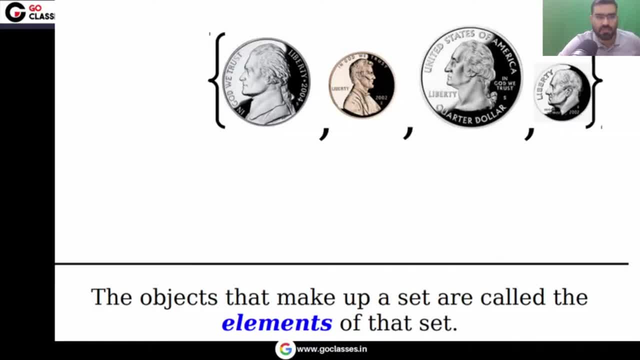 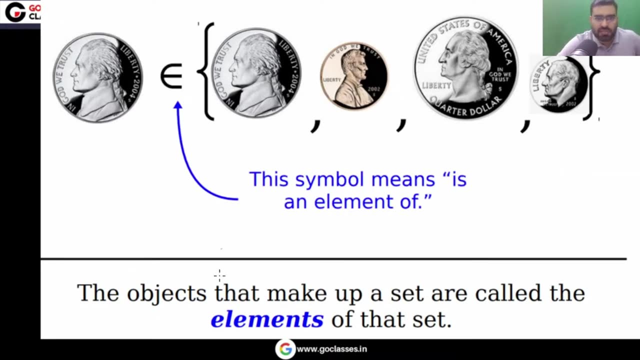 duplicates. duplicates do not matter. now, let's see. so the next is: you can see. so ultimately, you can see that this is a set. in this set, you have total four elements. the cardinality of this set is four. now you can easily see that if i give you, for example, look at this set i give 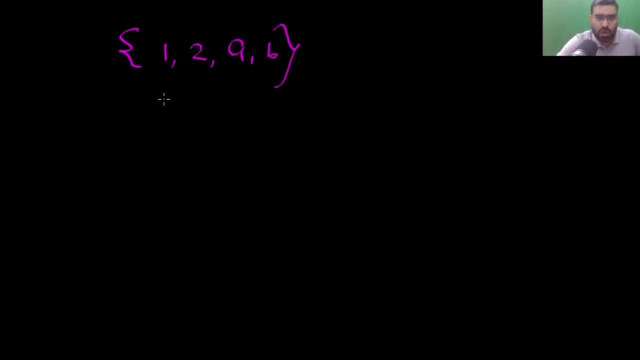 you one, two, a, b. in this set you can notice a belongs to this set. you see, set is a collection. you can consider this as a set or you can call it a collection. now, set is a collection, so this is your set, this curly braces. remember, within the curly braces, everything that is a element, so you 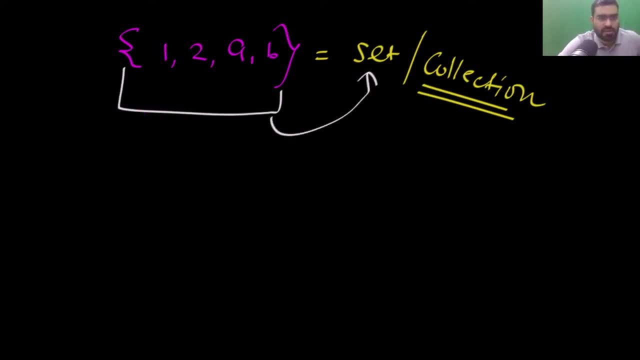 can see. this is element, okay, clear. so this is element. so let's call this set s, so i can say: this is element of s, okay, so that is the reason i can say this one: if you look at this one, this is this belongs to s, so this symbol we use. it means belongs to, it means belongs to, so this symbol. 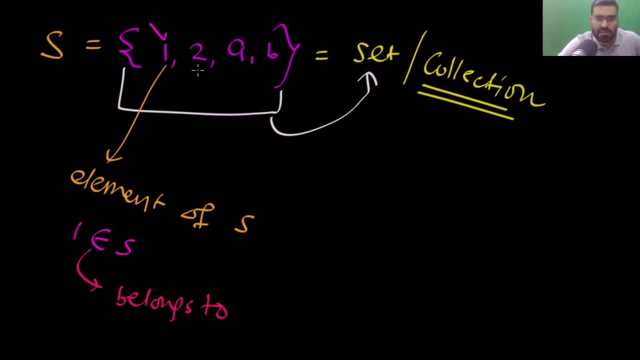 means belongs to means. one belongs to this set. one is in this collection. you can easily see three does not belong to this set. we don't have three in this collection. we don't have c in this collection. we don't have uh john in this collection. so these things we do not have in this collection, but you. 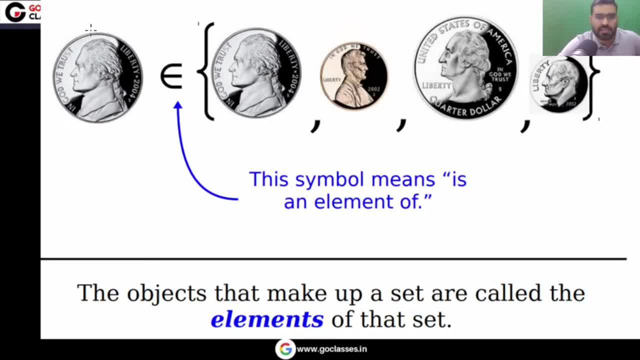 can notice b is in this collection. similarly, you can notice that this element belongs to this collection because belongs to this set, because you can notice this is already an element in this set. so this symbol means an element of all. right. I can say belongs to, so this is an element of this set. now let's move on. you can check that. 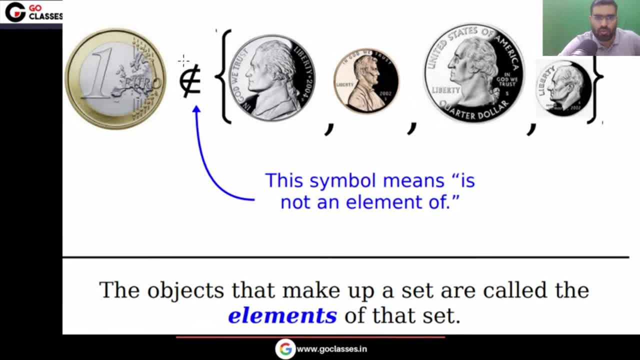 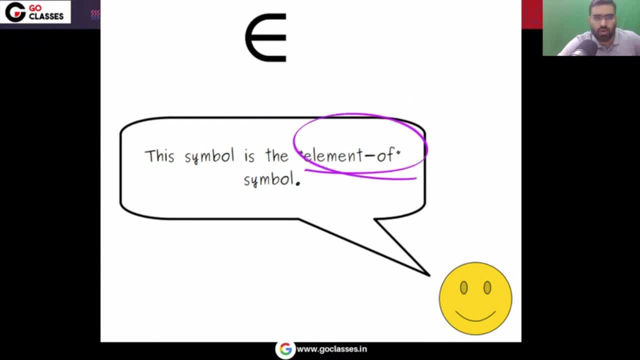 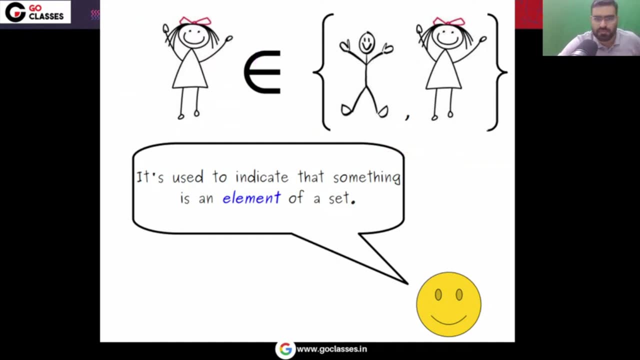 this is not element of this set. so basically it means: does not belong to, is not element of this, is not element of now. so this symbol means element of now. as you can see, this girl is the element of this set, because this girl belongs to this set. but you can notice, this dog does not. 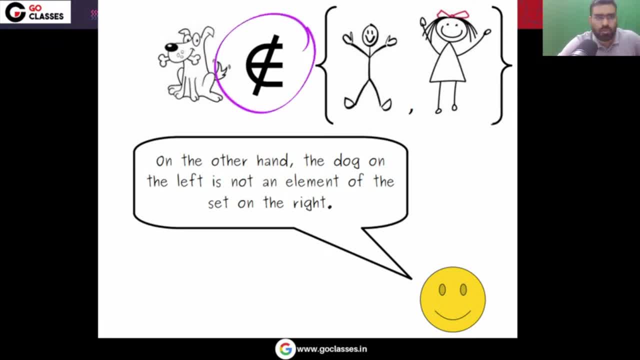 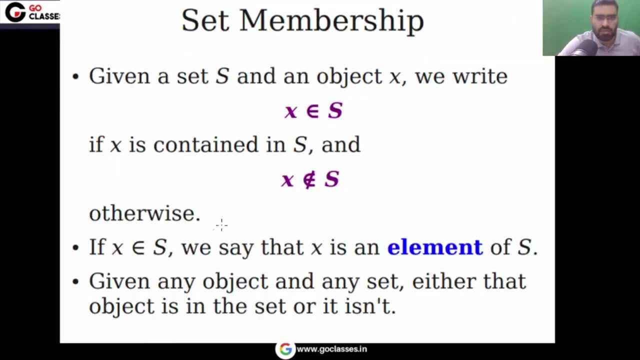 belong to this set. okay, so i can say this dog does not belong to this set and this girl belongs to this set. now let's move on. so finally, uh, we understood that some element can belong to the set or it it may not belong to the set. so you can easily see. now, very important thing i want to tell. 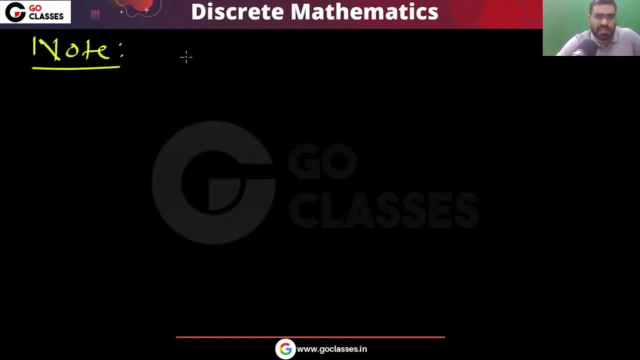 you. this is important- that if you have a set s, if you have some collection- as set means this is some collection- in this collection you have some elements those are separate from the set, separated by the comma, some elements you have now for any element, for any, for anything, for any a. 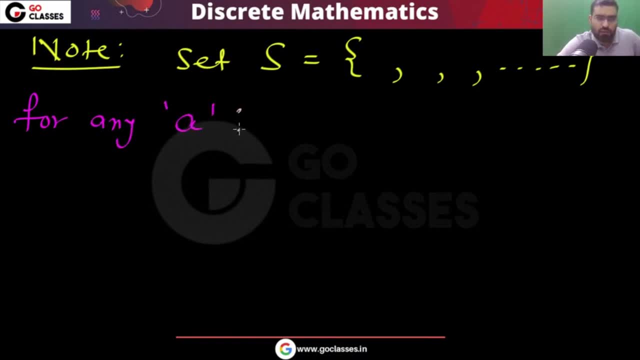 now, this a can be anything. remember this. a can be any element. so for any a, only two possibilities are there. what are the possibilities? either this will belong to this set, either this is an element of this set in this collection, either this a is element, or or- what can happen, this is not an. 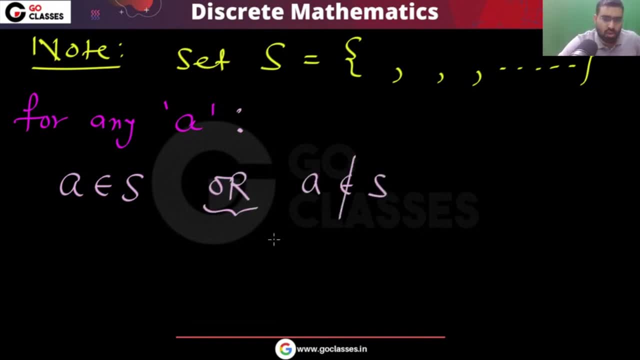 element. right, either this is element of this set or this is not element of this set, either. this very important that either this will happen or this will happen, but not both. okay, it cannot happen that and this a belongs to the set also, it does not belong to the set also, but not both. so this is a simple point I want to tell. 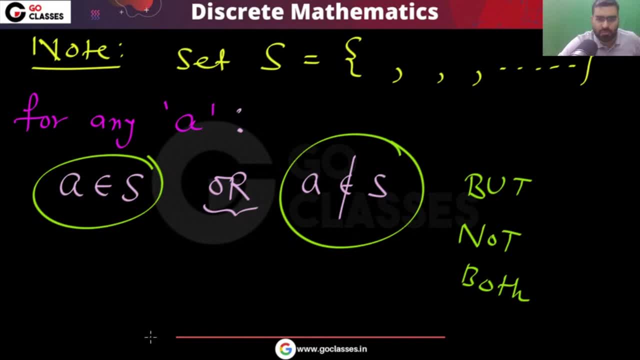 you that it cannot happen that both of them are true. okay, so if this happens, that if this happens, let me, as you, let me assume this happens- that a belongs to the set and it does not belong to the set. a belongs to the set and and it does. 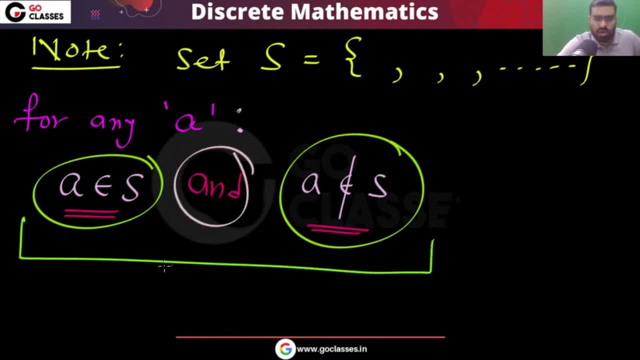 not belong to the set. this type of situation is called con paradox. this type of situation is called paradox because it it simply means that a is here also and a is not here. so this type of situation is called paradox. remember, or you can say, this type of situation you. 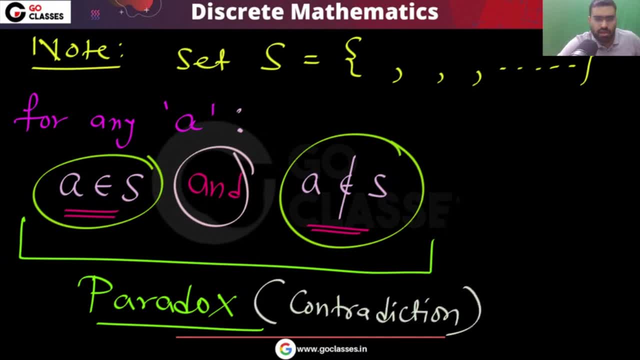 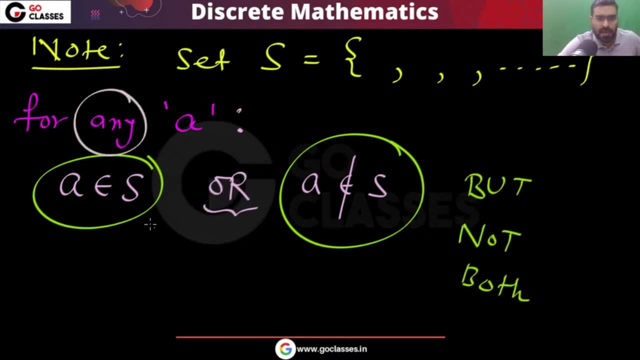 can call contradiction. so so, ultimately, i am saying that whatever for any a, whatever a you take for any a, this will happen: that either it will belong to the set, either it will be element of this set, or it will not be element of this set, but not both it cannot. 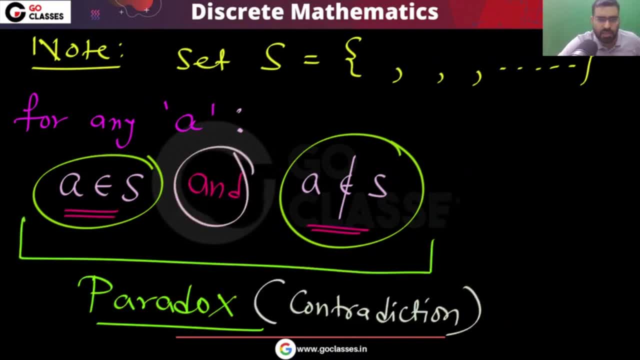 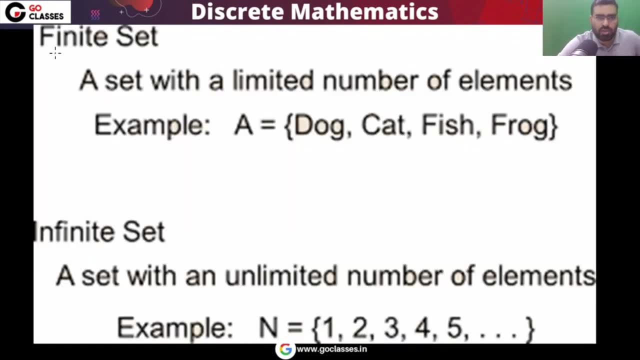 happen that both of them are happening together. if both of them happen together, it means it is element also. it is not element also. that is called paradox or you can say, contradiction. so, as i told you, there are two type of set. one is finite set, another is infinite set. 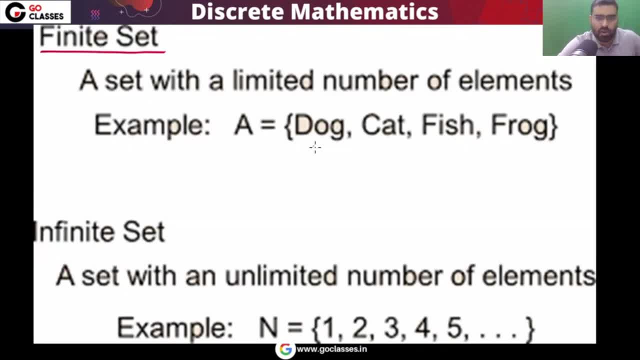 infinite set means infinite number of elements. finite set means finite number of elements. this is a set in which you have four elements, so this is a finite set. and this is a set in which you have infinite number of elements, so this is a set in which you have infinite number of elements, so this is a set in which you have. 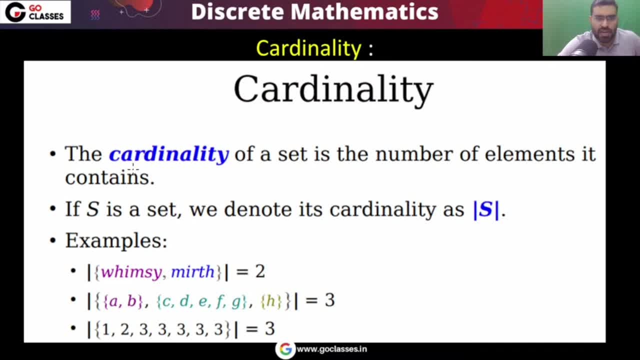 infinite set. so there are two type of set. now you can see what is the cardinality of a finite set. cardinality of a finite set, remember cardinality of a finite set, that is number of elements, how many elements we have in this set. so cardinality of a finite set is the number of elements in that. 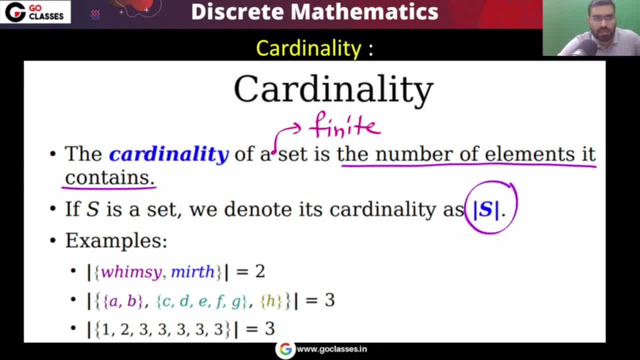 set. so and we denote by this symbol this is the symbol we use. this symbol means what this means. this means cardinality of s, cardinality of set s. so if s is a set, then we denote cardinality as Cardinality of S, For example, for this set. this is a set in which you have two elements. 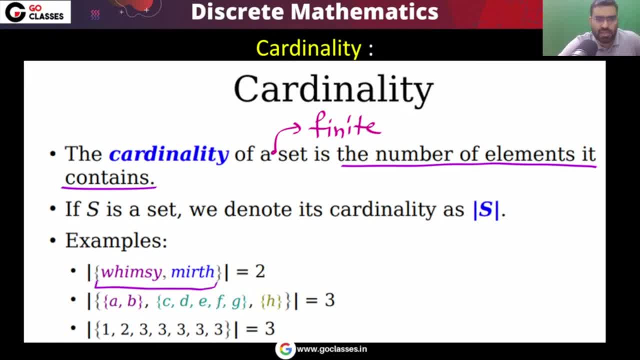 These are the two elements. this is an element, this is an element. So the cardinality of this set, you can see, cardinality is 2.. For this set, the cardinality is 3.. Repetition does not matter. 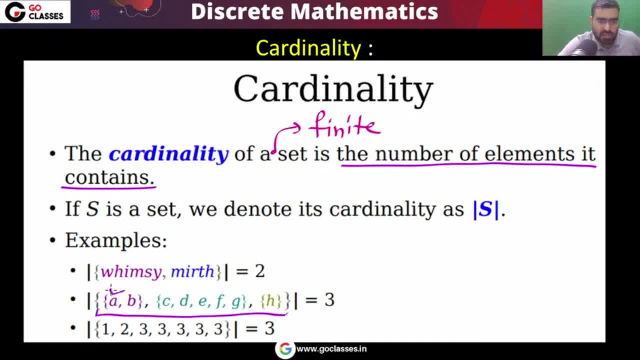 For this set. look at this set. the cardinality is 3.. Because this is element, this is element, this is element. Okay, you can notice that every element is also a set. So you can easily see: this is our set. 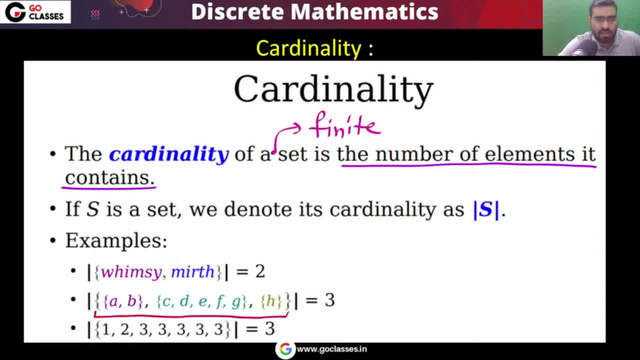 For this set, the cardinality is 3.. Because there are three elements: Element 1, element 2, element 3.. Every element is a set, Like this element is a set. this element is a set. this element is a set. 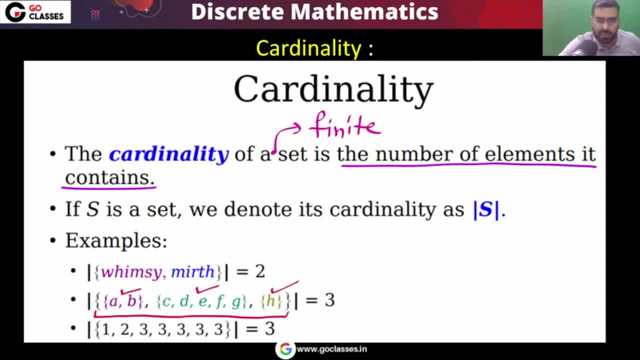 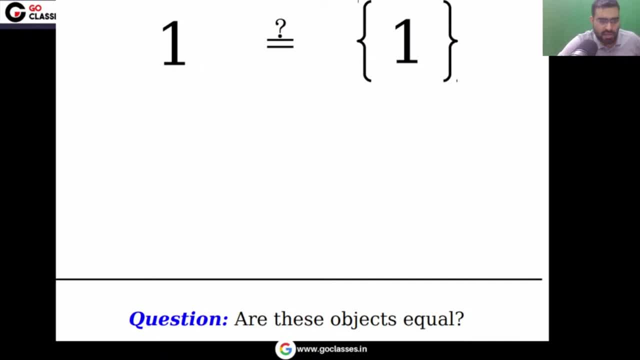 And that is fine. there is no problem. Okay, element can be set, Or element can be simple. No problem Now. so this is the concept of cardinality. What about this? Are they same? Are they same? Are these two objects equal? 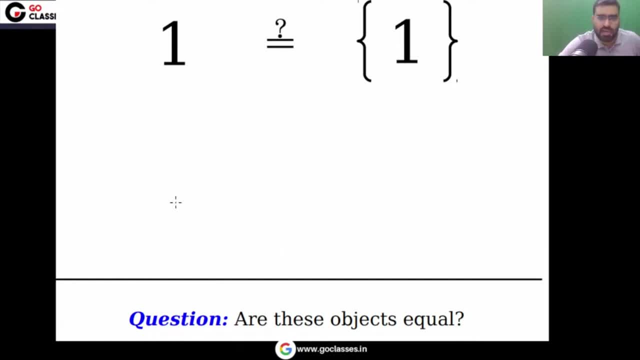 Look at these two objects and tell me: are they equal? So the answer is no. See, this is a number, right, This is a number. This is not a collection. This is a number. This is not a collection. This is not a collection. 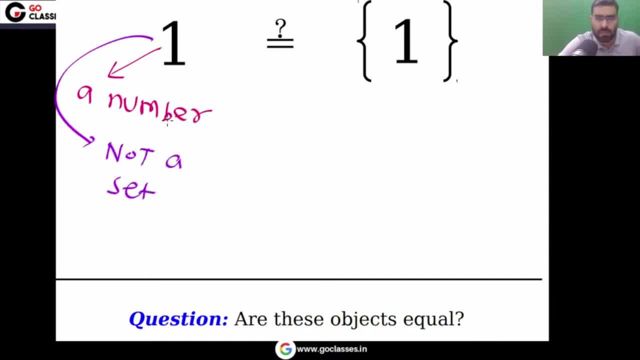 This is not a set. This is a number, Number 1.. But this is a set. This is a set which contains number 1.. Okay, so this is a collection. This is a box. You can think that this is a box. 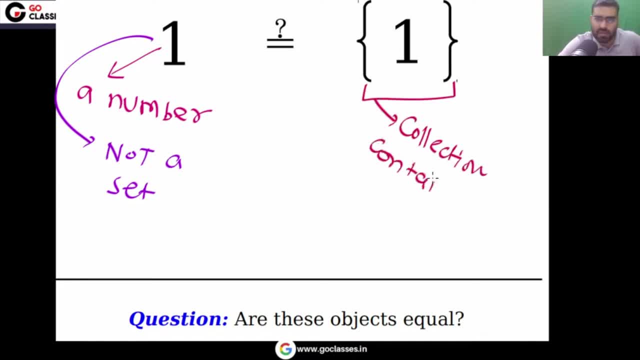 This is a collection containing one element Containing one element. There is one element in this set, set okay, and that containing one element, and that element is one containing one element and that element is one. so, remember, you can think that this is a simple number and you can think that this as 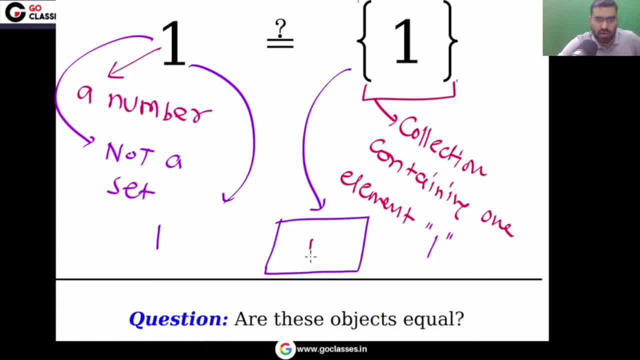 a box. you can think that there is a box in this box, there is this one. so remember, these two things are not same. so you can think this set as a box, you can. you can think this set, you can think as a box in this box, you have one. so these two things are not same. remember, they are not same, as i told. 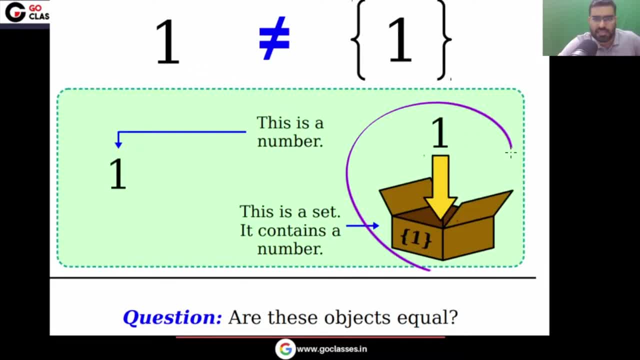 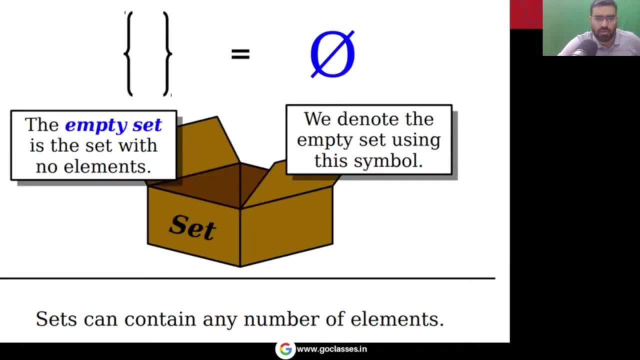 you. so this is just a simple number and this is a set which contains this number. now, as i told you, set you can. you can think about set as a box. now you can notice if your box is empty. if there is no element, then it will be called empty set. empty set means a set without any elements. so 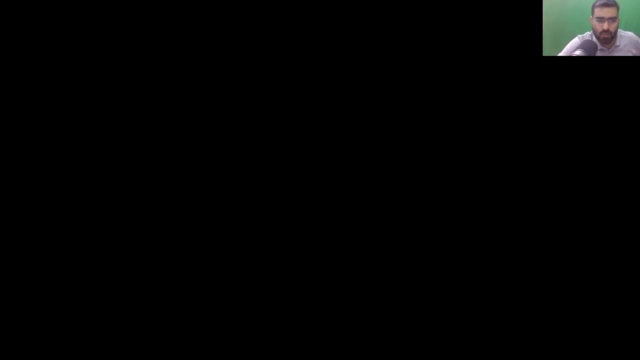 there are no elements. this type of set we call empty set. so if your box is empty, remember, if your set is empty, this is your set. this is your set. okay, you can think of it as a box. in this box there is no element. so this type of- okay, i can say it is like empty box. in this box there is no. 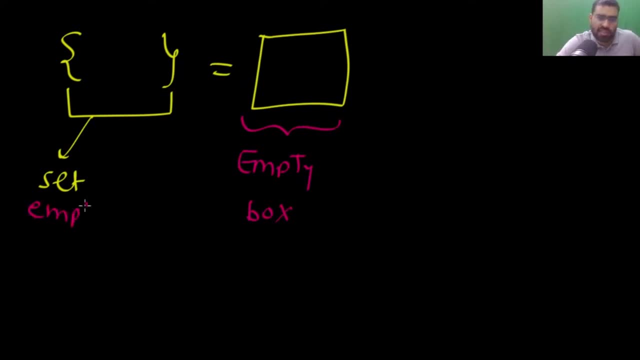 element in this and this is: this is your empty set, this is a set which is empty. so you can see, there is no element and we denote. we denote this, this thing, we denote by this symbol phi. so this symbol, we call it phi and what it means. 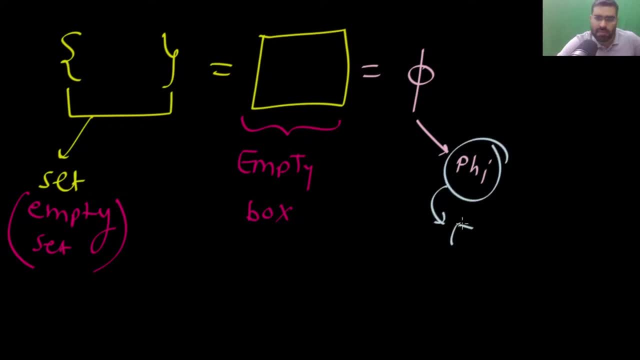 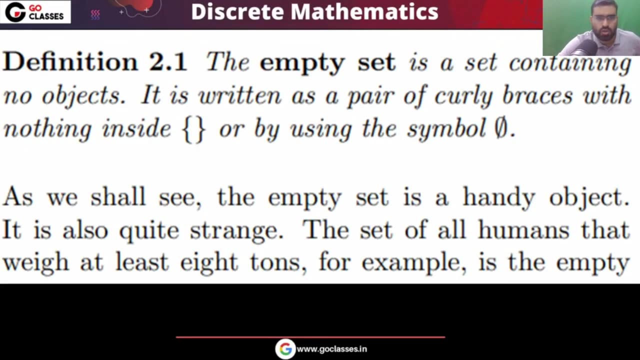 it simply means means that it simply means that empty set, okay. so this empty set, this empty box we denote by the symbol phi. now let's move on. so empty set means there is no element in this set. okay, that is called empty set, like, for example, the set of all humans whose weight is at least eight tons. 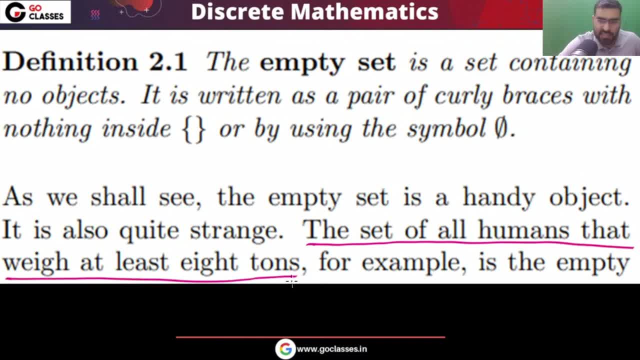 how many? how many elements are there in this collection? tell me how many elements? the set of all humans, the set of all humans whose weight is eight, at least eight tons, so of course that is an empty set, right? there is no element in this. there is no human being whose weight is eight. 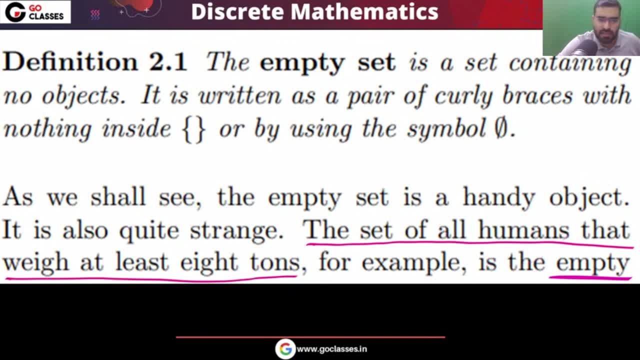 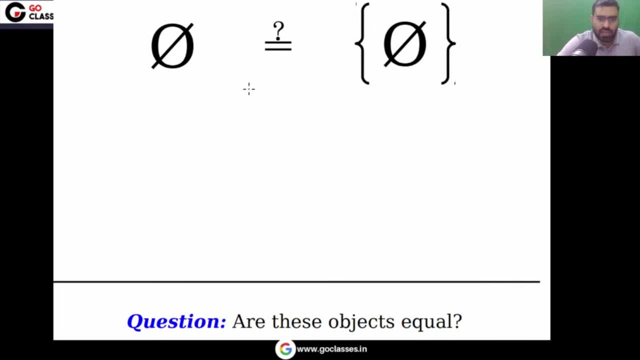 ton means eight thousand kilogram. of course, there is no element. okay, now let's move on. so let's check it out. so are these two same? look at these two objects. are these two objects same? these two objects are they equal? the answer is again no, because they are not equal. 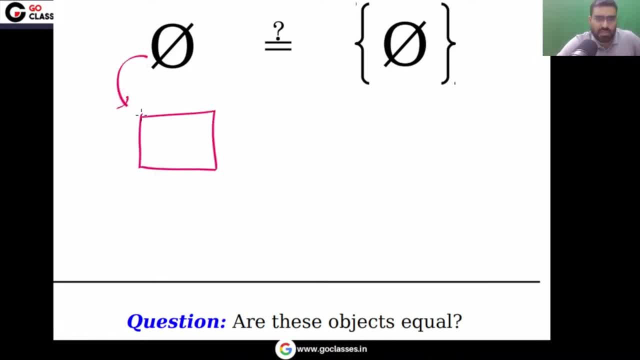 same, you can notice that this is your empty box. this is empty box in which there is no element. this is a box in which you have empty box. this is a box in which you have empty box. okay, are you getting my point? so these two are not. 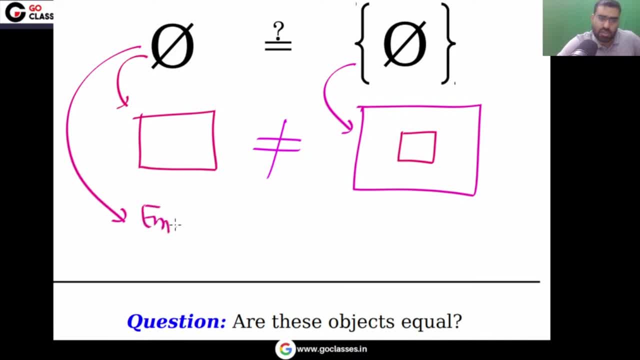 same. so remember this is empty set. this is your empty set, but remember this is not empty set. this is a set. this is not empty. this set is not empty set. in this set you have one element. this has this element you have in this set. in this set there is a one. 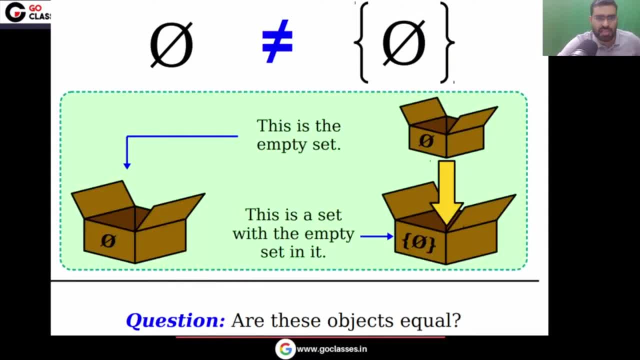 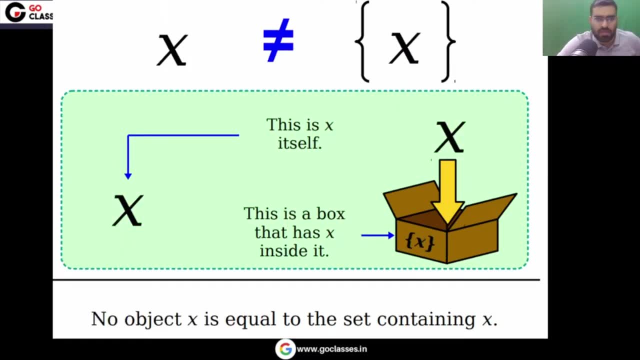 element. remember, this set is not empty, so these two things are not equal. as i told you, this is an empty set, so in this box there is nothing. in this box you have another box, okay? so, as i told you, no element is equal to a set containing this element. so this x, if this x, so this x is not equal. 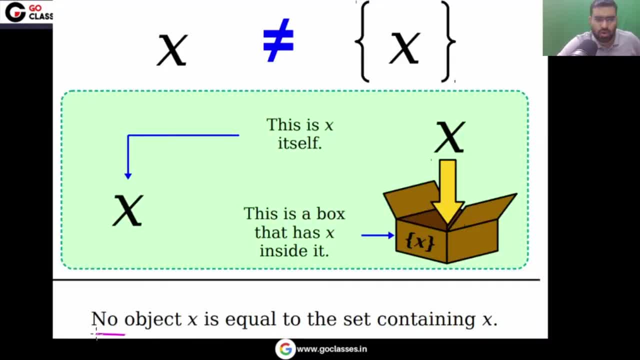 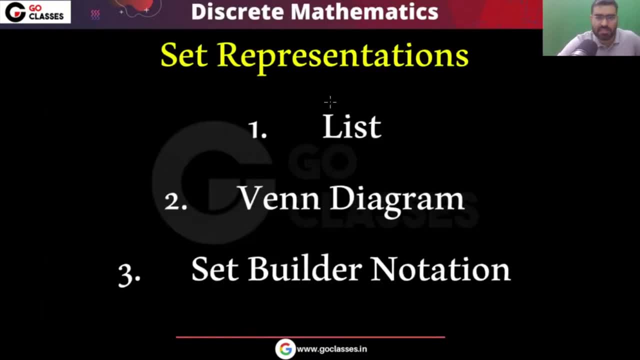 to set containing x. as you can notice, no object x is equal to the set containing x. so this is something important. now let's move on. what are the set representations? how many ways you can represent a set? there are many ways. for example, you can list all the elements like, for example, this: this is list representation. you are 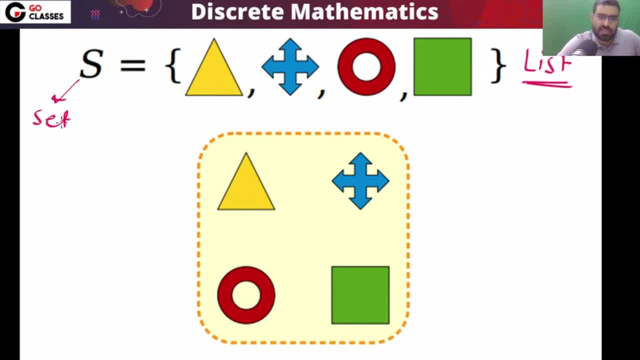 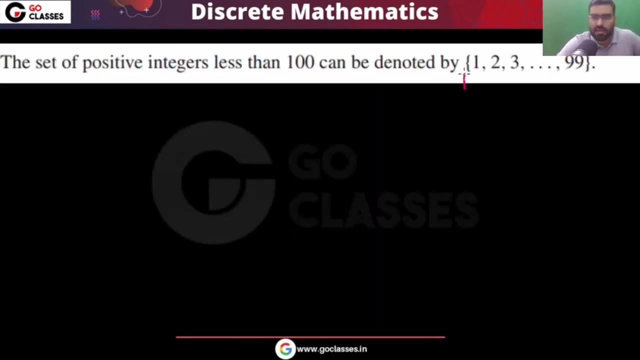 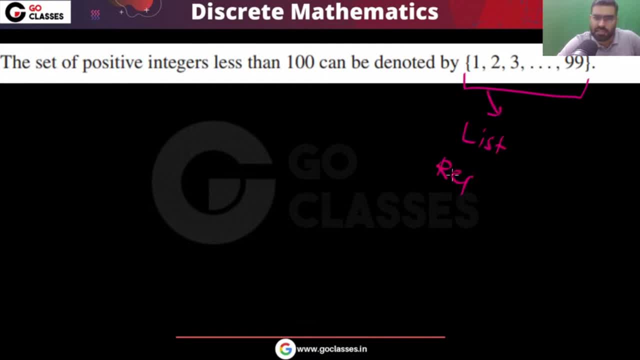 say: this is list representation of this is the list representation. you are listing all the elements, all the elements you are writing like which elements you have. okay, you are giving their explicit, uh, notation, you are giving their explicit representation, every element. you are telling that in this set you have one, you have two, you have three, you have four, five, six and ninety nine. 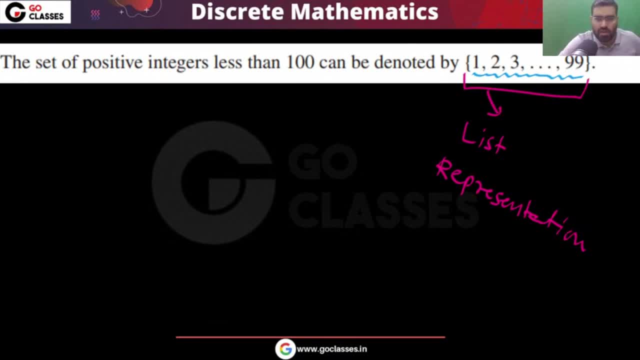 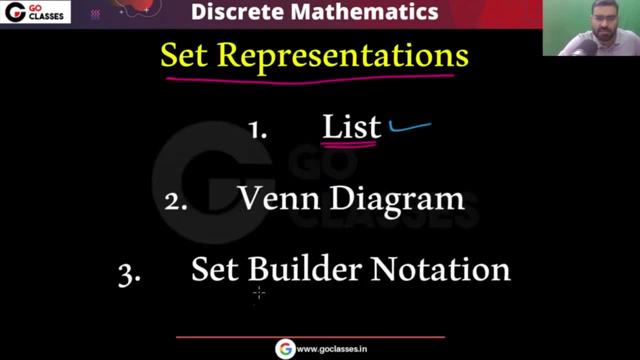 you don't have 100, you don't have 0, you don't have minus 1. now let's see, this is called venn diagram representation. this is another representation which is called venn diagram representation. as i told you, this is another representation. this is very simple, that basically. 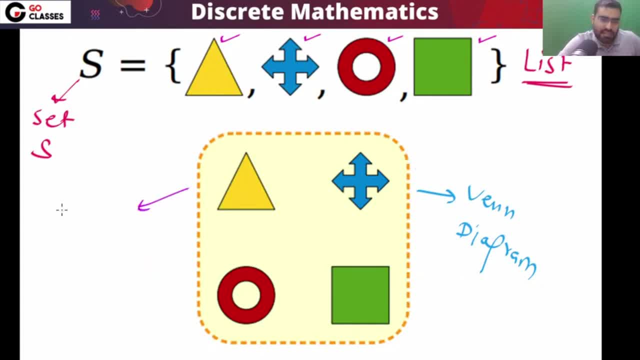 just make a box. this is, i can say, more friendly. right, this is more understandable, okay, like, even if you show this to any person so they can also understand it. so this is more understand. uh, understandable. okay. this it is very user friendly, i can say: okay, so this event diagram. 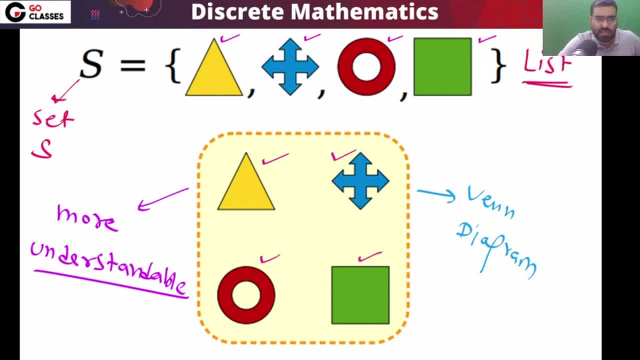 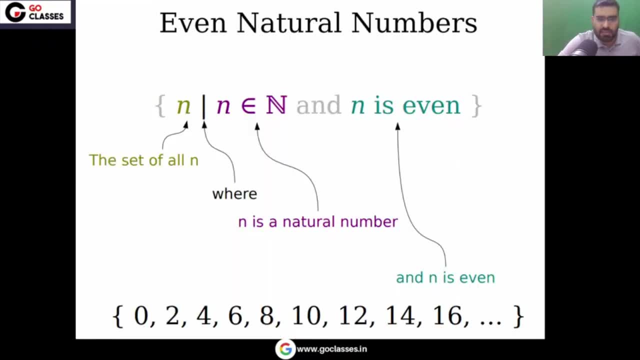 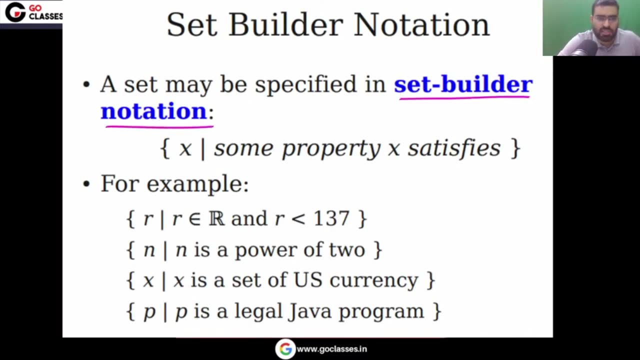 that you have total four elements. this is element. this is element, element, element. so there are four elements. now there is another representation. that is set builder notation. it simply means that some property you are satisfying- okay, some property you satisfy- this is called set builder notation. in the set builder notation you say that that we have those elements who? 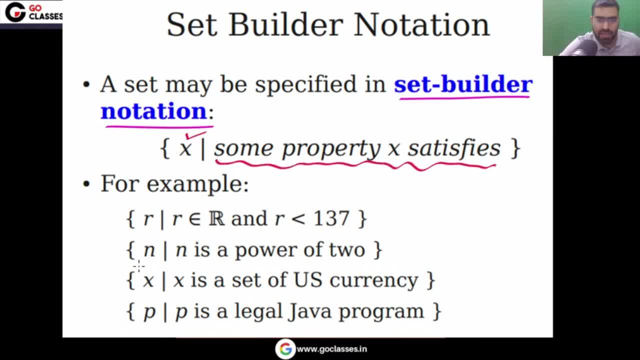 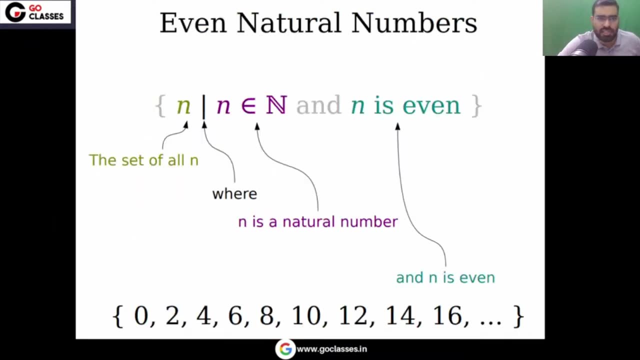 will satisfy this property, some property they must satisfy, satisfy. so all those elements we have in this set who will satisfy this property, some property, we will write here. okay, all those elements who satisfy this property are in this set, are in this set. okay, so this is your set builder notation, as you can see in this example. 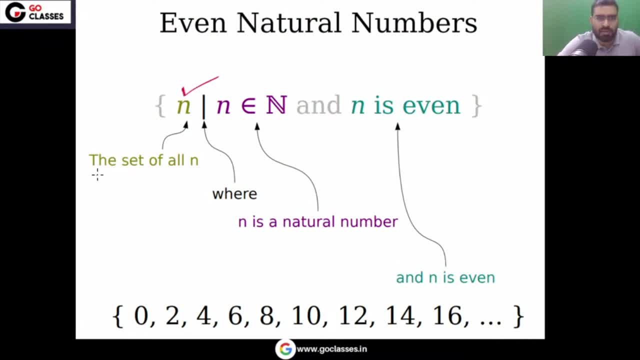 we have all those n, the set of all n, remember the set of all n, such that this property is satisfied, such that, such that, where such that n is a natural number and n is even, n is a natural number and n is even so, you can see, your set will be zero two. 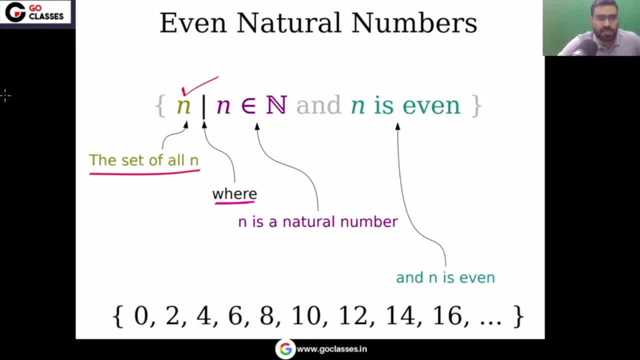 four, six. now you might be thinking, sir, zero is not a natural number. let me tell you that some people- they think they assume some authors, some mathematician, they assume that zero is natural number, some mathematicians- there are some mathematicians who don't take zero as a natural. 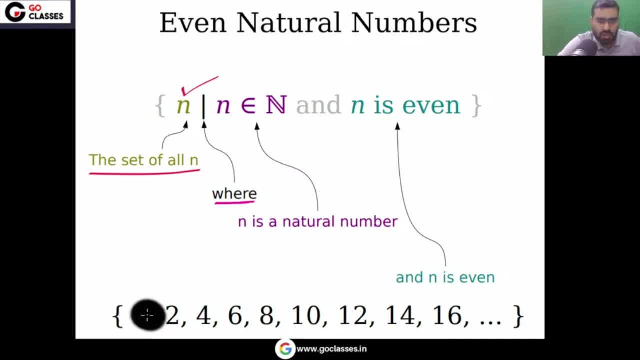 number. so it is your choice. okay, if you don't include this, no problem in the gate exam. you don't have to worry about it in the gate exam. be given if your answer depends on it. if your answer will change because of this zero, whether you take zero in the natural number or you don't take zero in the natural number, if your answer 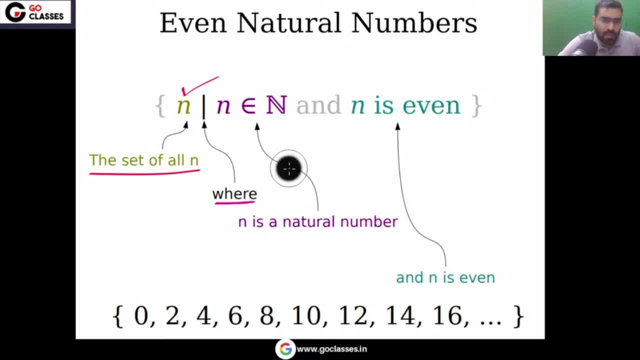 depends on that, then it will be given in the question. so do not worry about it, okay, if you are conf, if you don't want this zero in the natural number, then you can remove it, no problem, okay, but remember, don't worry about it, okay. some mathematicians: they consider zero as a natural. 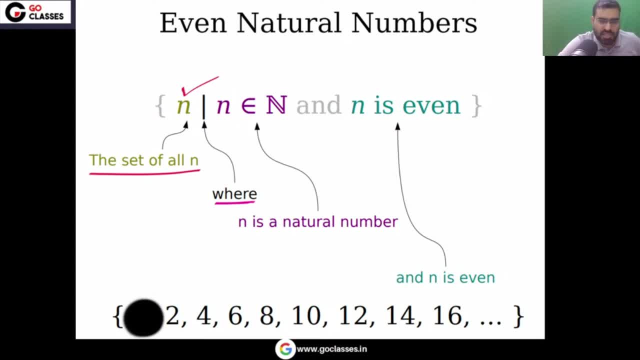 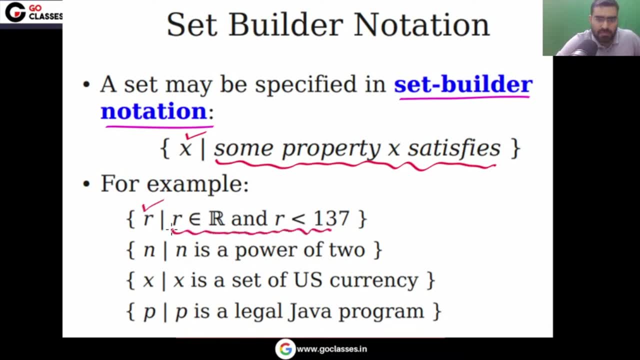 number, many mathematicians. they don't consider zero as a natural number. now let's see. so this is your set builder notation that all those elements who will satisfy this property. okay, so this is the infinite set, because you are saying that all those elements who are real number and 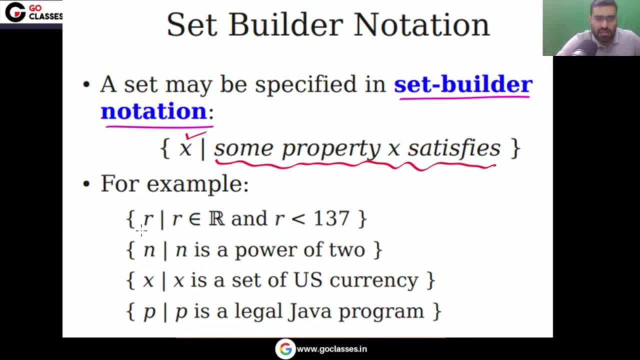 who are less than 137. so, of course, this is a, this is infinite set. all the real numbers which are less than 137. here you have, uh, basically, n is a power of two, all the numbers which are power of two. okay, this is a. this is a set which contains all the us currency and this is set which contains 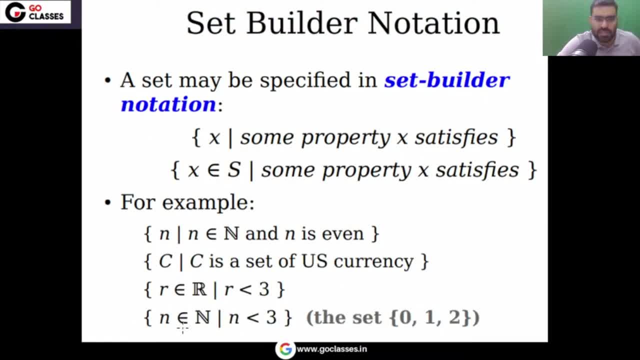 all the legal java program, so and so on. so very simple. you can check. for example, look at this set. this set says that those elements who are in natural number and who is less than three. so you can notice, if you don't want zero in the natural number, you can remove it, no problem. 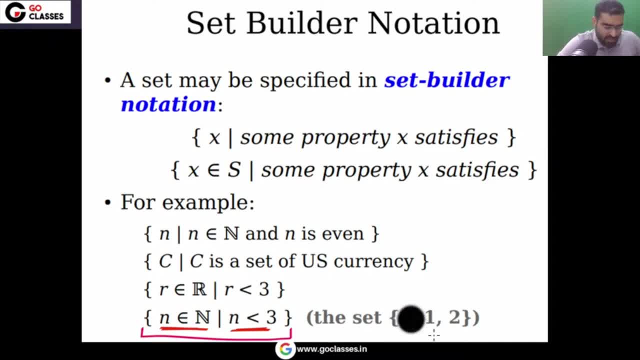 okay, you can, if you want zero. if you think that zero belongs to the natural number, then you can take it. if you don't think that zero does not, if you think zero does not belong to a natural number, then you can remove it. it does not matter. 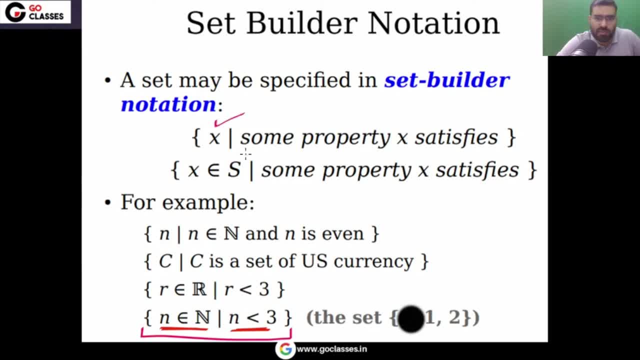 okay, so this is another notation, as you, as you can notice, those elements who will satisfy this property, or i can say those elements who belong to some set and their pro part- oh, and this pro, they satisfy this property. as you can notice, those elements which belong to set of natural number. 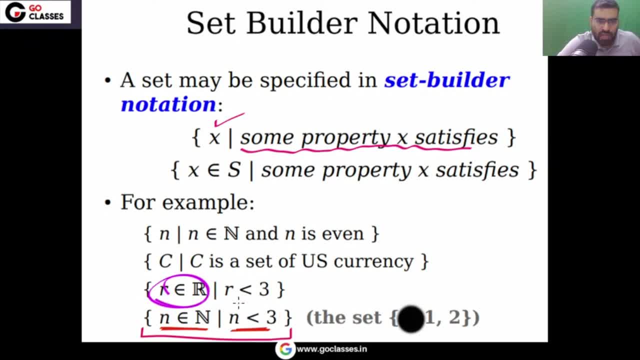 who are less than three, okay, those numbers who belong to set of real number who are less than three. so basically, in this set you have all the real number which are less than three. okay, in this set what you have, you have all the real number, all the real. 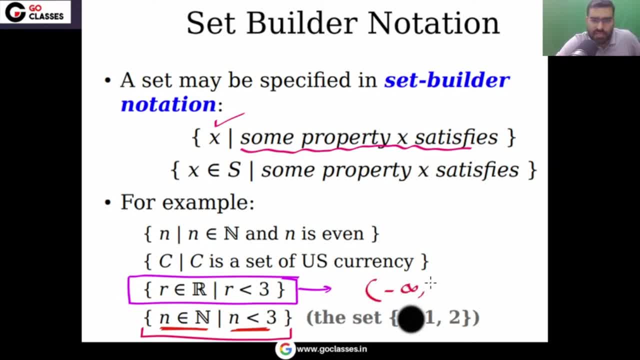 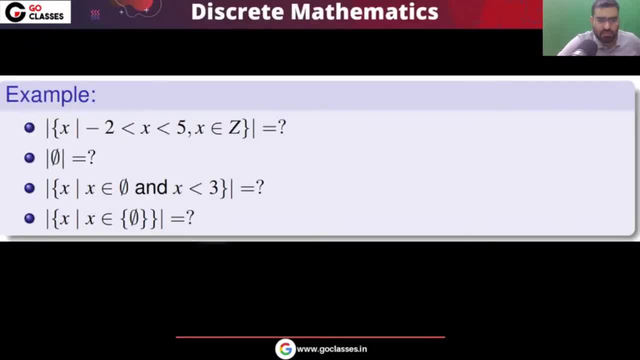 number which are less than three, so all the real number which are less than three. so this is your set. now let's move on. let's see this. tell me the answer for this question quickly, very quickly. tell me the answer. what is the cardinality of empty set in the empty set? empty set means there is. 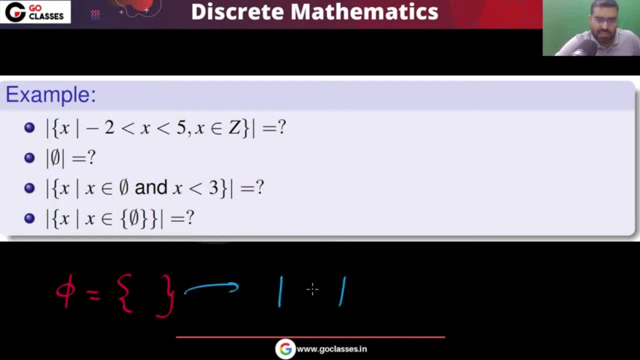 no element. what is the cardinality of this empty set? for this empty set, what is the cardinality? elements are there in this set, in this that there is no element, so the cardinality will be 0, so the cardinality of empty set that will be 0. okay, now the next. next, you can notice what is the. 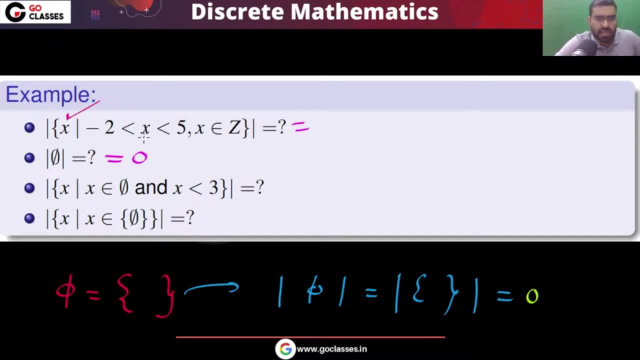 cardinality of this set. this set is saying that those elements greater than minus 2 less than 5. so what is this set? this set is basically asking cardinality of this set. okay, the set is basically like i can say minus 1, 0, 1, 2, 3, 4. so how many elements are there in the set? total? 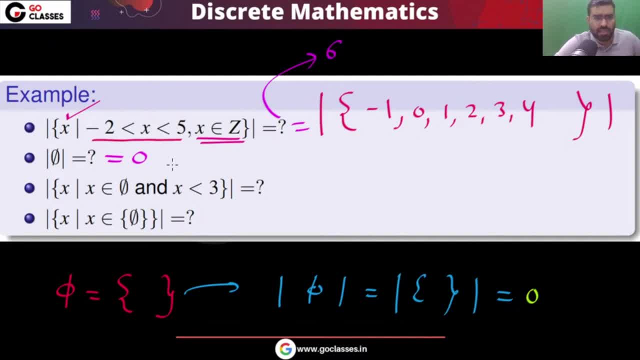 6 elements, so the answer here will be 6.. next, what is the answer for this question? the question is saying that: what is the cardinality of this set? what is the cardinality of this set? a set is given to you. what is the cardinality of this set? this is saying that x. 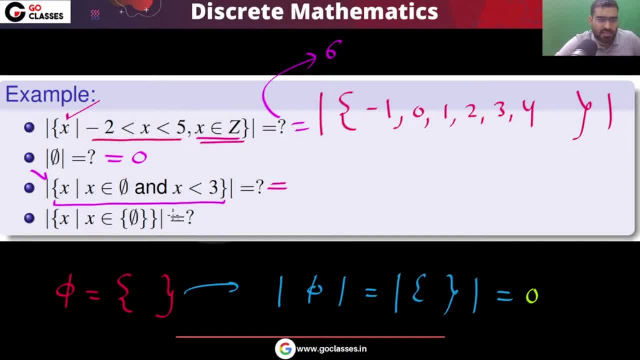 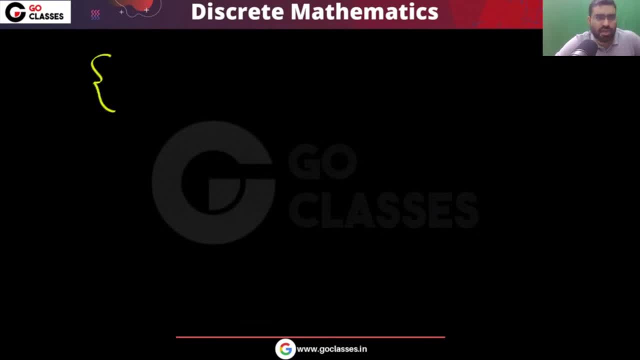 belongs to phi, but there is no x in the phi, right, see, there is no element. who will say that he qu chords and there is a set here, with a set, each one of them has a certain cardinality and satisfy this property, correct? do you agree? like if i say, if i say that x belongs to, there is no. 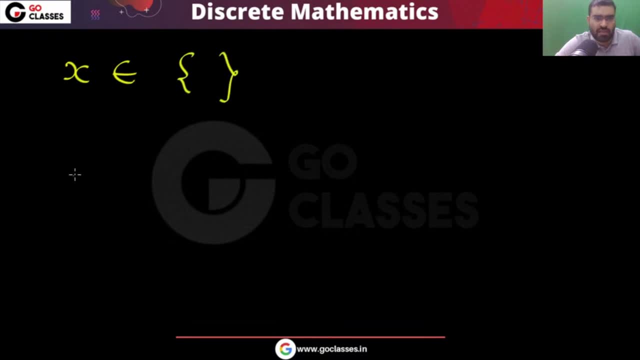 such x. if i say x belongs to phi, then it simply means there is no such x, right? okay, no, no such x. so if i say that let's assume there is a set, there is a set in which you have those elements who belong to phi- okay, those elements who belong to phi, then that is your phi itself, remember? 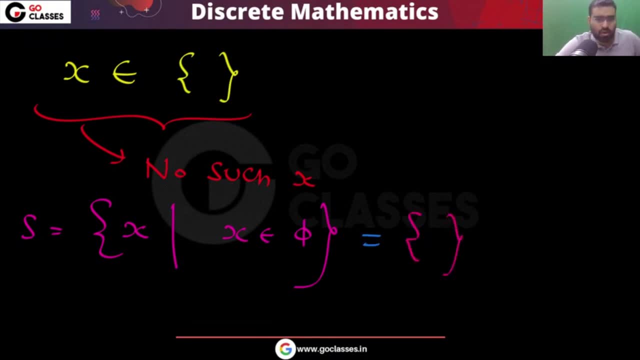 that is empty set. those elements belong to phi. that is empty set because there is no element which belongs to phi, no such x. so if i say that those i want, those elements who will satisfy this property, okay, those elements who will satisfy this property, then there is no such element. so 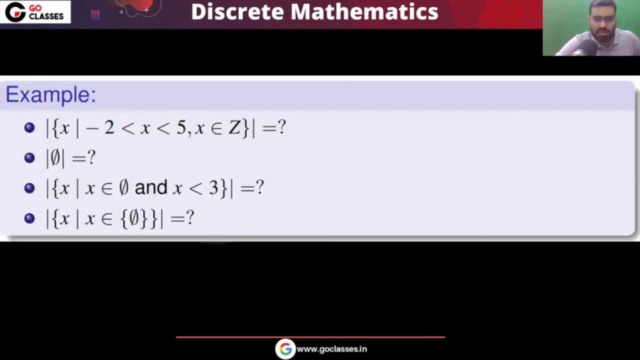 s will be empty set. okay, now here you can notice that this is your cardinality of empty set. so here also i can say the cardinality of, i can can say the cardinality of empty set, and that will be zero. what is the last question? the last question? 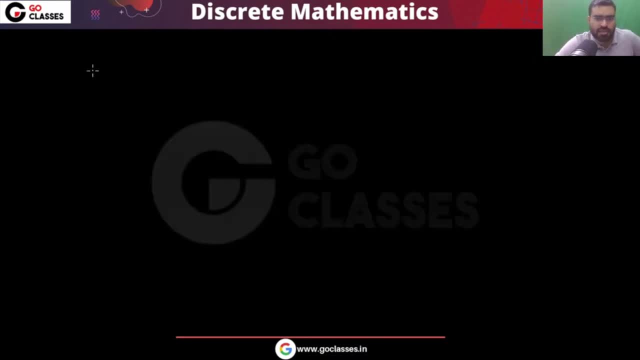 is saying that x belongs to this set. look at this: if i say that x belongs to this set, remember this is not empty set. please understand that. this is not empty set, right? this set is not empty set. in this set, you have one element, so it simply means that from here, you can easily see that x. 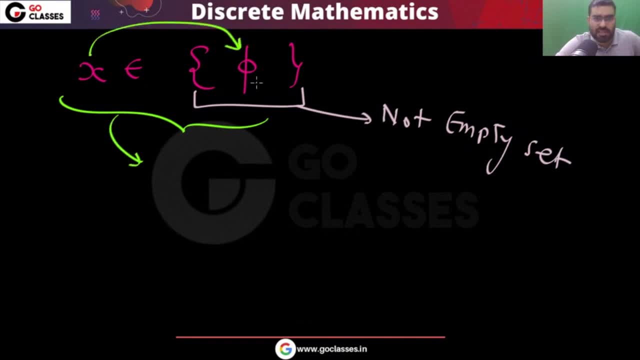 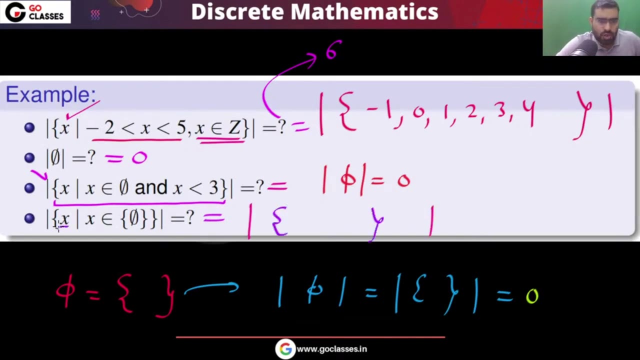 is empty set because it is. it simply means x is empty set, x belongs to this set. so i can say here i can say x is phi. okay, so very simple. you can notice that what this set? the cardinality. the question is asking for cardinality of this set. in which of that element which belongs to this set? 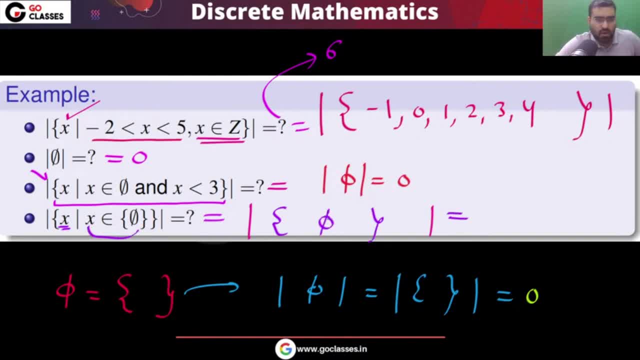 okay, so it simply means that x is phi. now for this set. remember, for this set the cardinality is one. so for this question answer will be one. i hope all you answers are correct. so the answer will be six zero zero one. this is going to be the answer, okay. 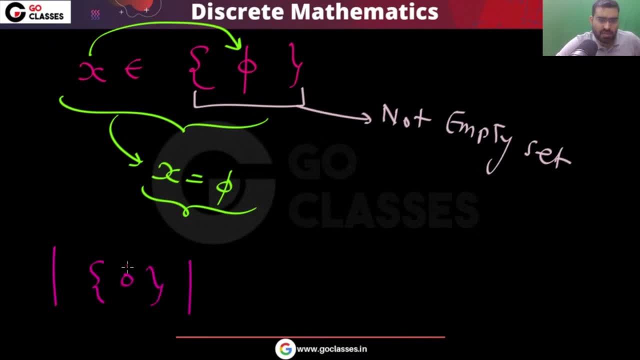 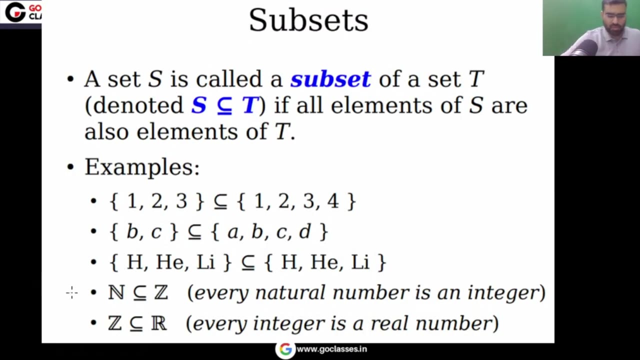 what is the cardinality of this set? the cardinality of this set will be one, because i am asking the cardinality of this set and in this set there is one element, so the answer will be one. now let's move on. now let's see the concept of subset. what is this concept? subset means sub collection. okay, 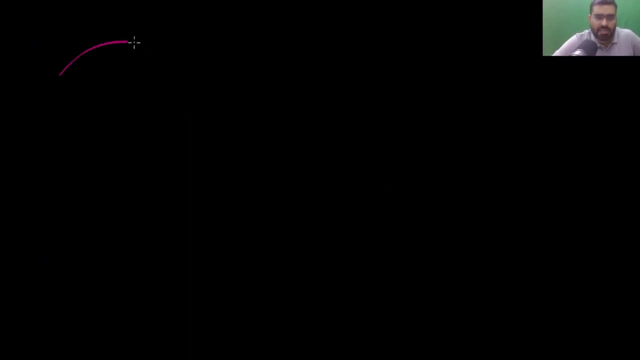 subset means sub collection. i can say that let's assume there is a collection. this is a subset of this collection. it simply means that every element that you have here, you can also find here. every element that you have, you can also find here. every element here, you can also find here. but, but, but. 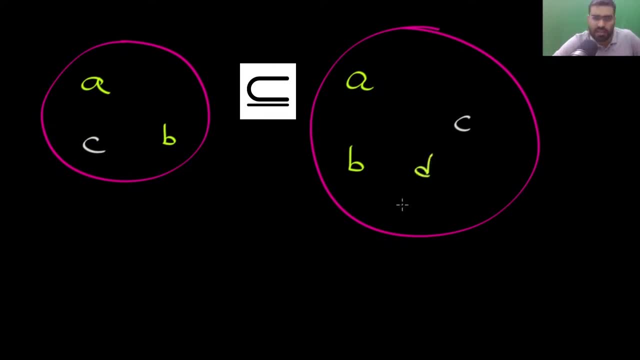 some extra elements can be here. for example, you can have d, e, f and so on. so i am saying that subset means subset means that every element that you have here that is also here. so i can say This: S is subset of T. It simply means that S is a subset of T. 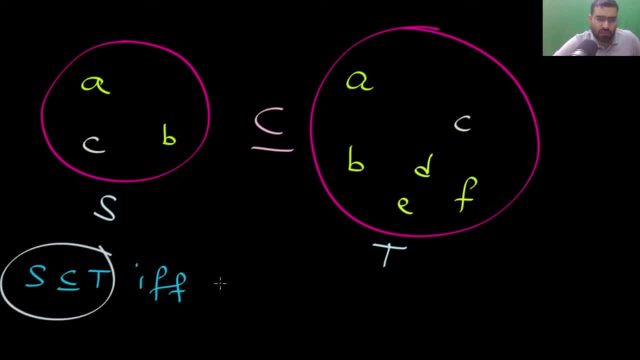 What this means: S is sub collection of T. What this means: This means that if anything belongs to S, then it also belongs to T, But T can have extra things In the T. you can have some extra things. But remember S is subset of, S is a sub collection. S is a subset of T. 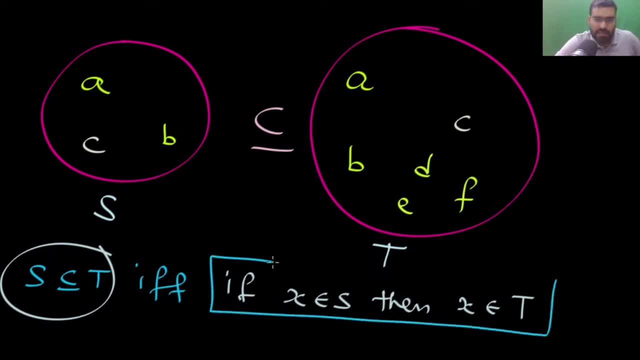 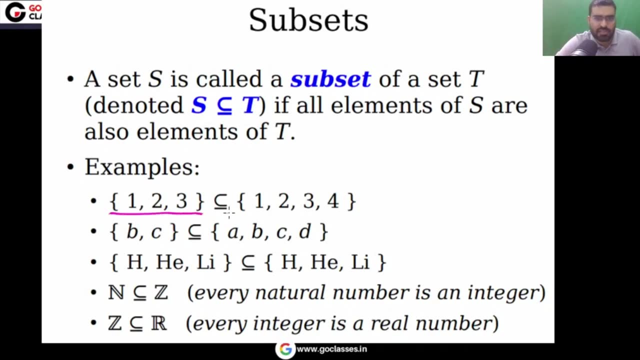 It simply means that if anything belongs to S, if any element belongs to S, then that also belongs to T. So, for example, you can notice This set is a subset of this set, Because every element is here also So easily you can see that this is a subset of this set. 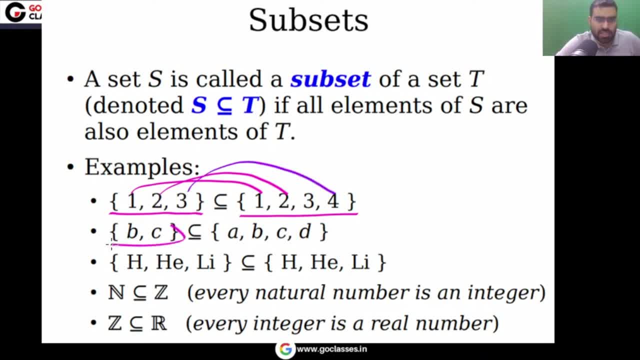 You can not. this is a subset of this set, Because in this set you have two elements. Those two are also an element of this set. You can not. this is a subset of this set. Every set is subset of it self, OK. 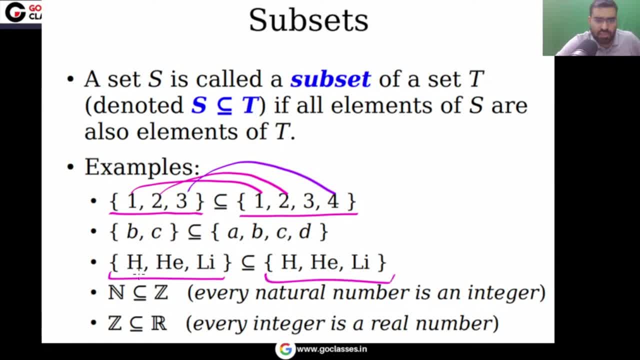 Of course, Because every set is subset of itself, because every element that you have here, that is also element here. so you can notice every set is subset of itself. you can notice set of natural number that is subset of set of integers, and set of integers is subset of set of real number. 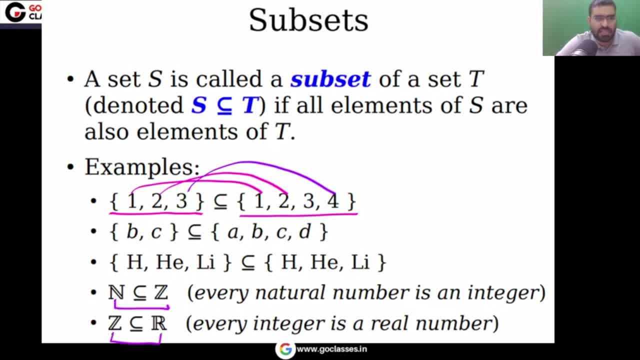 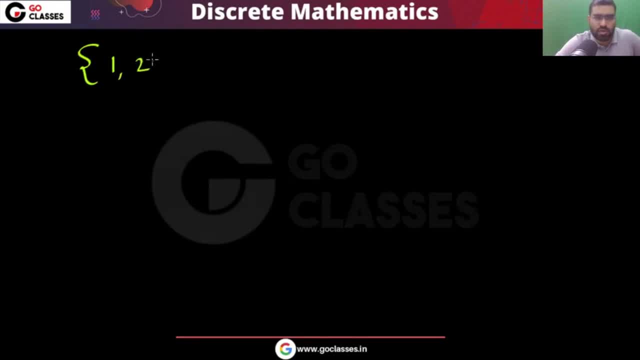 because every integer is real number, every natural number is integer. okay, let's move on. so very easily you can see what is a proper subset like. consider this set. you can see that this is also subset of one comma two. you can also see that one comma two, that is. 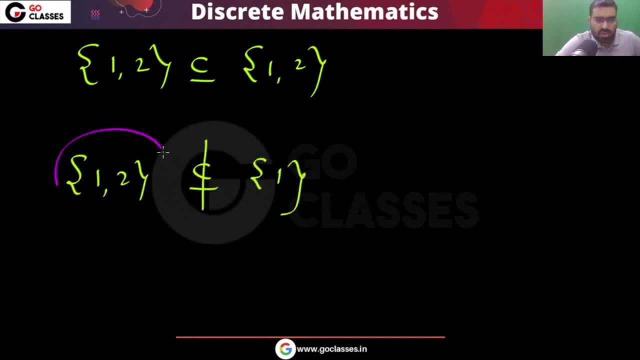 not a subset of one, because this is not a sub collection of this one. because you can easily see this: two is the counter example and what is the counter example? the counter example is two, the counter example, the counter example will be x equal to two, because you 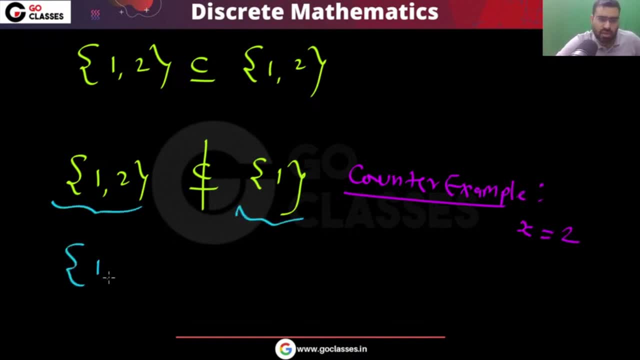 can notice x belongs to this, two belongs to here, but it does not belong to here. you can notice this: one comma two. this is not a subset of 1 comma 3. okay, again, you can notice this counter example. the same counter example will work. so here also the counter example will be x equal to 2. okay, so very simple. now i want to tell. 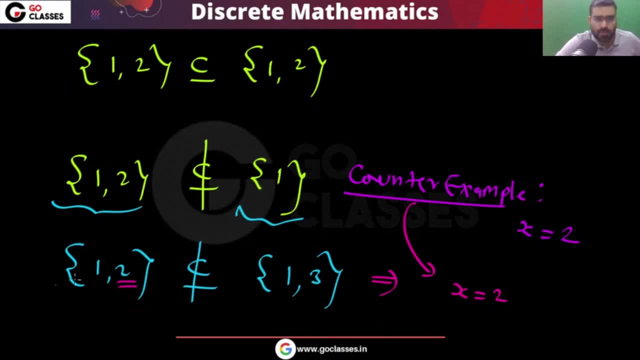 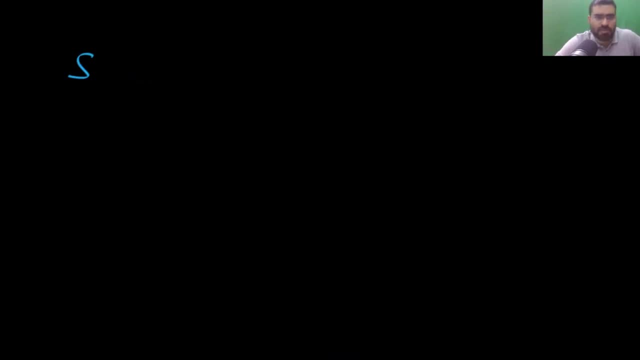 you that this type of set is. this is not a proper subset. proper subset means: proper subset means that i can say s is a proper subset. when can you say s is a proper subset of t? this means proper subset if, and only if, s must be subset of t and s must not be equal to t. okay means basically: 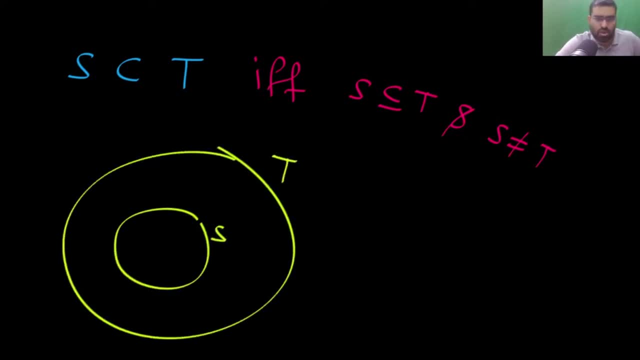 proper subset. proper subset means: this is your s, this is your t, every element in s, that is also element in t. but there must be some extra element. okay, there must be some, something extra, some extra, some, some extra element in t. so in this situation you will say that s is subset of s is proper. 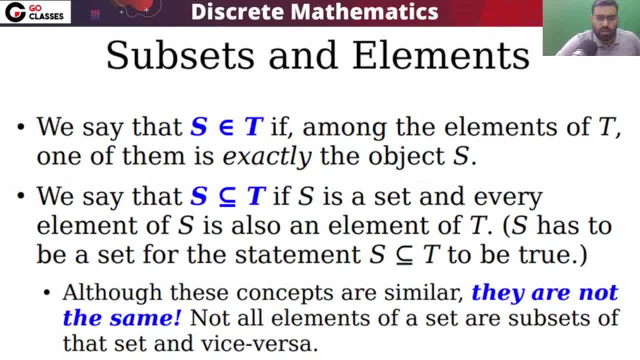 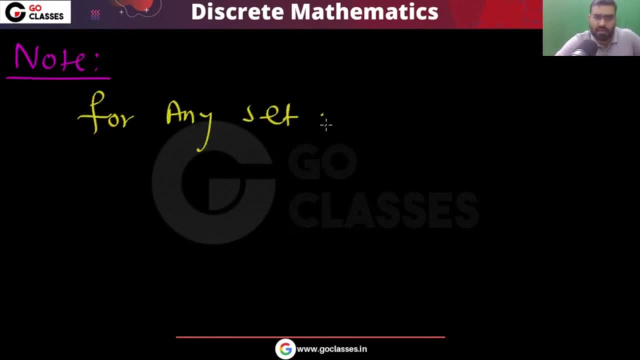 what are those for any set, whatever you. what are those for any set, whatever you, whatever set you take for any set, whatever set you take for any set, whatever set you take for any set, for any set s these two things will happen for any set s these two things will happen. 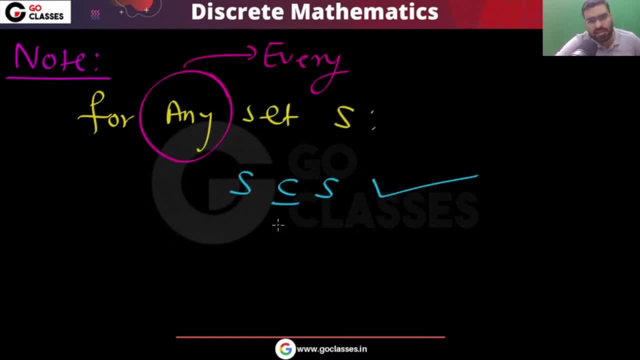 for any set s, these two things will happen. what are those you can take whatever? what are those you can take whatever? what are those you can take whatever? whatever set you take, that is subset of whatever set you take. that is subset of whatever set you take. that is subset of itself. 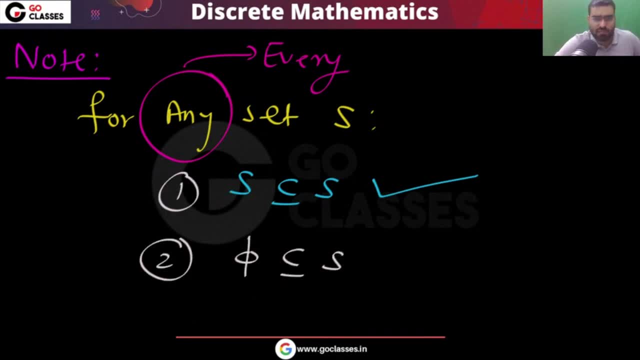 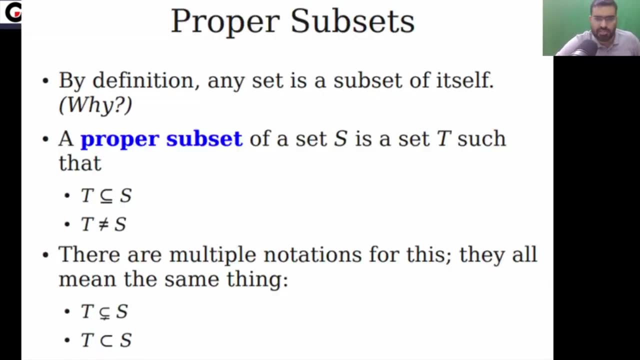 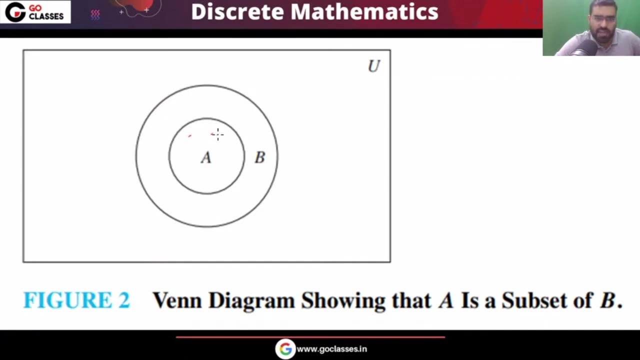 itself itself. and whatever set you take empty set is, and whatever set you take empty set is, and whatever set you take empty set is subset of itself. okay, Now let's move on. So we have seen the definition of this is the Venn diagram. You can notice every element of A is also element of B. 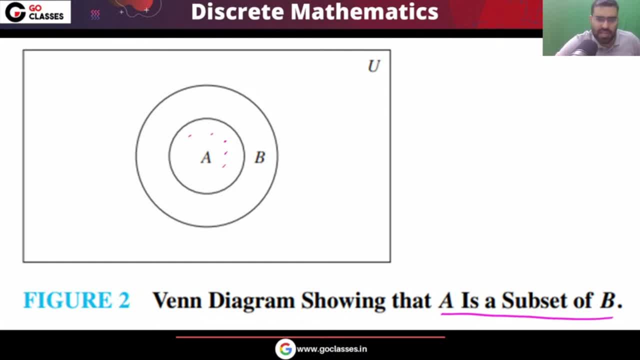 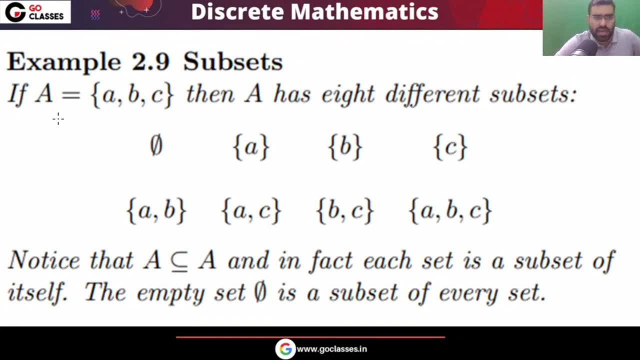 This is the Venn diagram of that. A subset of B means every element of A is also element of B. like you can notice that, for this set, how many subset you can create for any set, how many subset I can create in this set you have three elements. how many subsets you can. 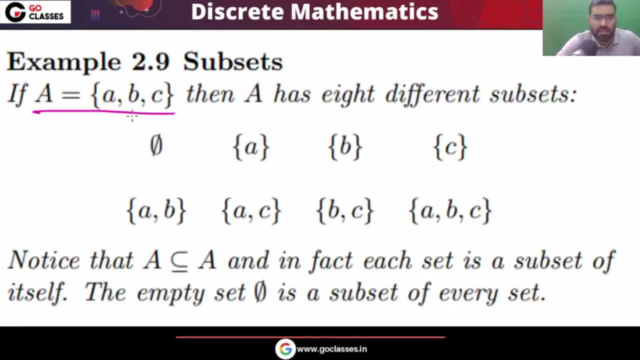 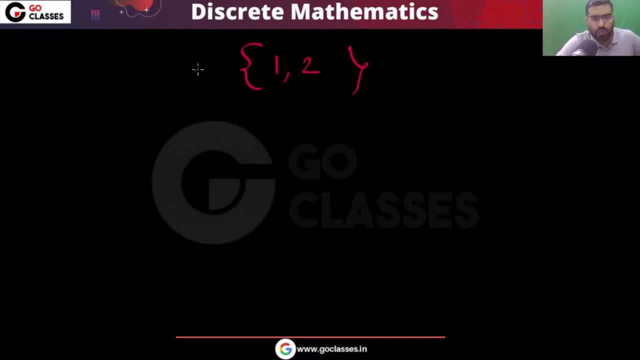 create. So how can we create the subsets? you can notice that if you want to create a sub collection, very easy. if I give you some collection, let us assume I give you 1 comma 2 if you want to create subsets of this. if you want to create subsets of this as sub collections, you want. 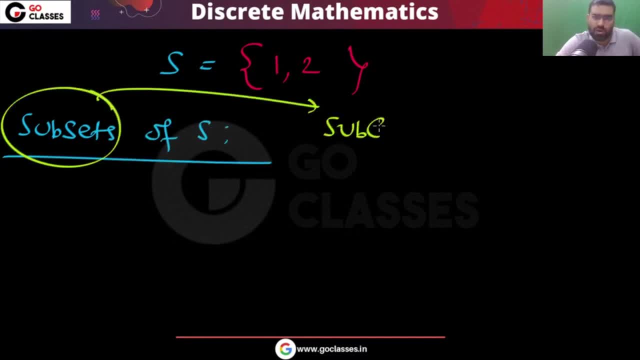 to create subset means sub collection, OK, so if you want to create sub collections, then what you can do, you can delete 0 or more elements, so sub collections, you can do what you can do, you can delete both the elements. just remove both the elements. you will get a sub collection that is empty set. 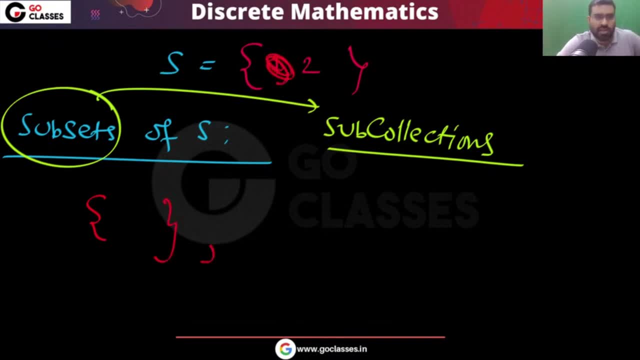 OK, So this sub collection you will get if you delete this element. you will get another sub collection that will be this sub collection. You can notice that every element in this collection is also element in this collection. So I can say this is a subset of this set. 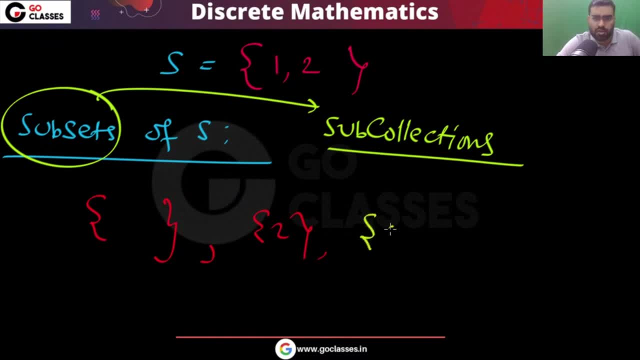 Next, you can delete this one. then you will get another subset, So you can delete these two. you will get another subset. that will be that will be one. You can notice that every element in this set that is one that is also element in this set. 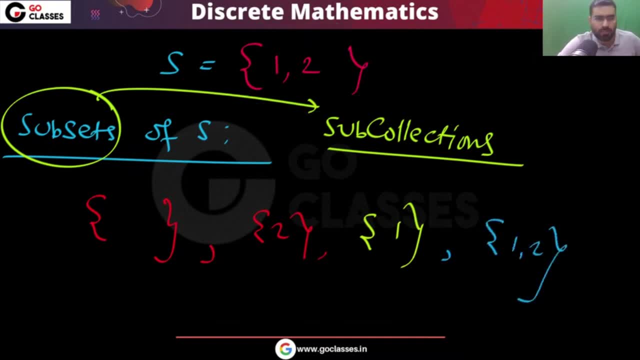 you can notice, you can keep both of them. Okay, you can keep both of them. you can notice that every element here you have two elements here: 1 comma 2- every element here is also element here. So this is another subset. So total how many subsets? you have four subsets. 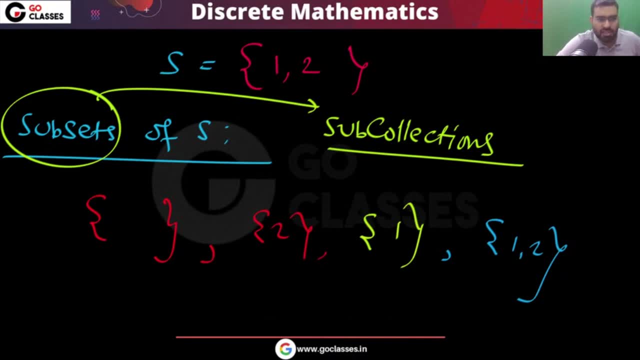 Okay, now let me tell you that if you make a set of all these subsets, if you make a set of all these subsets means all these subsets, if you put in a set all these, if you put in a set, that will be called power set. Okay, that will be called power set. 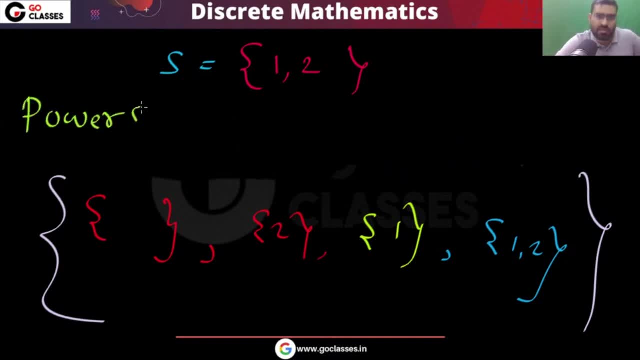 So this is the definition of power set. power set means This will be called power set of S. You can denote this by P of S, power set of S, or you can denote this by 2 power S. These are the notations. Okay, so you can denote as P of S power set. 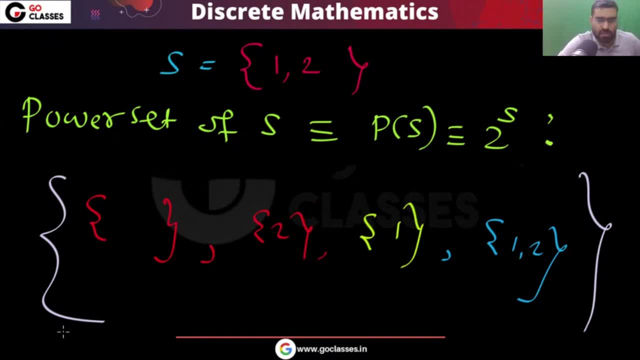 It simply means that set of all the subsets of S. Okay, you can notice, this is a set. This is a set which has all the subsets, All the subsets of S. So, collection of all the subsets of S, that is your power set. 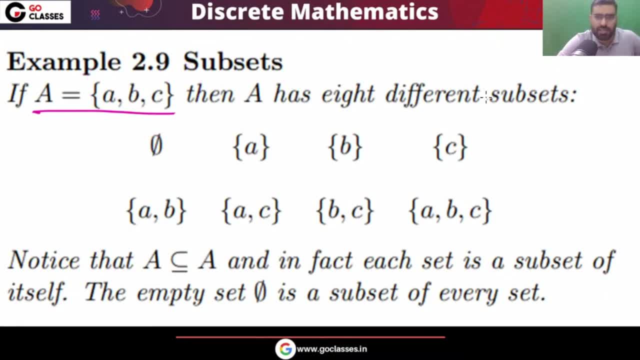 So you can easily see if your set has three elements, then you can create total eight different subset. you can create: Okay, this empty set is subset of every set. Every set is subset of itself and you can notice, every element of this set is also element. 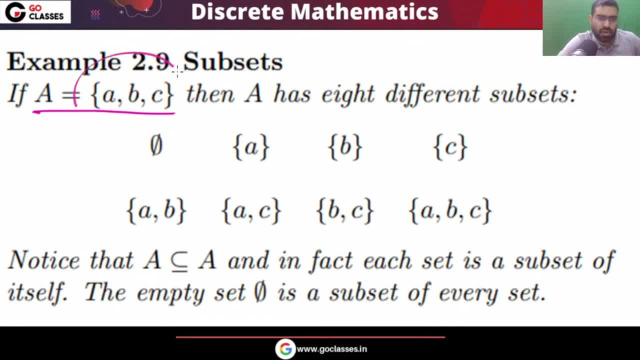 of this set. As I told you, if you want to create subset, then you can delete zero or more elements from this set. So from this A, I can delete zero or more number of elements I can delete To create subset. if I delete this B, then I will get this subset. 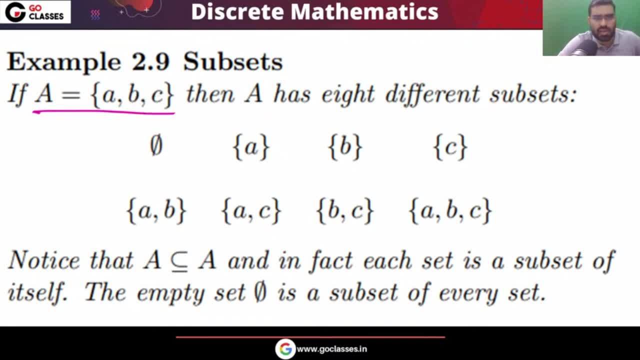 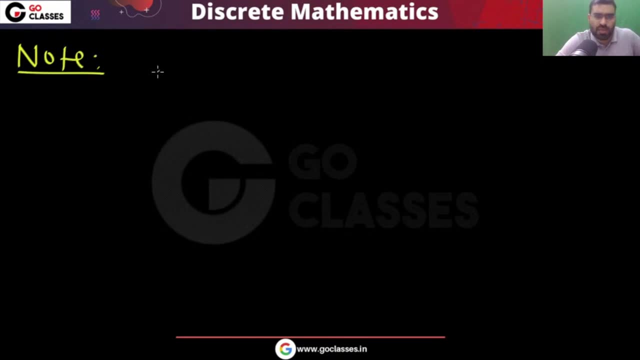 If I delete this B comma C, then I will get this subset. So total eight subset I will get. You can notice every set is subset of itself and empty set is subset of every set. Now, how many subset you can create? Simple question. I am asking a very important note that if you have a set, let's assume if 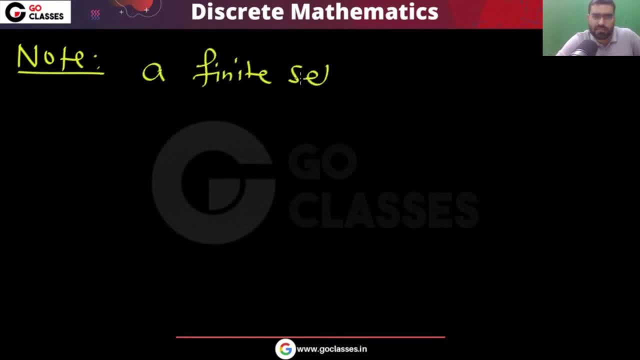 you have a, if you have a finite set, If you have a finite set S of n elements In which you have total n elements of n elements. So if you have total n elements in the set, then how many subsets you can create? What is the number of subsets? 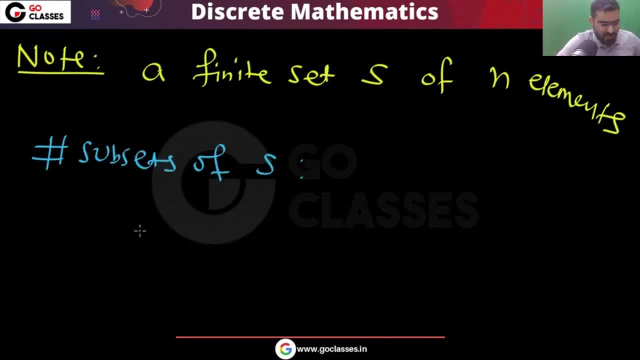 What is the number of subsets of S? So how many subsets can we create? tell me, In you have a finite set of set, S set of n elements. there are n elements in this set. then how many subsets you can create? That will be two power n, two power n subsets you can create. 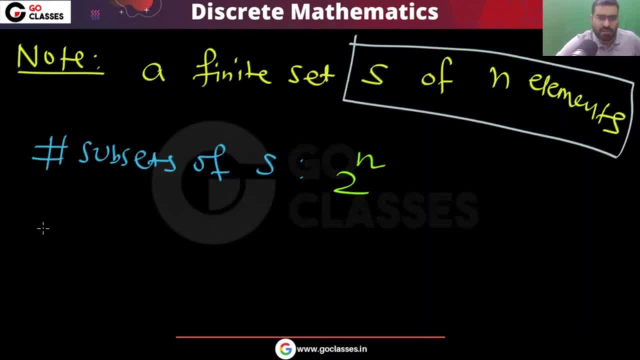 Okay, Very easy. Every element. you have two choices, right? See? very easy that if I give you a set S, let's assume I give you some set S. then when you are creating the subset, like let me give you A, B, C now from this set, when you create a. 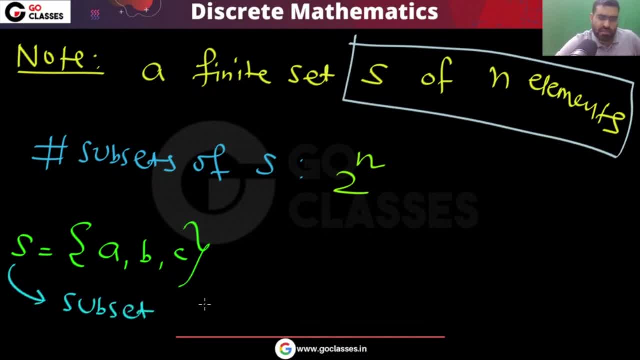 subset, a subset you are creating- let's assume you are creating a subset S one- then you can notice that when you create this subset, then every element has two choices. Okay, when you are creating this subset, then it simply means that every element has two choices. 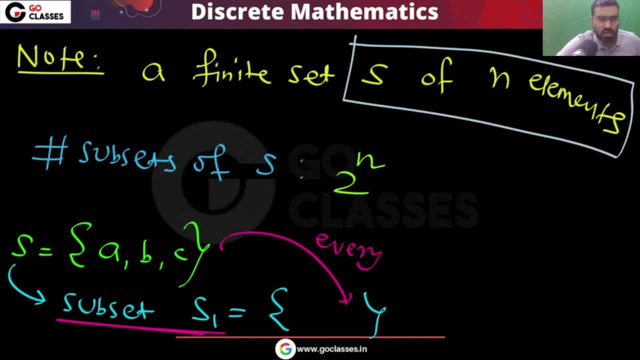 Every element of S has two choices: either it will go to the subset or it will not go to the subset. Okay, so every element of S, every element of S, has two choices. Okay, you have two choices. every element has two choices. for example, this A has two choices. 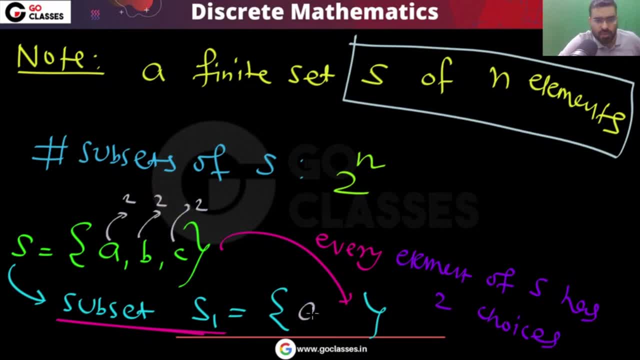 this B has two choices. this C has two choices. either you can put it or you don't put it. Okay, This B has two choices: Either you put it in the subset or you don't put it in the subset. Okay, subset. So every element has two choices. So you can notice number of subset will be. 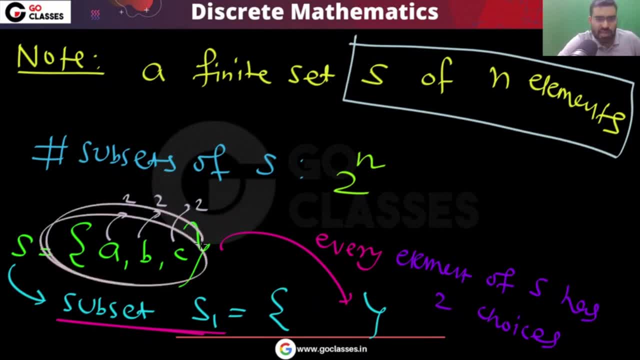 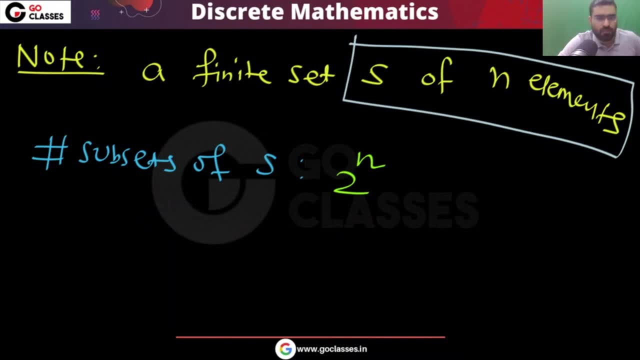 two into two into two. That is, two power three. If you have three elements, then number of subset will be eight And if you have any limits, then number of subset will be two power n. What is the number of proper subsets? What is the number of proper subsets That? 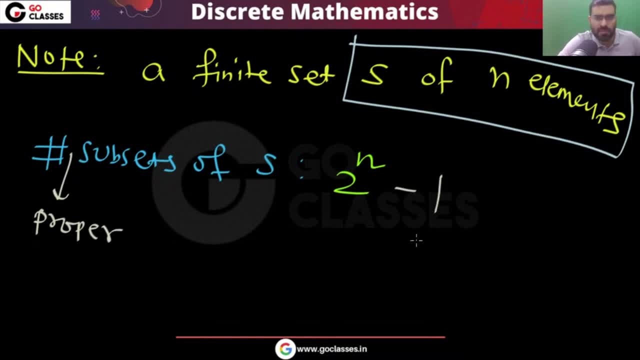 will be two power and minus one. Okay, It will be two power and minus one. This one you are removing for as itself. Okay, For as itself, you are removing this one. Remember one thing: You tell me a simple question. I am asking if I give you a set, for example, 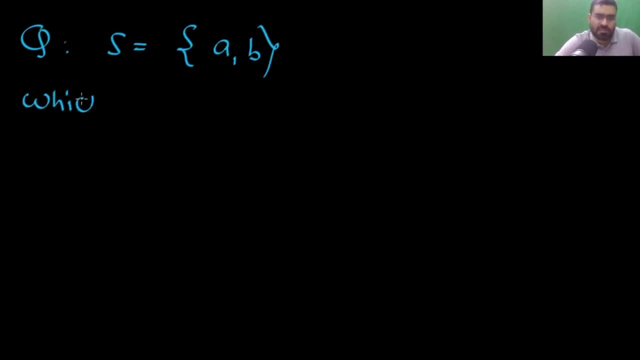 a, comma b, this is a set. Then tell me which is a proper subset, Which is a proper subset? A simple question I am asking: Which is a proper subset? First option: Is this a proper subset? Another option: Is this a proper subset? Another option: Is this a proper subset? 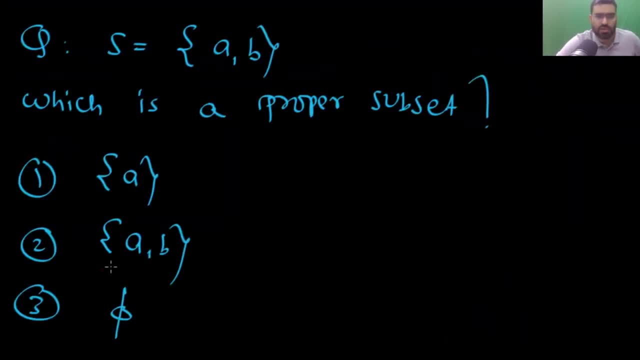 Which is a proper subset? You tell me the answer: Which is a proper subset? Proper subset of s, of course, Okay, I am asking which is a proper subset of s, So the answer will be: this is a proper subset, because this is another option I can give you. I can give. 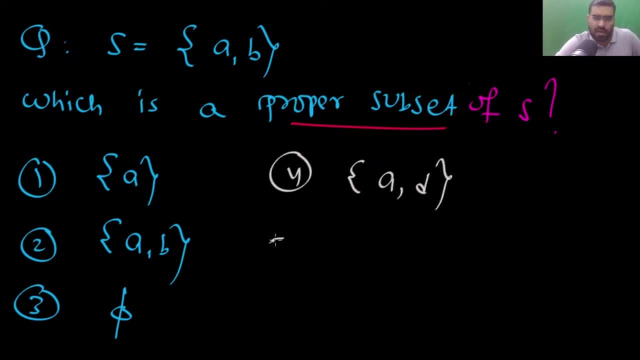 you this option, a, comma d, Another option I can give you that I can give you as e. So these are the options I am giving you. You tell me So you cannot. this is a proper subset. It is a subset and it is not same as s. 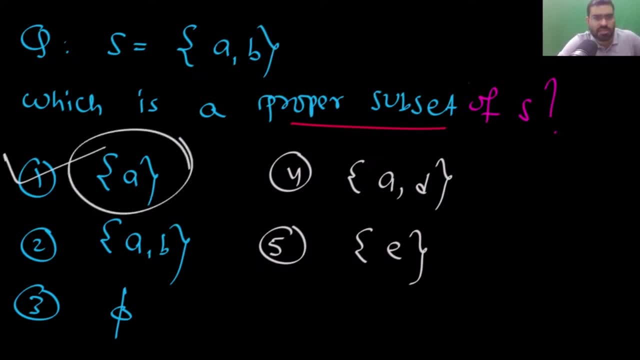 This set and this set. they are different and you cannot. this is a subset, So this is not a proper subset. This is a proper subset. This is not even a subset. This is not even a subset. So remember: this is a proper subset. This phi is a proper subset, Very simple. 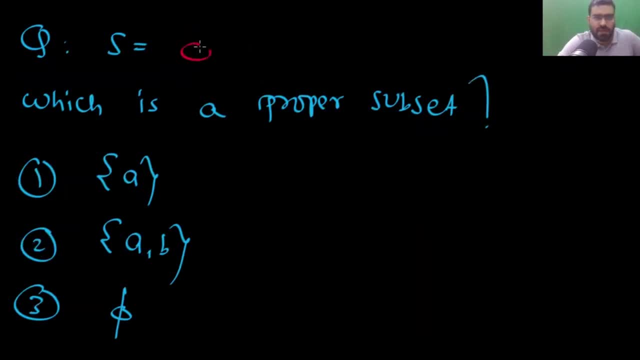 Now let me ask you if your set itself is phi, If your set itself is phi, then what is proper subset of s? What are the proper subsets of s? So tell me. And the fourth option is none. The fourth option is none, So tell me the answer now. 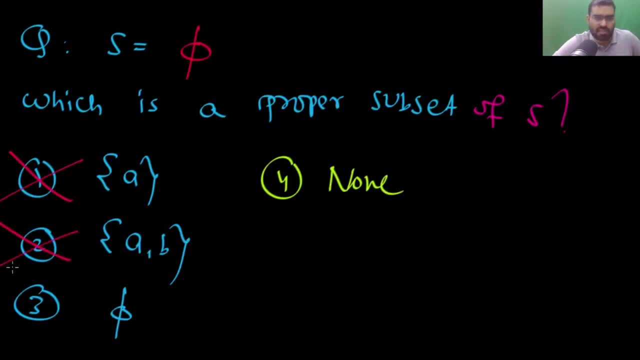 So easily you can notice. this is not even a subset. This is not even a subset. This is a subset, but this is not a proper subset. Okay, So this is not a proper subset. So there is no proper subset of phi. Okay, Because phi does not have any proper subset. Remember. 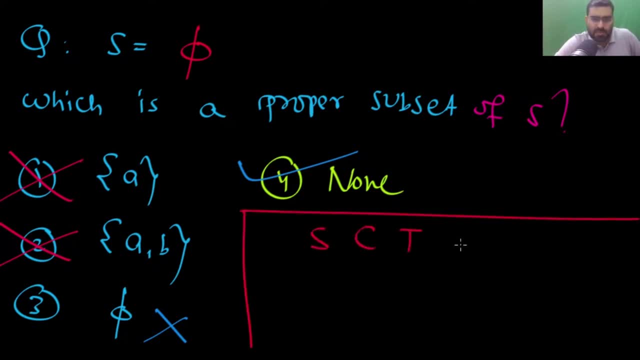 the definition. I can say: s is a proper subset of t if, and only if, s is not equal to t and s is a subset of t. Okay, s is subset of t and s is not equal to t. So remember this: phi is not a proper subset of phi. Very simple, You can see this. Now let's move on. So what? 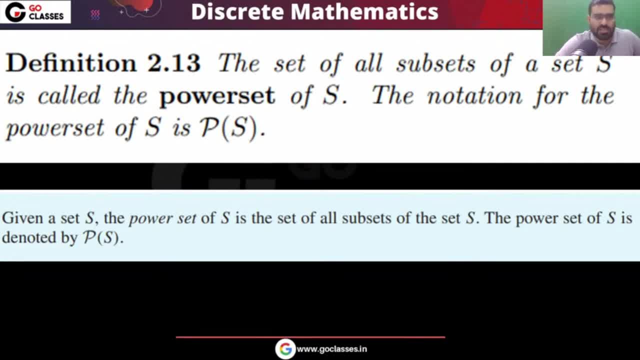 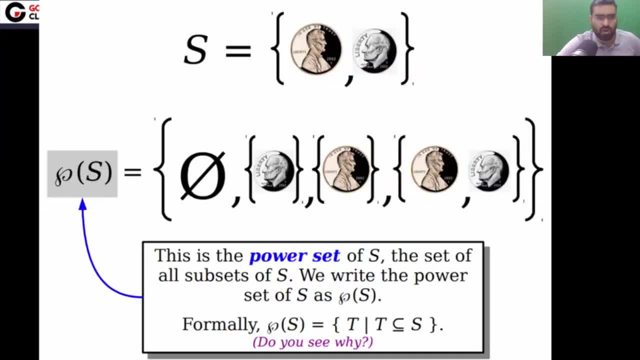 is a power set. Power set means set of all subsets of s. Okay, That is power set of s. That means set of all subsets of a set s. That is called power set. Now let's move on Like this set. you can notice, In this set you have two elements. The power set will. 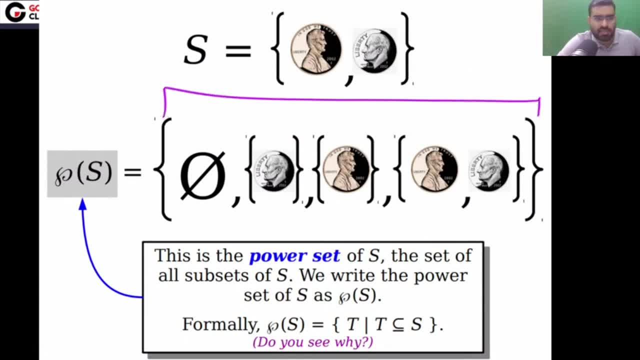 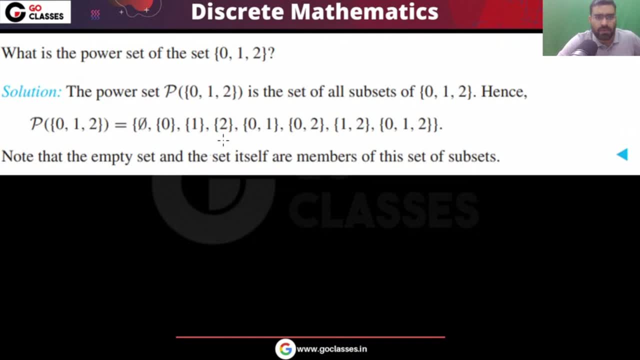 have four elements. Okay, Power set. In this you have all the subsets of s. These are all the subsets of s. Very simple. Now let's move on. You can see for this set, the power set will contain the set of all the subsets. So the power set will contain total eight elements. Can you tell? 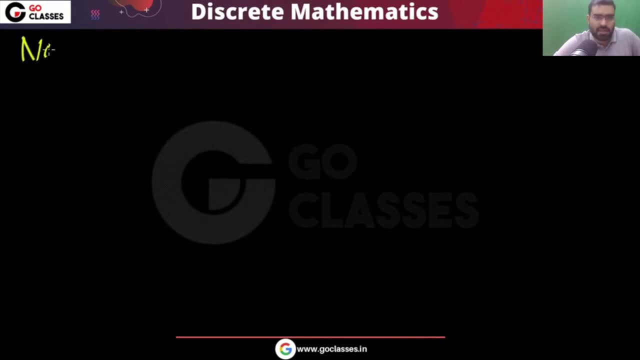 me what is the cardinality of power set? Another note, Another important note: that if you have a set s of n elements, If you have set s of n elements, Then tell me what is the cardinality of power set of s, What is the cardinality of this? 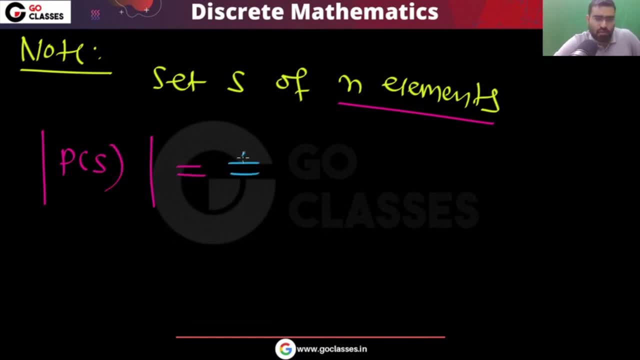 power set of s, That will be same as number of subsets, Because in the power set every element is a subset. So that will be same as number of subsets of s And that is same as two power, and that we have already seen. So in the power set every element is a Every. 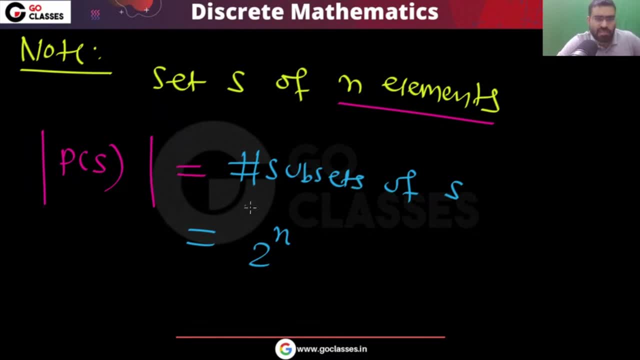 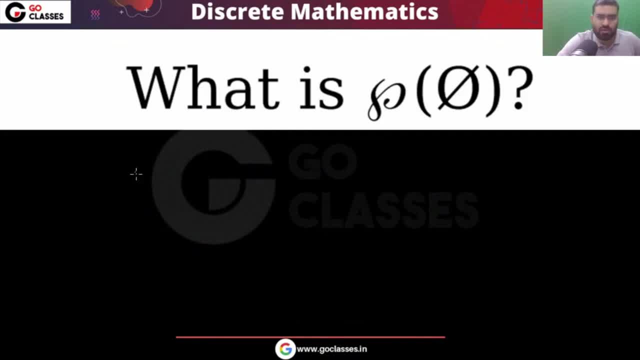 be two power, and very easy. now let's move on. tell me what is the answer for this. what is the power set of phi? so remember, phi is empty set. so how many subsets are there? first of all, you find out all the subsets, all the subsets of this phi. how many subsets are there? the only subset is phi. 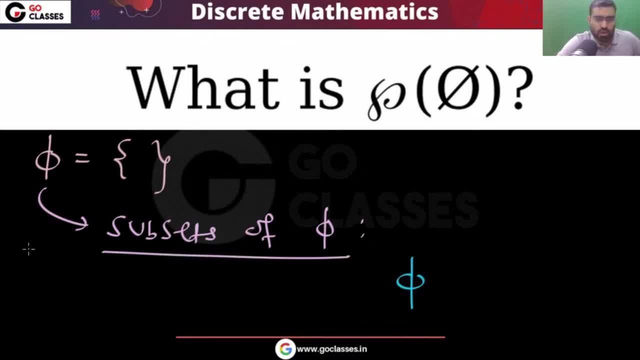 for phi. the only subset is phi. so now you can find out the power set. now you can find out the power set of phi. the power set of phi will be the collection of all the subsets of phi. this is a subset of phi. the collection of all the subset of phi. this will be the power set of phi. 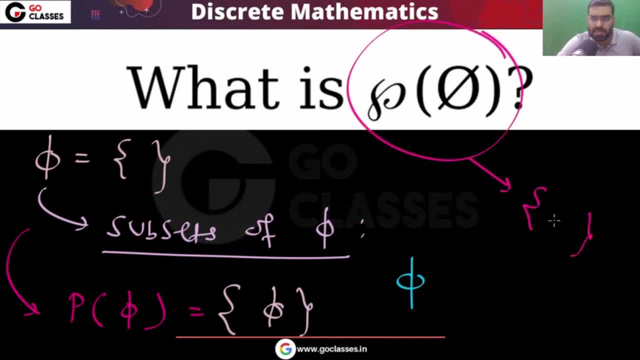 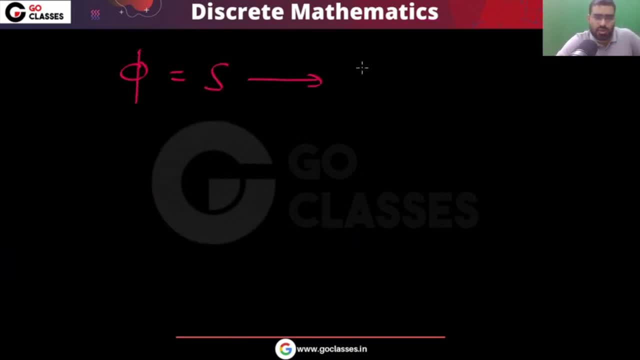 so remember, for this question the answer will be set containing phi. okay, and you can easily see. you can easily see that this phi, let's call it as so the cardinality, is basically zero. so the cardinality of power set of phi, the cardinality of power set of phi, that 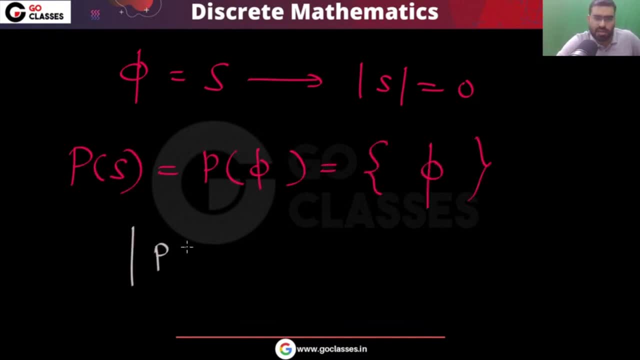 is basically one and that should be one. okay, the cardinality of power set of s, that is, two power, the cardinality of s. so you can notice here, the cardinality of s is basically zero. two power: zero is one. so that is correct. okay, let's move on now. let's see this. 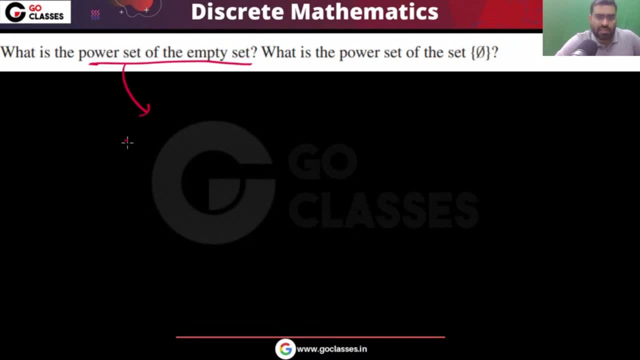 uh, so what is the power set of empty set that we have already seen? the power set of empty set will be set containing empty set. what is the power set of this? so here your set is not empty set. here your set has one element. so in the power set there will be two elements. 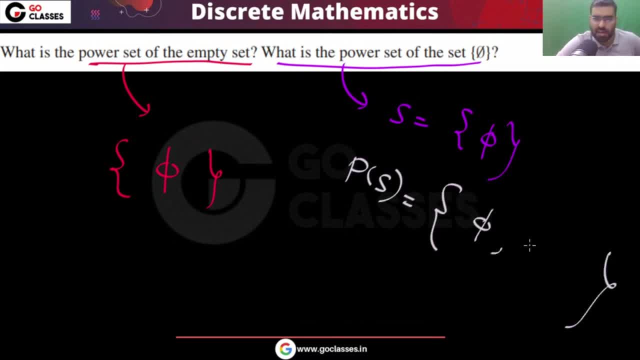 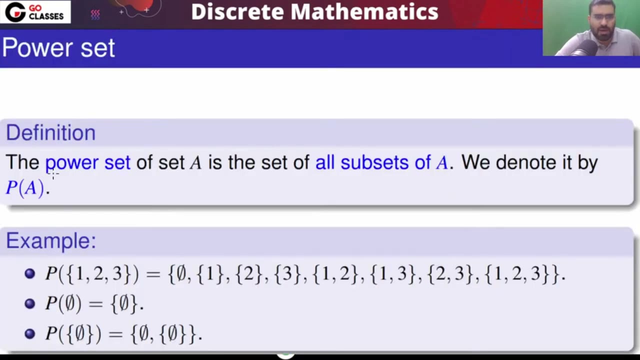 in the power set there will be two element. one will be empty set, another will be as itself. okay, so you can easily see here the cardinality will be two. okay, let's move on. so these questions you can do. uh, okay, so this is the definition. power set of a set is basically: 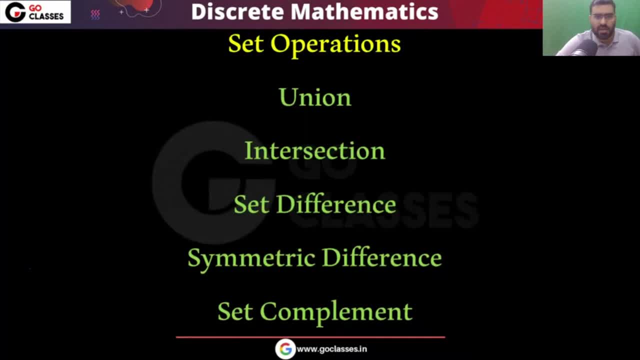 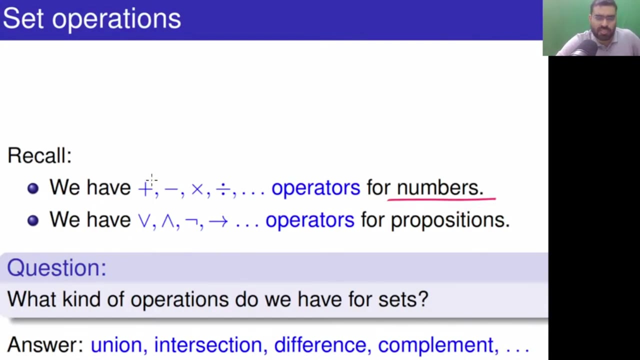 set of all subsets of a. so that is your power set. now let's see set operations. how many set operations are there? they? we have many set operations like union, intersection, uh, set difference, symmetric difference, set complement. see, you have operations on the numbers. so when you study the numbers, then you have some operations like addition, subtraction. 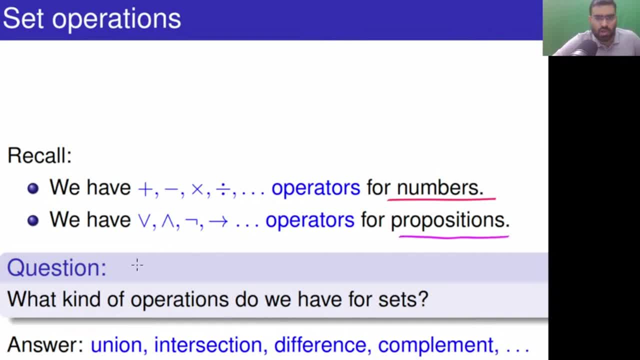 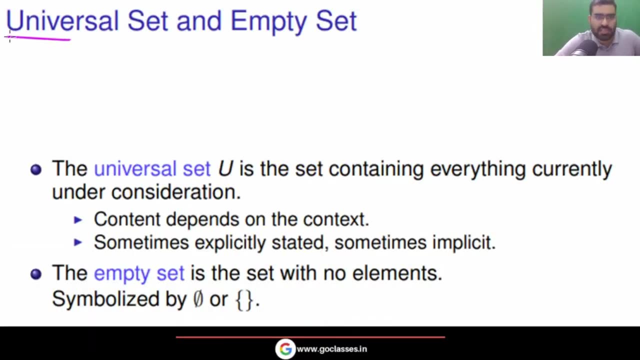 multiplication, division. when you study propositions, then you have some operations like conjunction, like disjunction, conjunction, uh, negation, implication, and so on. similarly, for the set also, you have some operations like union, intersection, difference, complement, and so on. let me tell you what is a universal set. universal set, the name itself is telling you: universal. universal set contains everything that. 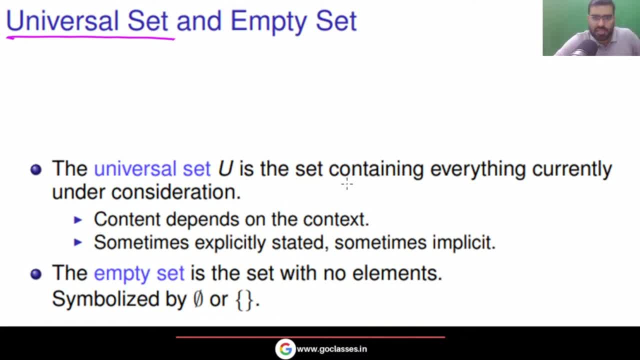 is under consideration. okay, remember, universal set contains every element that is under consideration, every element that you consider that is under consideration. that element belongs to universal set. of course, it will depend on the context. for example, if you study chemistry, then your universal set can be set of all the elements in the chemistry. now, similarly, if you study 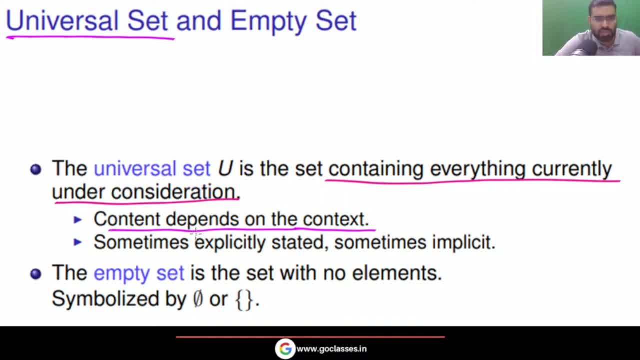 natural number, then universal set can be set of natural number. if you study real number, universal set can be set of real number. if you study complex number, then universal set can be set of all the complex number. so universal set contains everything. okay, this is important. universal set contains everything that you consider that is under consideration. 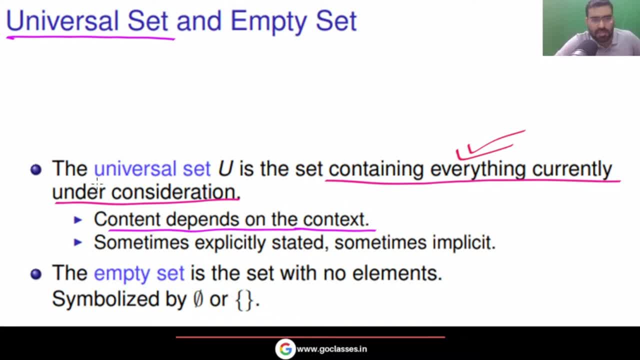 okay, sometimes it will be given, sometimes it will not be given, sometimes it will be given and if it is not given, then it will be clear from the question, from the question, from the context. it will be clear. okay, so don't worry about it. but anyway, universal set: the name itself is telling. 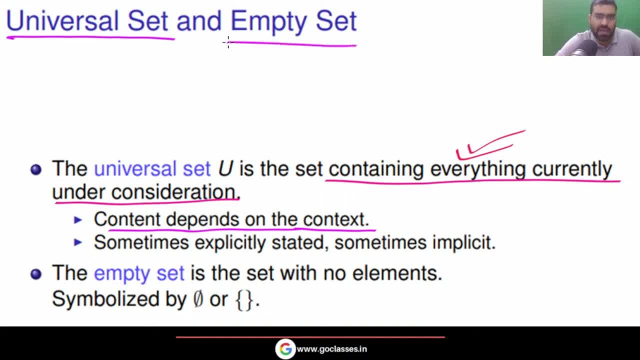 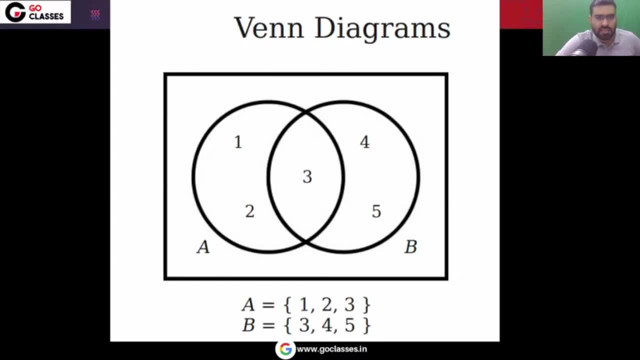 you. this is universal. it contains everything that is under consideration. empty set does not contain anything. empty set is set with no element. there is no element. now let's see. this is a venn diagram. you can notice that in the set a you have three elements: one, two, three. in the set a, this is your. 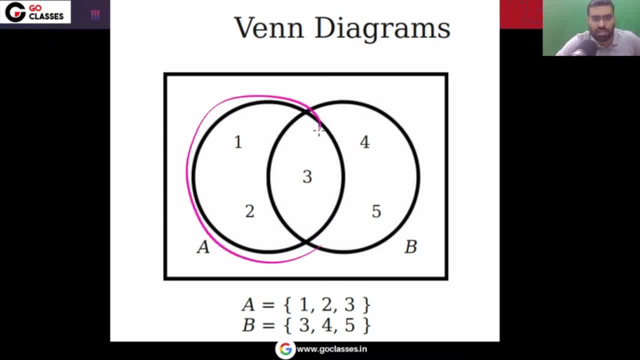 set a. you can notice in the diagram. this is a venn diagram, so this is your set a, in which you have one, two, three. these are the elements. this is a set b in which you have three elements: three, four, five. now you can do some operations. you can easily see, if i do this, what will be this area. can anyone 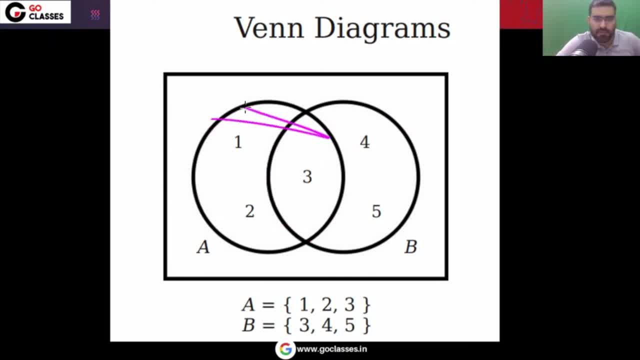 tell me quickly some questions. i am asking you, tell me if i, if i, if i ask you, what is this area? what is this area? this is the area of a. very good, okay, this is the area of a. what is this area? can you tell me what is this area? look at this area and tell me what is this area. this is the area of b. 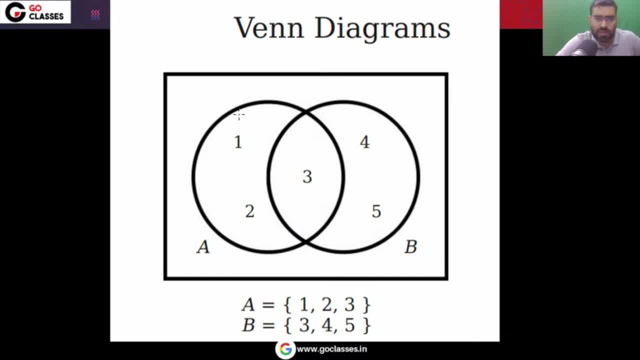 Now, what is A union B? A union B means take all the elements of A and B. Okay, this area is the A union B. So A union B is this area: All the elements of A, also all the elements of B. 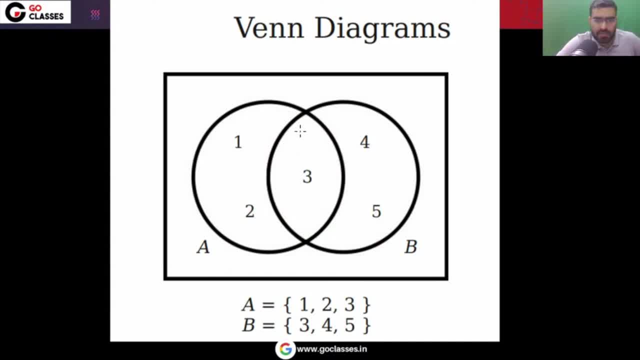 This is union. Intersection means common. These are the elements which are common. This is the intersection of A B. This is intersection. What is A minus B? Okay, set difference. What is A minus B? A minus B means: 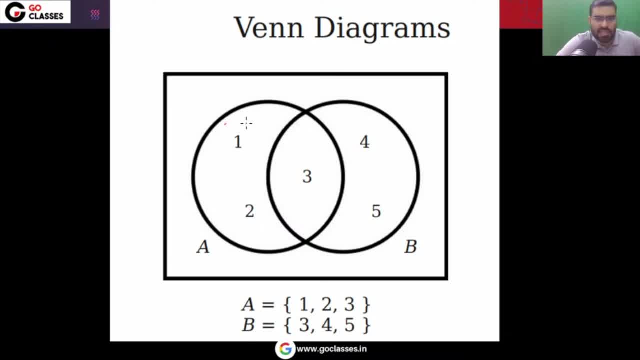 only in the A, only in the A. This area, this area means only in the A, This area is A minus B, This area is B minus A, Only in B. Okay, And this area: A minus B, Union B minus A. 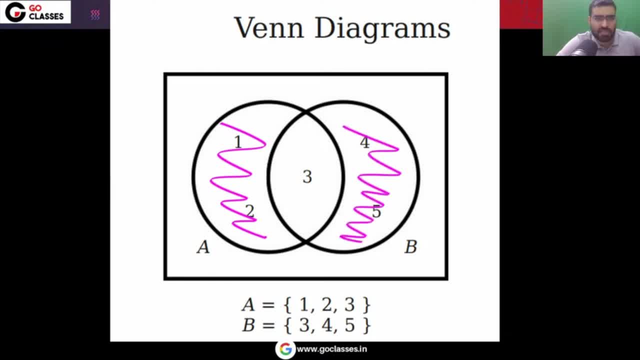 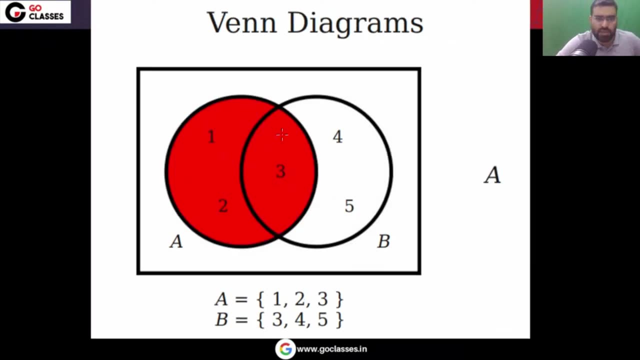 This area is symmetric difference. This is the symmetric difference. This area is set: difference A minus B. This area is set: difference B minus A. This area union, this area, That is symmetric difference. so like this you can find out, so you can easily see if i do this: this red color, this is the set. 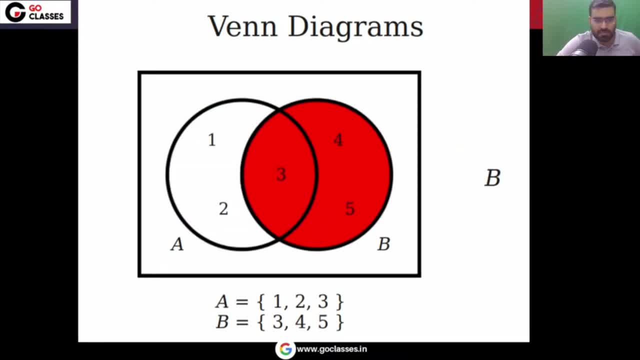 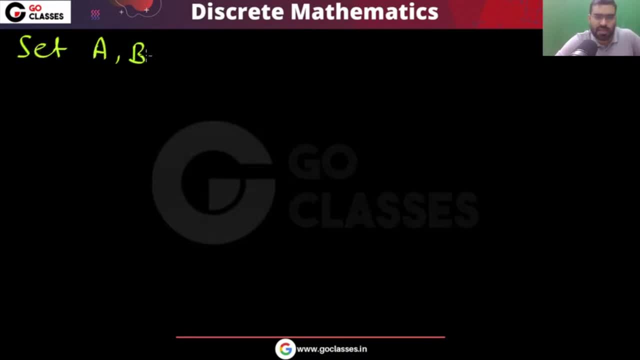 a. you can see this red color is a set b. okay, so very simple. now, what is union? now let's see if you have, if you have two set. let's assume you have set a set b, you have two set. then what is a union b? this is the symbol for union. okay, so this is your. i can say this is the symbol for union. so 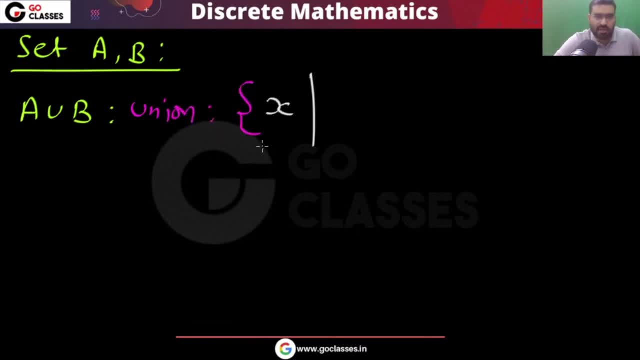 what is a union b? in the a union b you have those elements. you have all the elements of a comma b. you have all the elements of a comma b means you have those elements which are in a, so that all the elements of a comma b you have. so those elements which are in a, or this element can be. 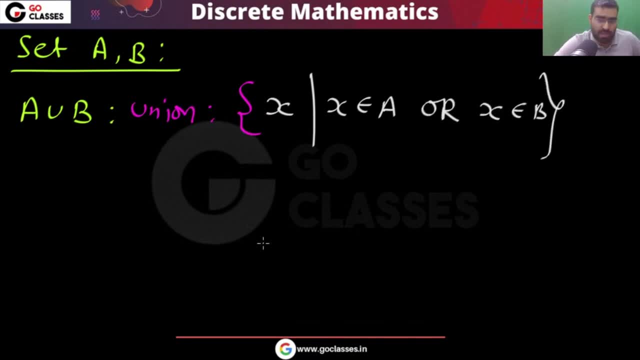 in b. so, basically, take all the elements of a, take all the elements of b. okay, take all the elements of a, take all the elements of b, take all those elements. that will be your union. next, you can notice intersection. what is intersection? what is this? intersection of two set. intersection means: 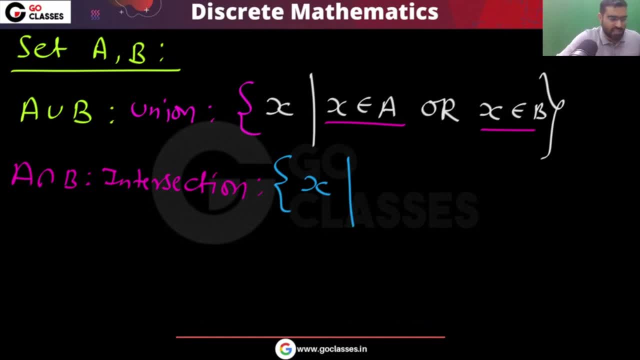 common elements, so those elements which are in both the set, those elements which are in both, which are common, which are in a also and which are in b also. okay, see, you can notice those elements, those elements which are in a and b which are common in a comma, b intersection means common. 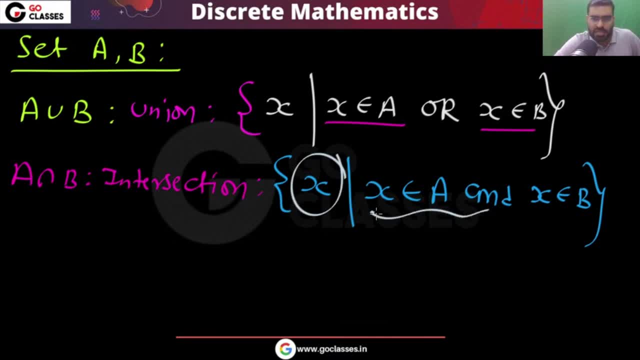 part. so this is the common part. so those elements which are in a and b. now let's see. the next is a minus b. this is called set, difference, set, difference, set, minus. in this, what you have in this you have a minus b. okay, from a you remove b means finally it will give you those elements. 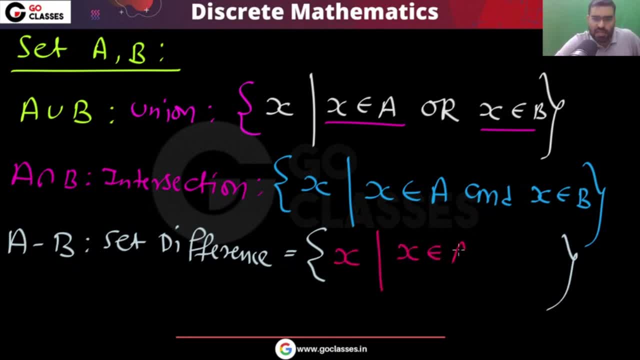 which are only in a. okay, those elements which are in a but and which are not in b, okay, so those are only in a, those elements which are only in a. that is your set difference: a minus b. so what is what will be b minus a? what will be b minus a? that will be those elements which are 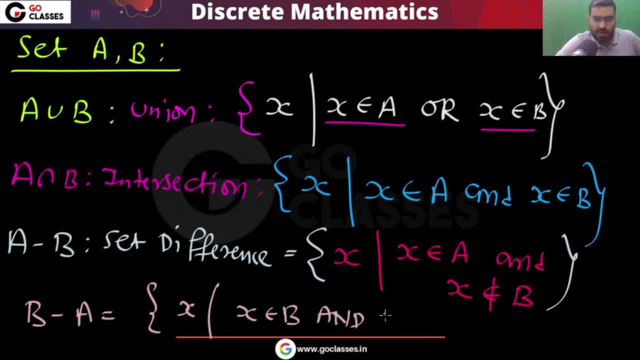 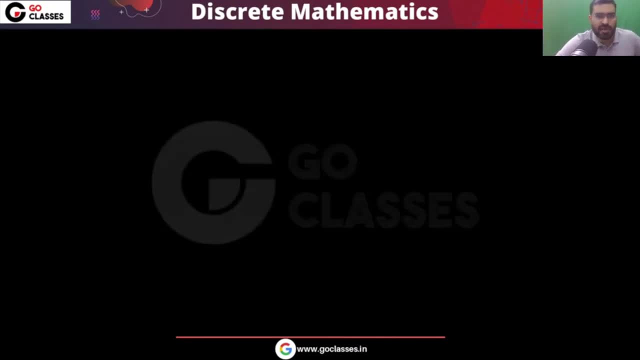 only in b, which are in b and which are not in a. okay, so they are not in a. so that is the definition of b minus a. so, very easily, now let's see the symmetric difference. this is interesting. let's see this symmetric difference. symmetric difference that is like a exclusive or okay, this symmetric difference. let me tell you. 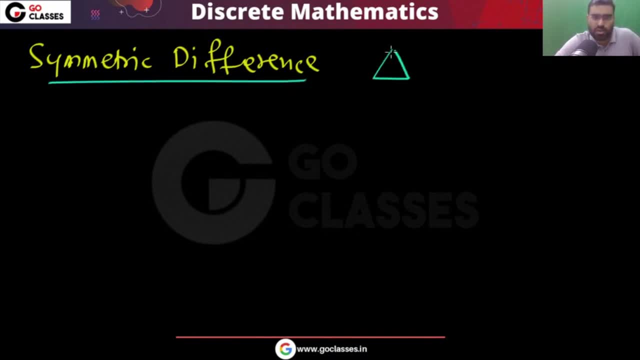 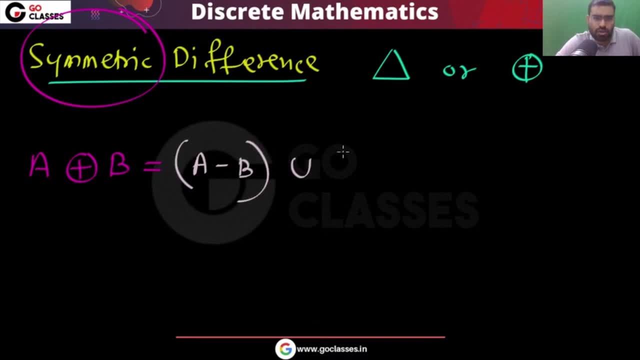 a minus b. only in a union, only in b. okay, so take the union of all those elements, so what you do only in a union, only in b. for example, if this is a, if this is b, then you can notice: only in a union, only in b. this is your symmetric difference. okay, now, very easily, you can find this. 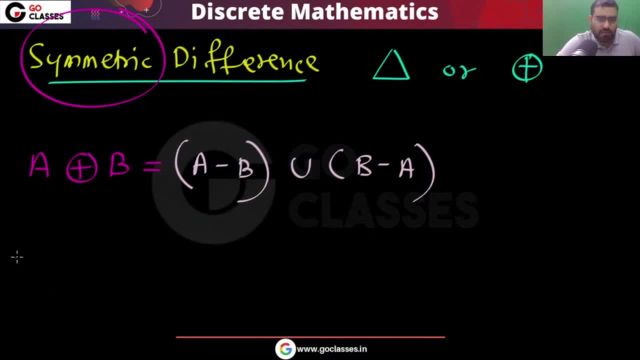 let me tell you: this definition will not help you much. what is symmetric difference? the best definition is this: what is the best definition? this is exclusive elements of a comma b. okay, set of exclusive elements of a comma b. i can say: set of exclusive elements, exclusive elements of a comma b. that is the reason you can also call it exclusive or. 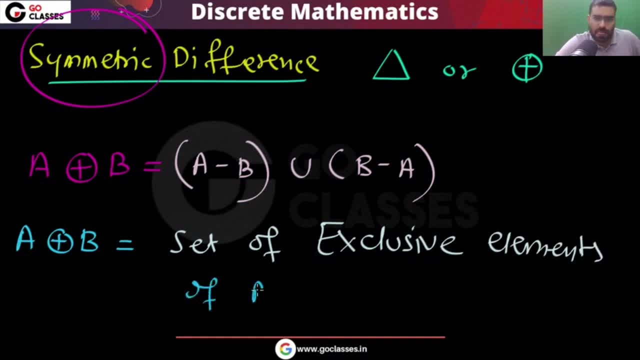 set of exclusive elements of a comma b. exclusive elements means those elements which are only in a or those elements which are only in b. c, set of all exclusive elements means only in a or only in b. so those elements which are exclusive, okay, which are exclusive elements of a comma b. so that set is called, uh, symmetric difference, so the symbol you can use. 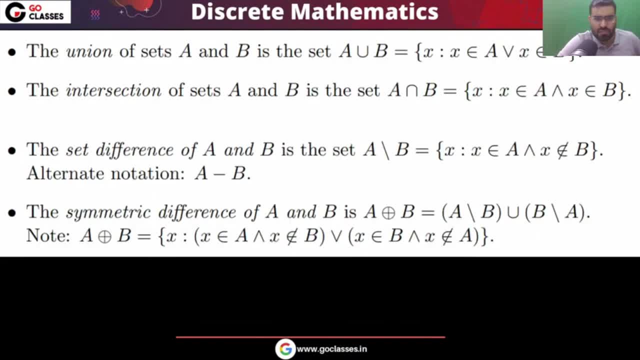 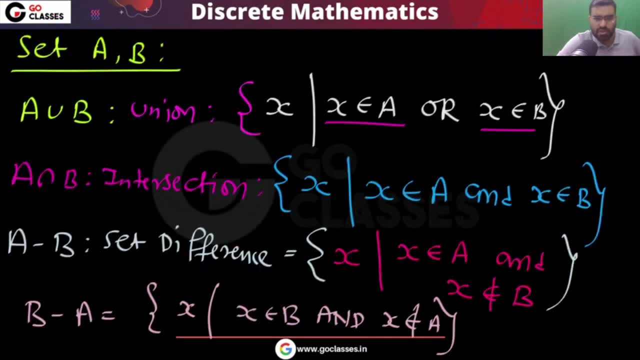 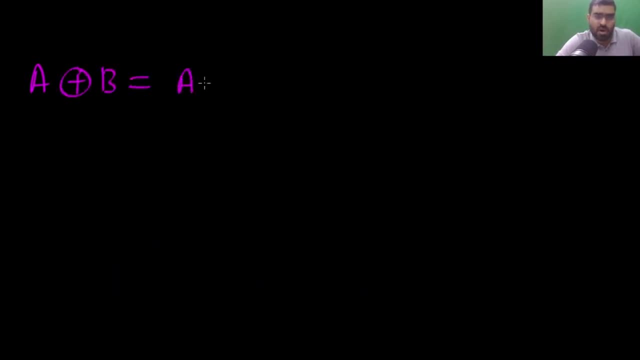 this symbol or you can use this symbol: this is the symmetric difference. very easily you can see. okay, now let's move on. another definition you can see for the symmetric difference. if you want see the symmetric difference definition, you can also see like this: this is the symmetric difference. 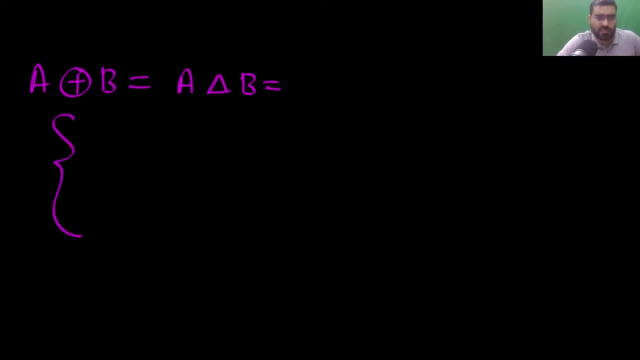 or you can use this symbol and this definition will be like this: you have those elements, okay, either this would happen: either it belongs to a and it does not belong to b, okay, either it is only in a. i can say: either this element only belongs to a, or what happens, or what happens. 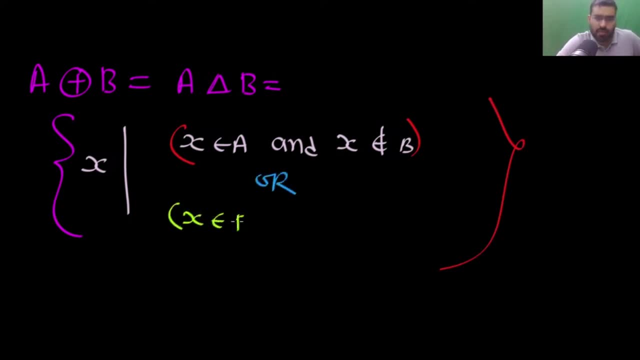 or this happens, that it only belongs to b. x belongs to b and x does not belong to a. so either it only belongs to a or it only belongs to b. this is the definition of symmetric difference. let's move on now. the next definition is complement of a set. 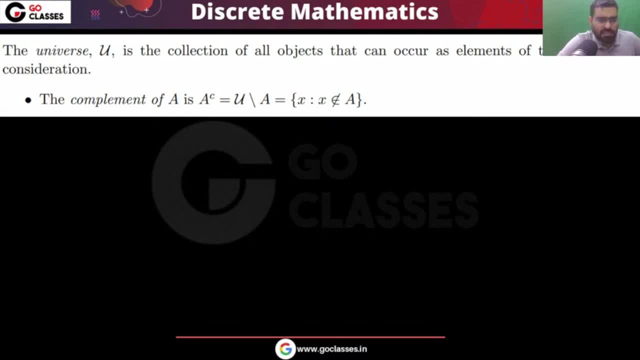 complement of a set, as i told you, that is, all the elements which are not in the set. so if you have a set s, then what is complement of this set? as? or you can say as this, or you can say negation of s, or you can say negation of s. all these are same, okay. so what it simply. 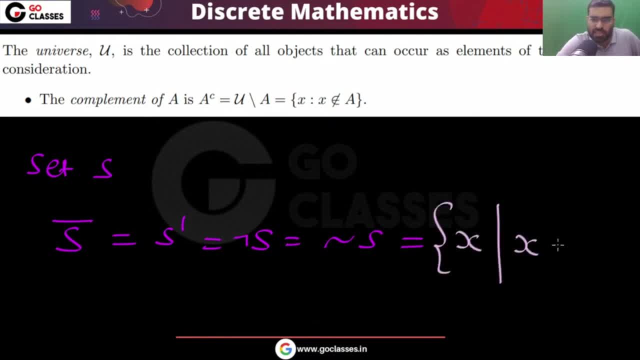 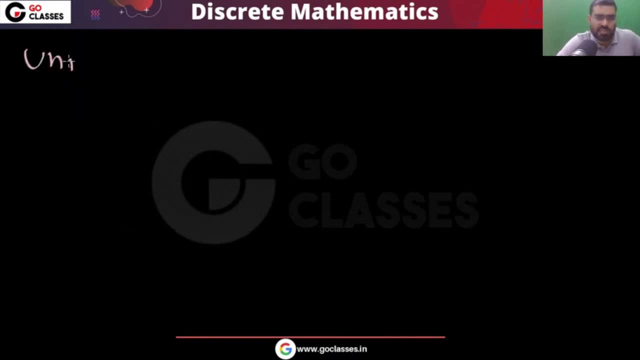 means? it simply means that all the elements which are not in the set, as all the elements which are not in the status, so of course these are in the universal set. so let's assume you have a universal set. universal set contains everything, remember. let's assume you have a universal set m, then in: 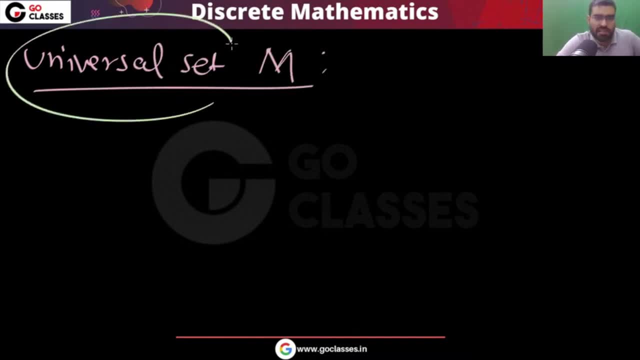 this situation? uh, you can notice that it contains everything. remember, this is the definition of universal set. universal scent contains everything. like this: is your set m. it contains every element. Ok, this universal set. it contains every element. so you can see that every set will be subset of itself, whatever set you take. 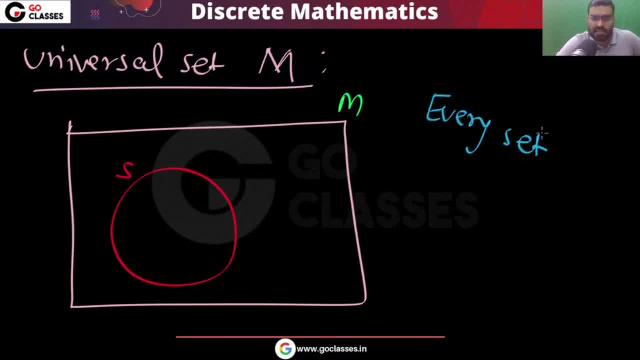 So you can easily see that every set under consideration, every set, whatever set you take, that is a subset of universal set, Because universal set contains every element. So every set is subset of universal set. Now you can easily see if this universal set contains everything. 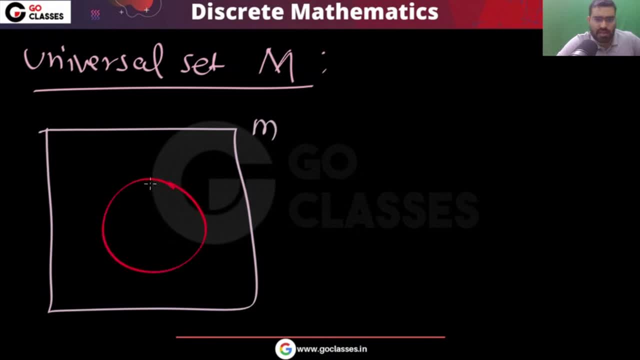 Now, if you have a set S, this is your set S, let me assume this is the set S- Then all the elements which are not in this set S, all these elements, this is called. this is called S complement. S complement means I can say S, complement means M minus S. 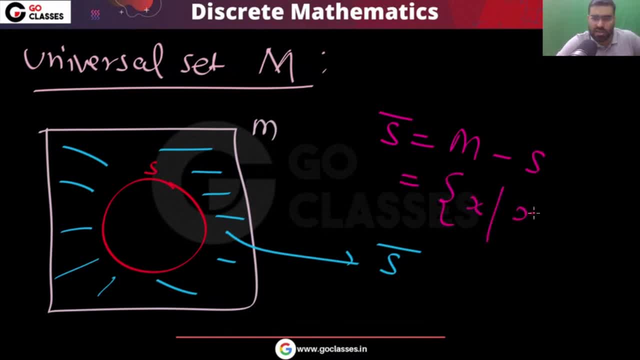 Okay, all those elements, all the elements which are not in S, of course they are in M. Okay, of course, because in this universal set you have all the elements, so of course those are present in M. Okay, of course, because in this universal set you have all the elements, so of course those are present in M. 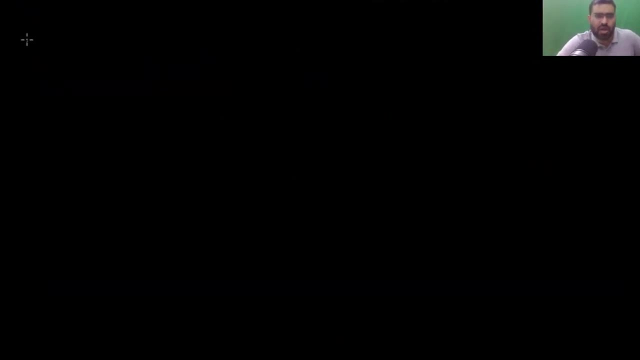 so this is the definition. also, i want to tell you one very important thing: that this symbol for the set difference symbol, set difference symbol. most of the time they will use this symbol. either you can say that a minus b, either you can use this symbol or you can use this symbol. so either this symbol will be used or this symbol will be used. 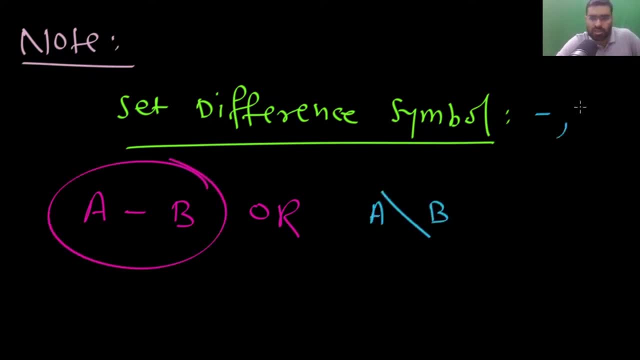 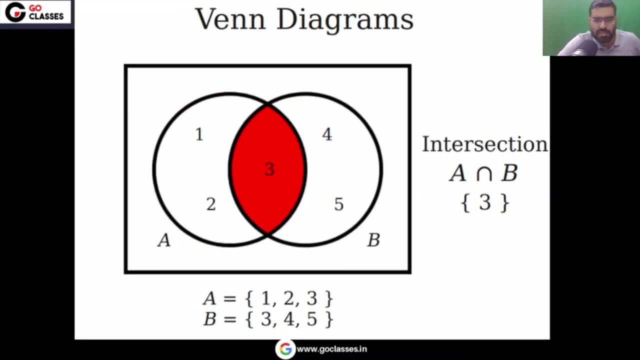 backslash. so this symbol, remember, either you can use this symbol or you can use this symbol. both are the symbol of set difference. now let's move on. so you can notice, this is the union of a comma b, this is the intersection of a comma b. and when can we say that two set are disjoint? when their 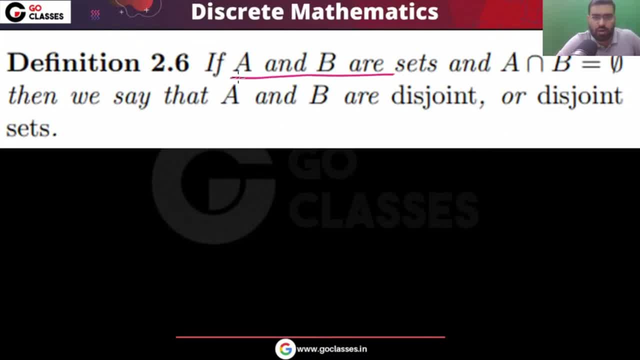 intersection is phi. okay, so this is the. this is the definition. a, comma, b are set and their intersection is phi. if intersection is phi, nothing is common, intersection phi means nothing is common, then they will be called disjoint set, okay. so remember, if you have two set, set a and set b, and if their intersection is phi a, intersection b. 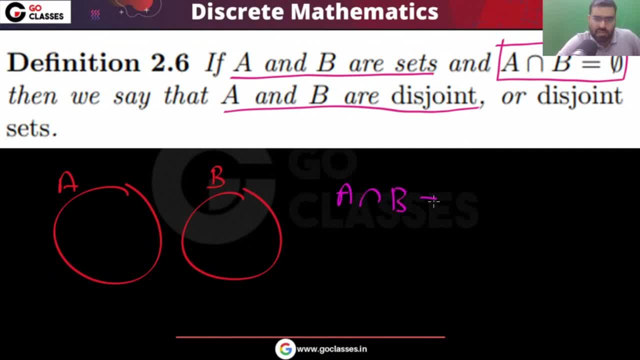 if they had. if they don't have anything common, there is no element which is common. if their intersection is phi, then then a comma b are disjoint, okay, then a comma b are called disjoint. they are disjoint from each other. they are completely disjoint from each other, okay, so? 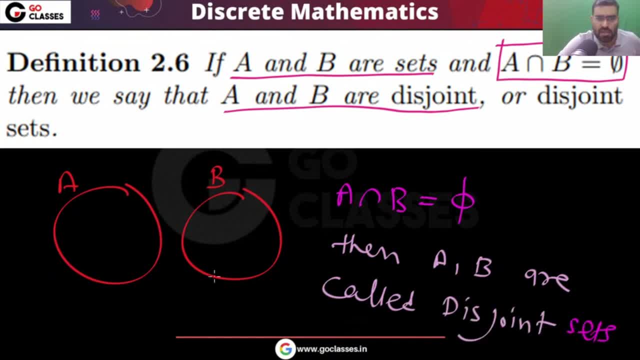 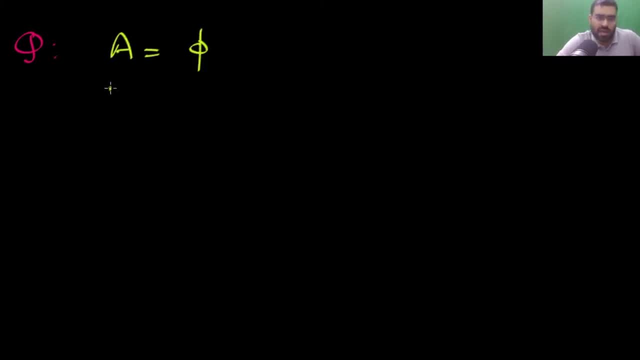 this is the definition of disjoint set. so they are disjoint sets. okay, now you tell me simple question. i am asking: what about phi, comma phi? let's assume a is phi and b is phi. are they disjoint? are these two disjoint, these two set? are they disjoint? yes, they. 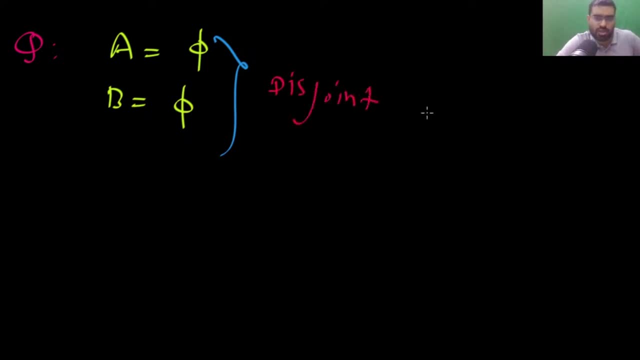 are also disjoint. all you have to do just apply the definition. they are disjoint because you can see a intersection, b is phi. there is no element which is common in these two. remember, in this and in this there is no common element. we don't have any common element. so these are designed. 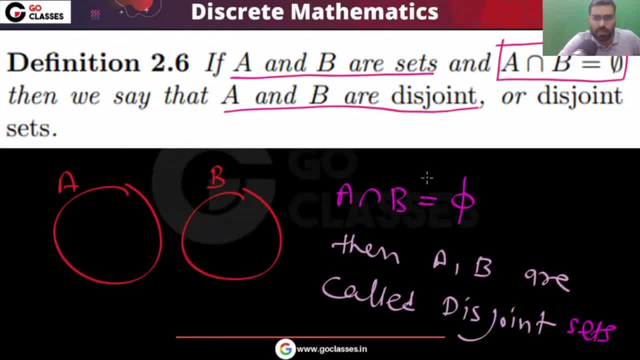 designed means they don't have any common element. so the definition you can apply. this is the definition of design. so whenever you are in the confusion, then remember, just apply the definition that a copy are designed. if their intersection is a fine, okay, let's move on. you can consider. 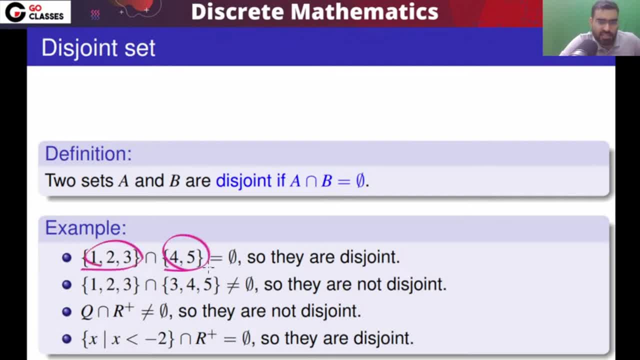 these examples like: this set has one, two, three, three elements. this set has four, five, two elements. their intersection is five, so these two elements are these two set. this set and this set are designed. you can notice, this set and this set is not designed because they have some common element. 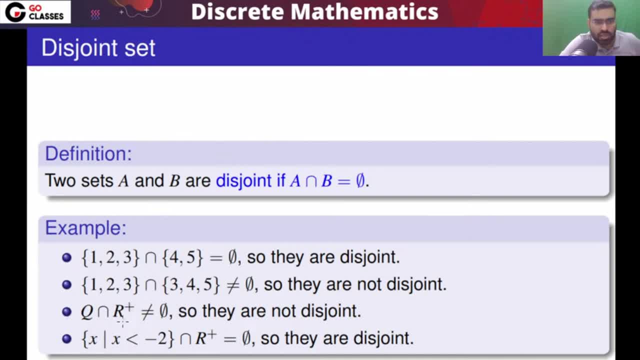 at least one common element. these two you can notice they are not designed. and you can notice that these two are designed okay. so here you have positive real number and here you have real numbers less than minus two. so they don't have anything common, so they are also designed. let's 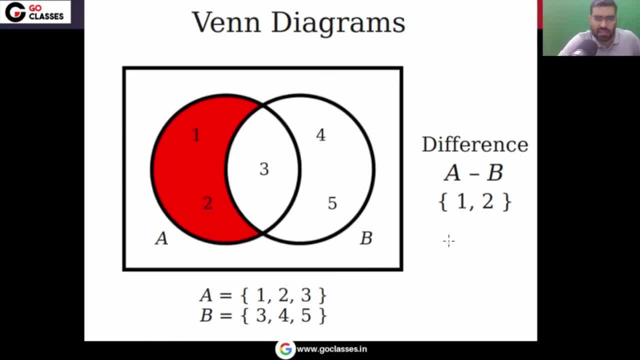 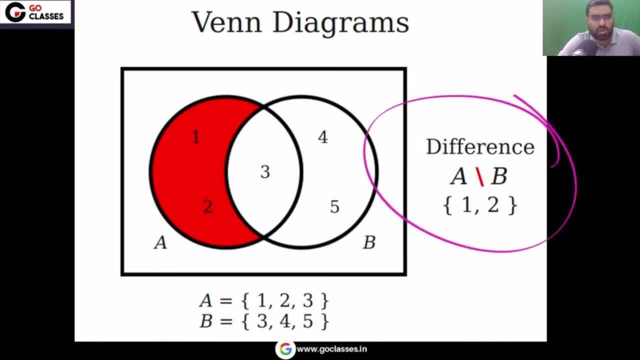 move on so you can see. this is a minus b. this is set difference. or you can use this symbol a backslash b, this symbol also you can use. so, as you can notice, this symbol also can be used. this is your definition of set difference. this is your. 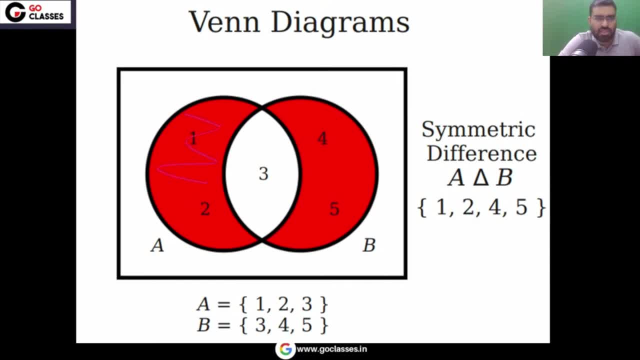 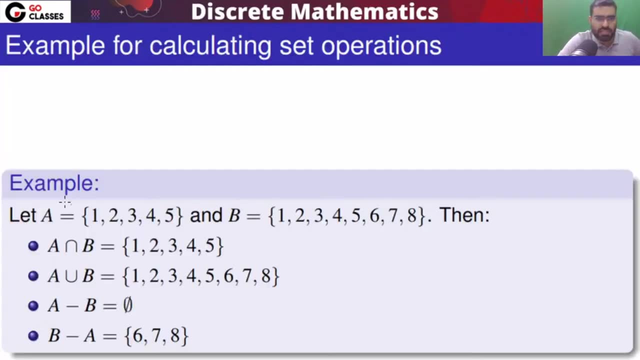 symmetric difference. symmetric difference means all the exclusive elements, those elements which are in a, only in a or only in b. this is called exclusive symmetric difference. so this is like this: a minus b union, b minus a. now let's move on. so you can easily see this example, you can 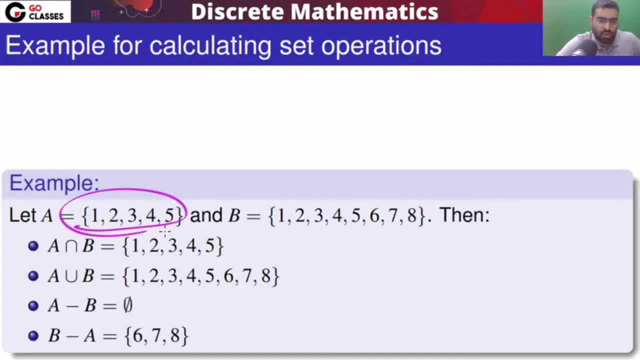 see this Out: you have a set a in which you have five elements: 1, 2, 3, 4, 5. you have another set b in which you have, uh, one, two, three, four, five, six, seven, eight. so you can see what are the common elements you can see as a subset of b. you can easily see every element of a as element of b. 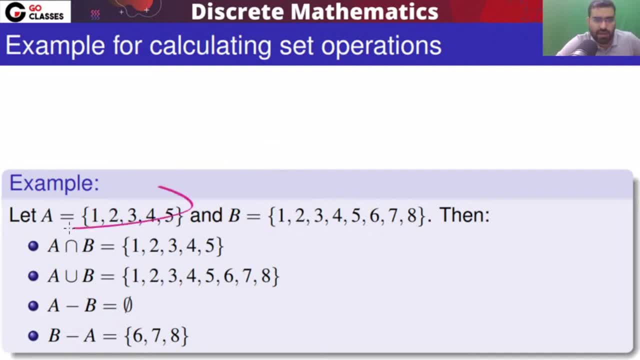 every element of a element of b. okay, every element of a is element of b. okay, you can from this example, you can easily see from this example that a is a subset of b. this ai, This is a subset of B. This is your A In A. whatever you have that is also in B. 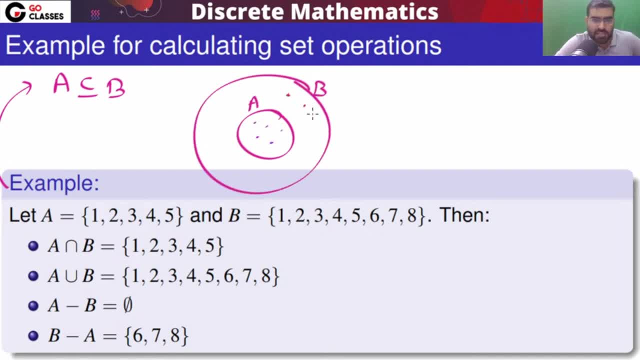 Okay, every element of A is also element of B, But there are some extra elements in B, So I can say: A is a proper subset of B. This A, this is a proper subset Because A is not equal to B. 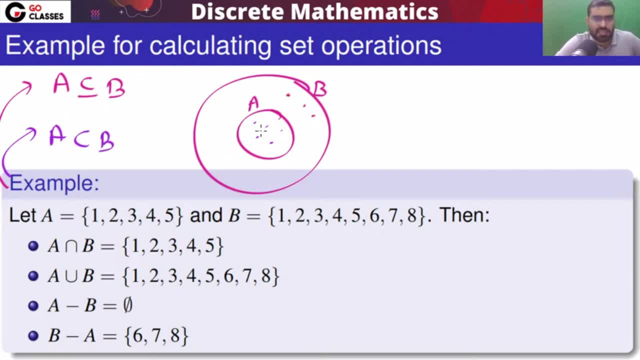 So you can see that whenever A is subset of B, then their intersection will be A. Okay, so you can easily see their intersection is A, Because the common area will be this: A, Now what is A? union B, That will be B. 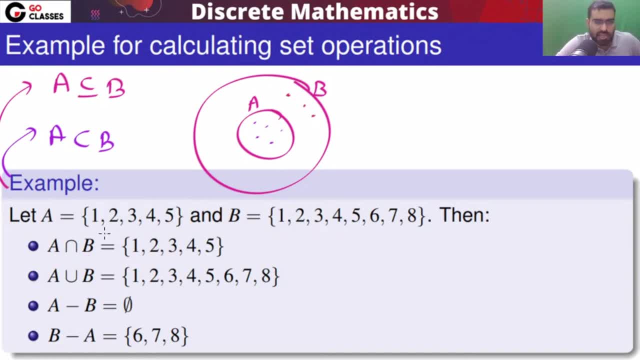 What is A minus B? That will be phi. You can notice. there is no element which is only in A. A minus B means all those elements which are only in A, But there is no element which is only in A. B minus A will give you these elements. 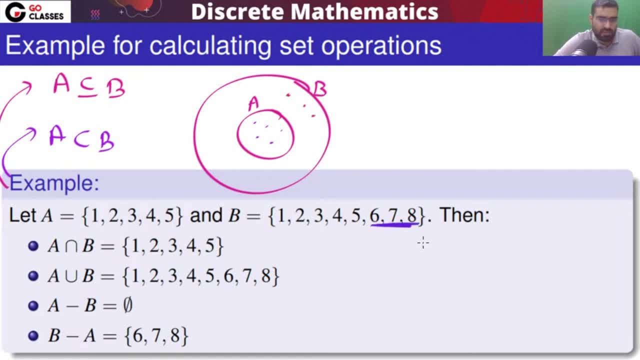 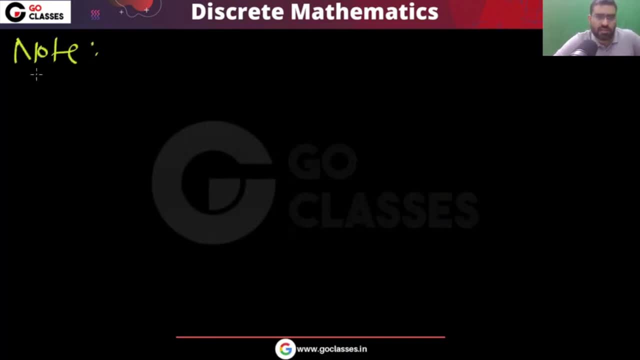 These are B minus A. These elements belong to only B, They do not belong to A, They only belong to B. So this is B minus A. Now some important note you can see. Tell me some questions I am asking. 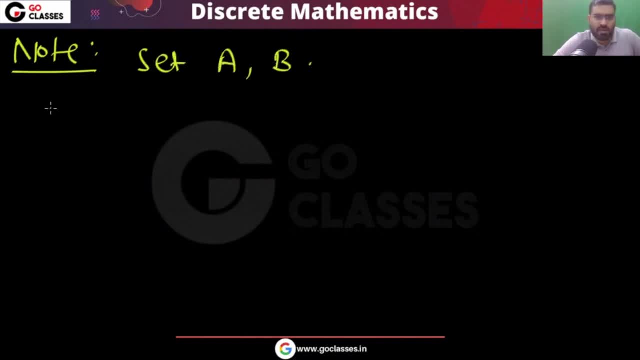 You have set A, comma B. Let us assume Set A set B, If A is subset of B, If this A is subset of B, then which will be true? Some options, I am giving you Some options. I am giving you like. 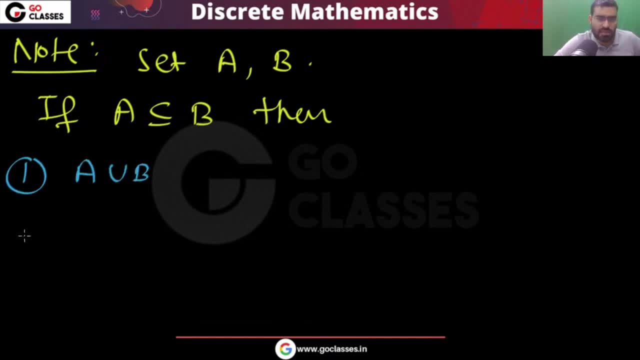 What can you say about A union B? What can you say Like: what can you say about A union B? What can you say about A intersection B? What can you say about B minus A? What can you say about A minus B? 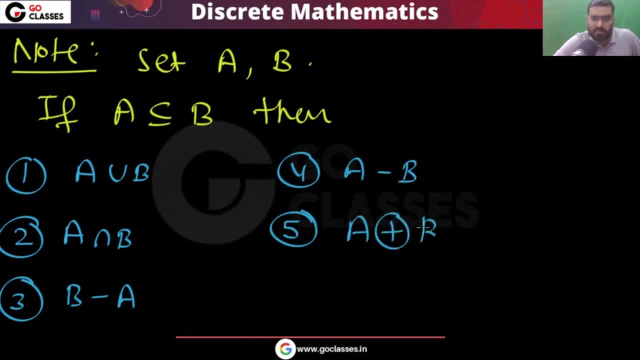 What can you say about A symmetric difference B? What can you say about Aba? What can you say about A complement? What can you say about B complement? What can you say about A complement? What can you say about B complement? So these things, some questions I am asking. 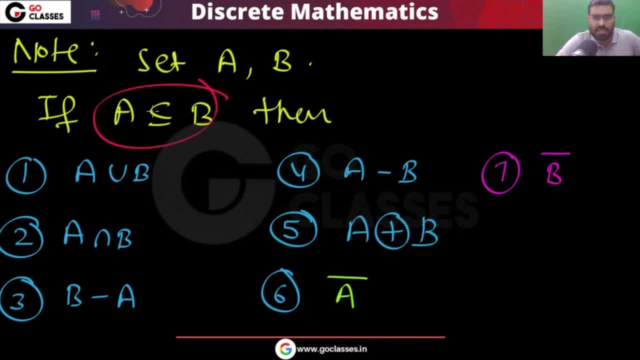 Tell me the answer. If A is subset of B, this A- Remember, this A- is a subset of B, This A, every element of a, is also element of b. so this a is subset of b, then their union will basically be same as b. okay, all the elements, a, union, b. so there you can notice, the union will be same as b. 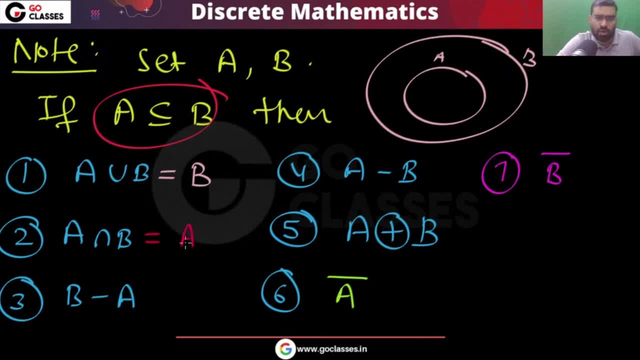 the intersection will be same as a. the intersection, the common part, will be same as a. next, what is b minus a? that can be something we cannot say anything about it, yes or no? we cannot say anything about it. b minus a means those elements which are in b, not in a. so we cannot. 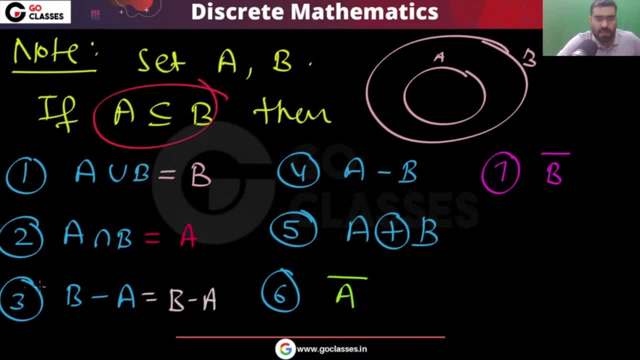 say anything about it. we can just simply say: b minus a means b minus a, but what is a minus b? that is definitely phi. okay, that will definitely be phi, because there is no element which is in a but not in b, there is no element which only belongs to a. what about symmetric difference? 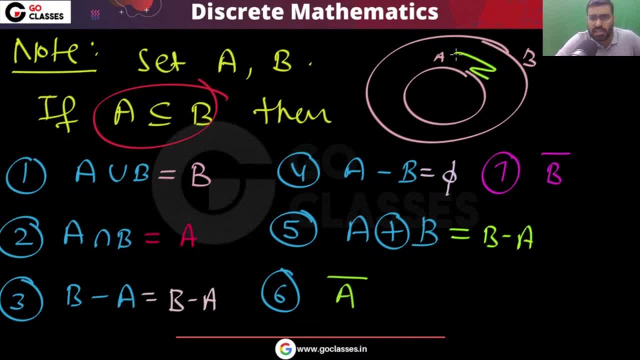 this will be same as b minus a. only these are the exclusive elements, only these are the exclusive elements in a comma b. okay, so a exclusive asymmetric difference b, that will be b minus a. we cannot say anything about b a complement because, remember, the universal set can be anything. 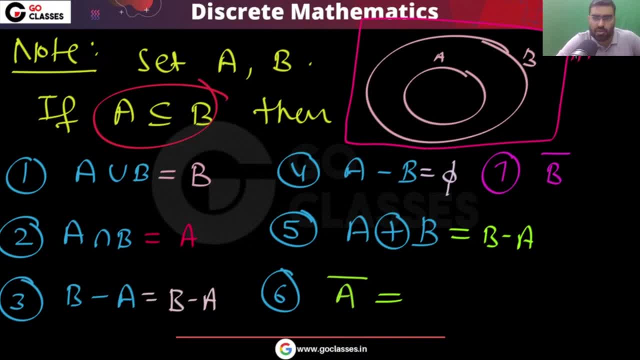 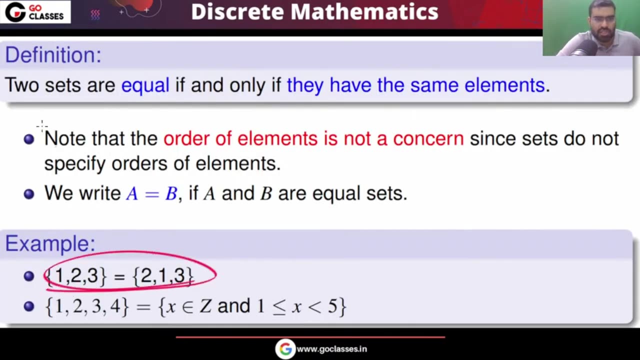 remember, remember, remember the universal set. the universal set can be anything, we don't know. so the a complement is simply, i can say, m minus a and the b complement is simply m minus b. okay, so very simple, like this you can find out. now, you can, you can see here these two set are: when can i? 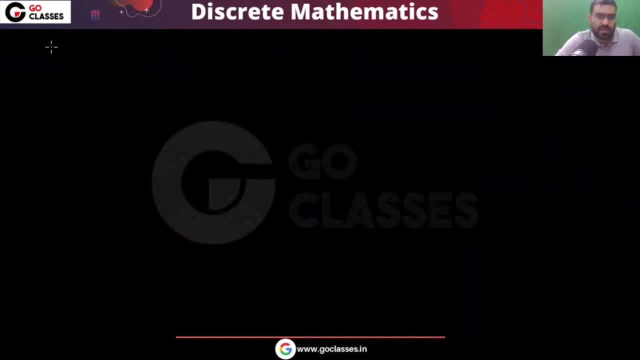 when can i say two set are equal? when can i say that two set are equal? this is very important because you will use this in a many question. if you have set a comma b, then when can i say a is equal to b? these two set are exactly equal. when can i say they are equal? if, and only if, see these: 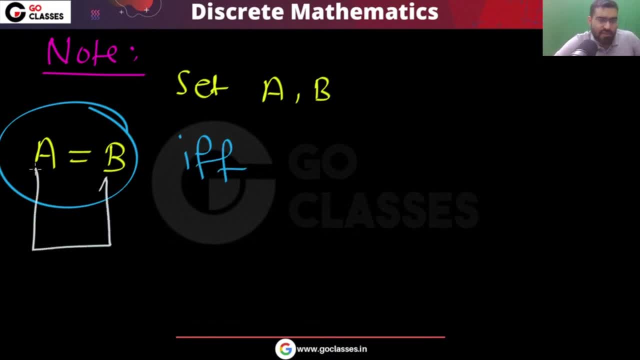 two set are equal means every element of a is element of b and and, and every element of b is element of a, every element of b element of a. okay, i can say that a must be subset of b and every element of b must be subset of a. so b must be subset of a, so i can say a is equal to. 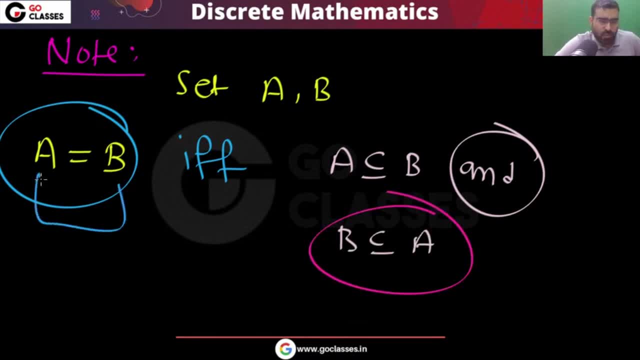 b. if, and only if, a subset of b means a subset of b- every element of a is on is element of b and every element of b is element of a- then we can say that they are equal. they are exactly equal if, If A is subset of B and B is a subset of A, 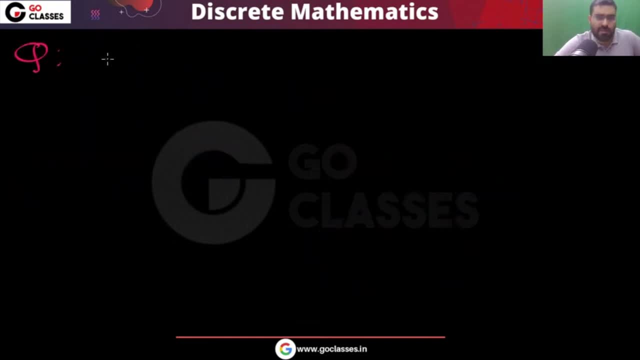 Okay, so very simple. Now you tell me a simple question Again. I am asking that if you have a set in which you have 1,, 2, 3 and you have another set, Let me assume you have 1, 1,, 2,, 2,, 2,, 3,, 3, 4.. 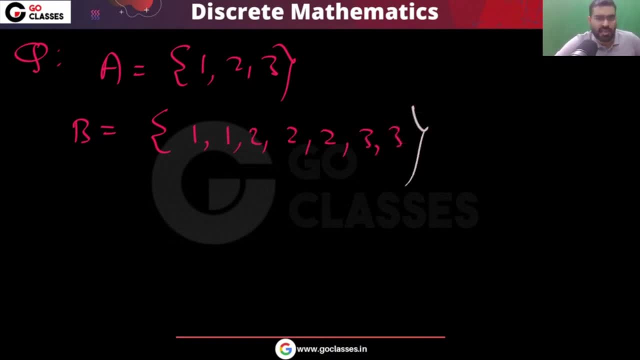 Now you tell me what about this set. Can I say they are equal? Can I say A is equal to B? Can I say they are equal, Yes or no? Yes, of course they are equal. Yes, of course they are equal, because every element of A is element of B. 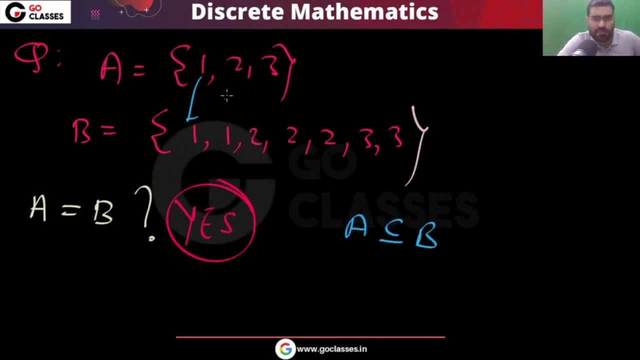 You can notice that every element of A is element of B, Like every element of A is element of B. You can see, And every element of A is element of B And you can notice that every element of B is element of A. 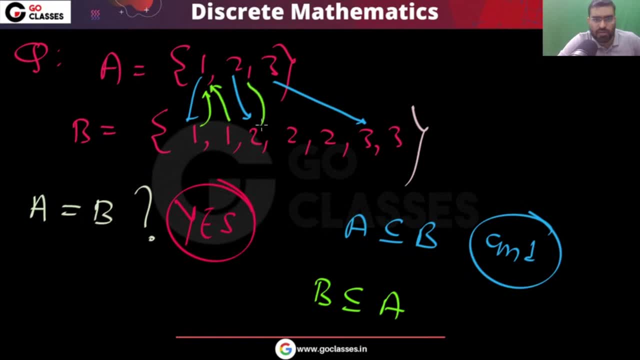 Like you can notice, every element of B is element of A. Okay, every element of B is element of A. So you can easily see, Very easily, you can see that every element of a element of B and every element of B is element of. 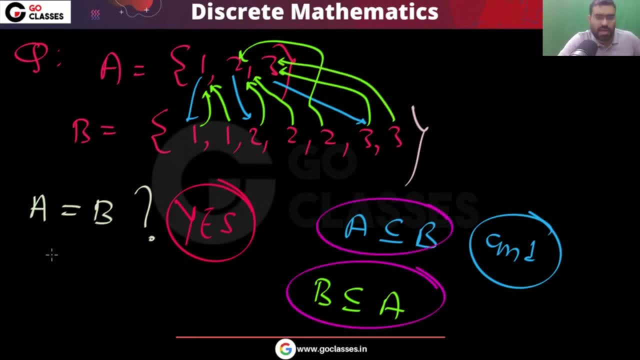 A. So that is the reason I can say they are same. So remember, A, comma, B are same set. So because you so, finally I can say you can remove the duplicates in the set. Duplicate does not matter. So, as I told you, the cardinality of this set is three. The cardinality of this: 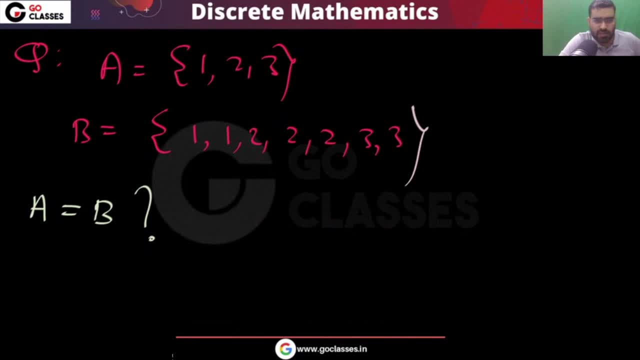 set is also three. So this is the definition. When can I say two set are equal? This is very important, that if you want to check how to check how to prove how to prove that some set A is a subset of set B, OK, like how to prove this. This is very important. 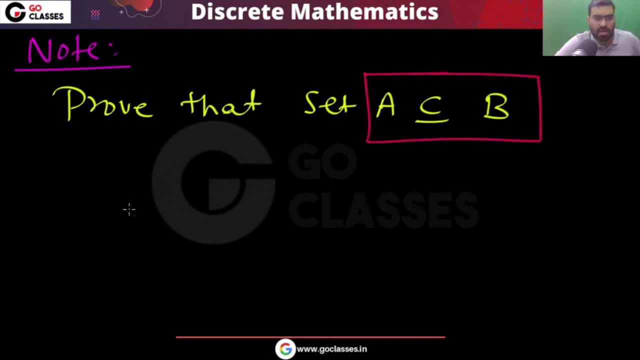 How to prove that A is subset of B. Let's see this: How can we prove that A is subset of B? So very simple. The proof is very simple: Just use the definition. All you have to do, just use the definition. 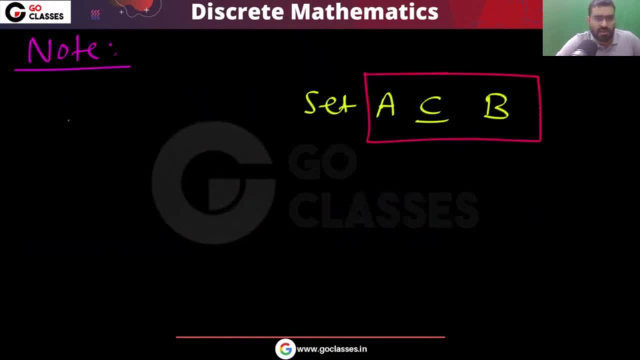 What is the definition? What is the definition? Let's see, Just use the definition. You tell me about the definition of when can I say that A is a subset of B? A is a subset of B. This is the definition, for this is this is the definition that I can say A is a subset of B if, and only if. 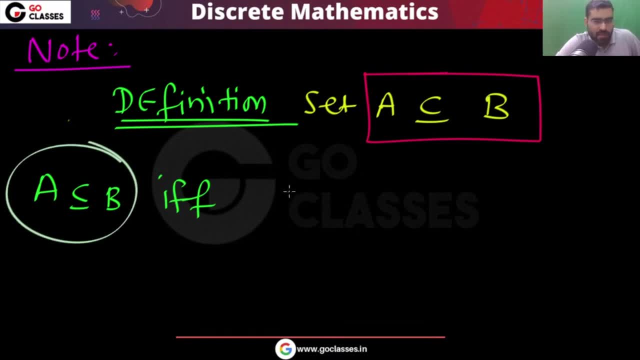 What will happen? This will happen that for any random element. OK, for if X belongs to A, then this X should also belong to B. OK, this is the definition. If anything belongs to A, if any element belongs to a, if this X belongs to A, then 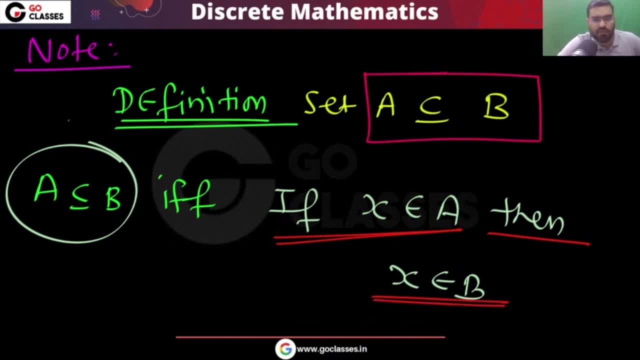 it also belongs to B. OK, so this is the definition of a subset of B, where X is a random element. This X is a some random, any random element, any, I can say random, arbitrary element. This X, this is arbitrary element. So you can take a random element, X, And if you can, 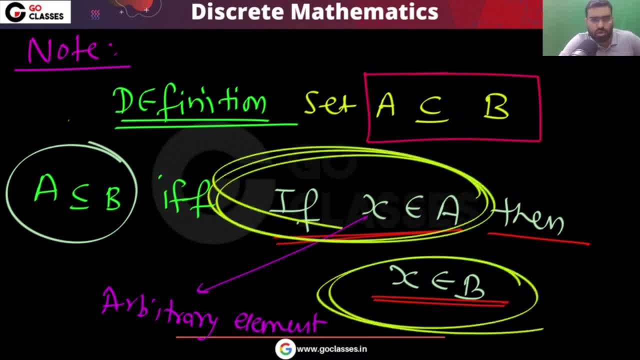 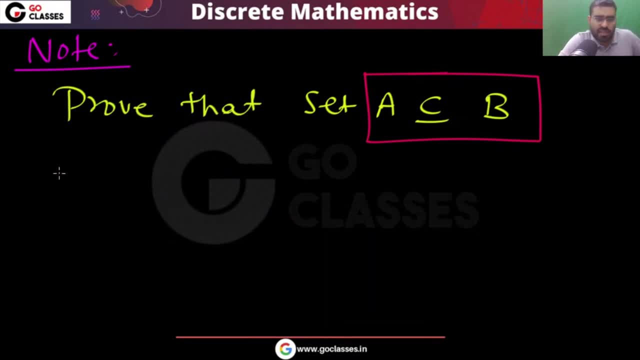 prove that if this X belongs to, then it will also definitely belong to B. then we can say: A is subset of B. This is the definition. Now, how can you prove this Very simple? Take arbitrary element belonging to A. This is what you can do. 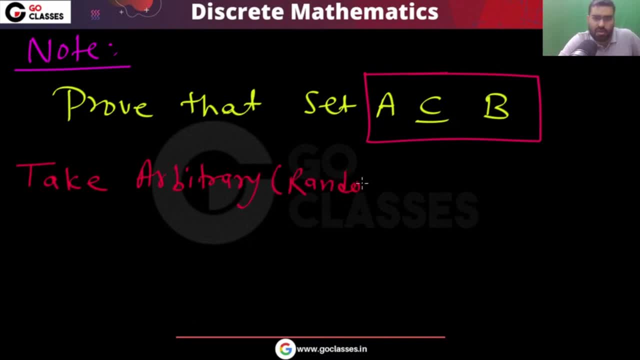 You can take arbitrary. arbitrary means random. Okay, so take a random element x that belongs to A. Okay, so this is what you do. Take, assume. I can say you take, or I can say you assume, So this is what you do. 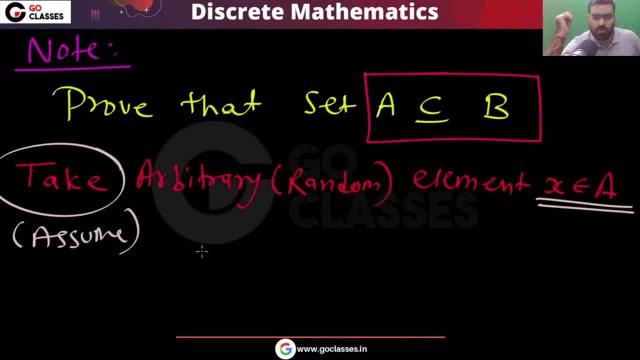 You assume that x belongs to A. This is what you assume. Okay, then prove, then show, then show that x also belongs to B. Okay, so very simple. If you want to prove that A is subset of B, then what you do. 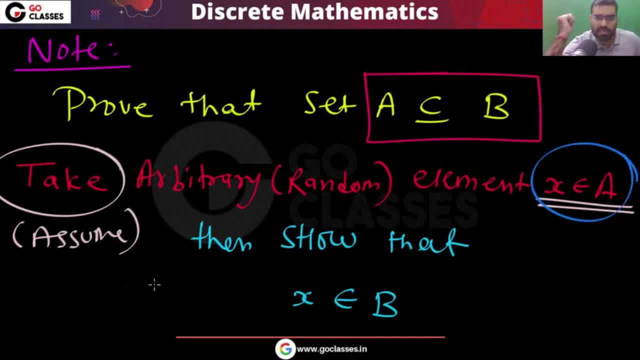 You assume some arbitrary, random element which belongs to A. This is what you assume. You start here And then you show. then you prove that x also belongs to B. Like this you can prove that A is subset of B. How can you prove B is subset of A? 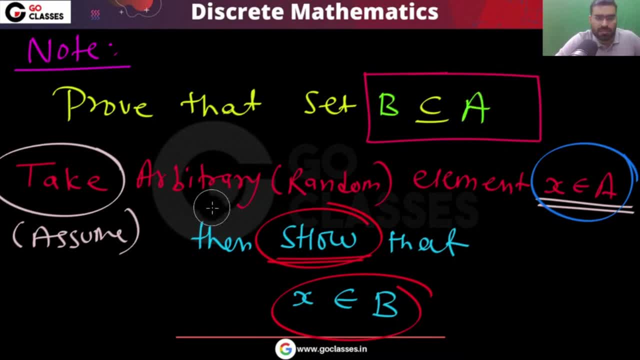 How can you prove that B is subset of A? B is subset of A means you take some random element in B. You take some random element in B And then you prove that if it belongs to B, then it also belongs to A. 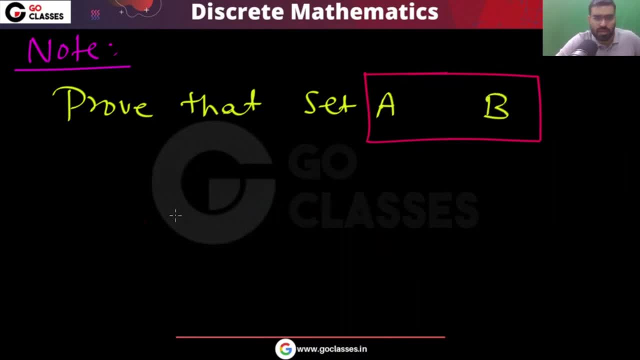 Now how can you prove that A is equal to B? How can you prove that A is equal to B? So there are two things you have to do: Prove: prove A is subset of B And prove B is subset of A. 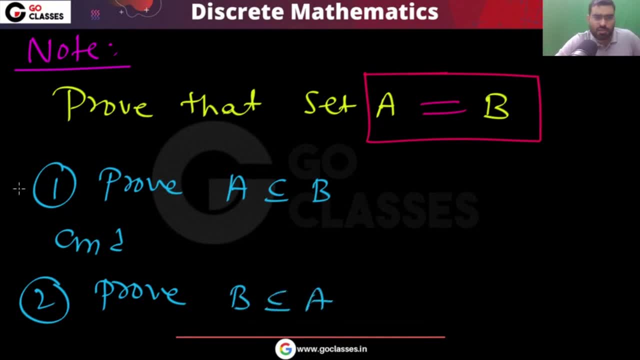 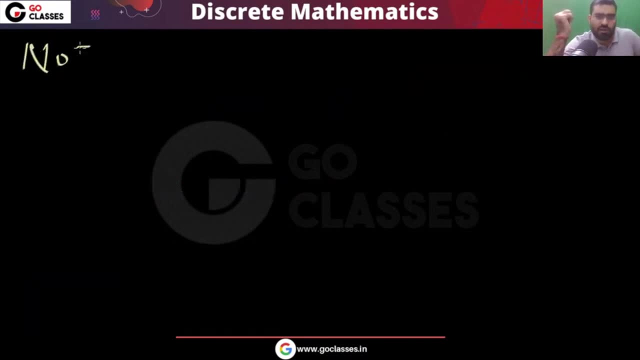 Okay, so prove A is subset of B And B is subset of A. So this is what you can do, Or you can use the Venn diagram. Okay, so this is the important note I want to tell you. Then most of the set theory questions: 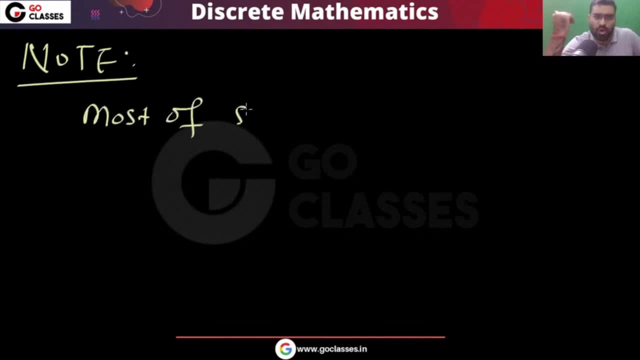 you can solve using Venn diagram. Okay, most most of set theory questions. Most of set theory questions easily solvable using Venn diagrams- Easily solvable using Venn diagrams. So many many set theory questions you can easily solve using Venn diagram. Many, many set theory questions. 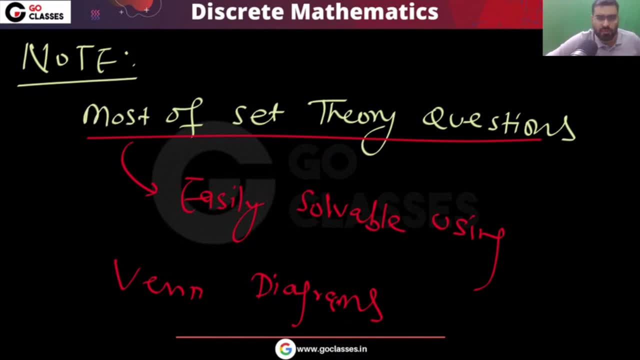 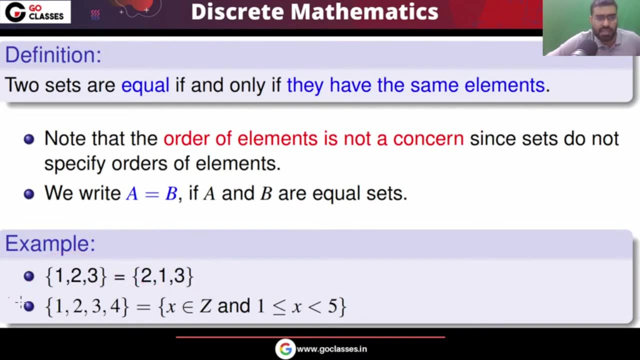 Many of I can say most Okay, or I can say many, whatever. So now let's move on. So, as you can see, these two set, look at these two set. This set is equal to this set. They are definitely equal. 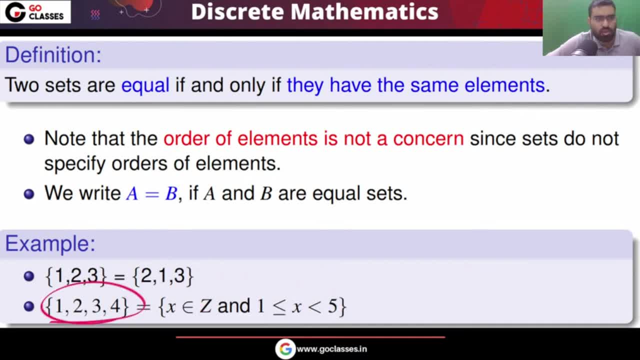 This set is equal to this set. You can see that in this set you have four elements: 1,, 2,, 3, 4.. In this set you have those elements which are integer but greater than equal to 1, less than 5.. 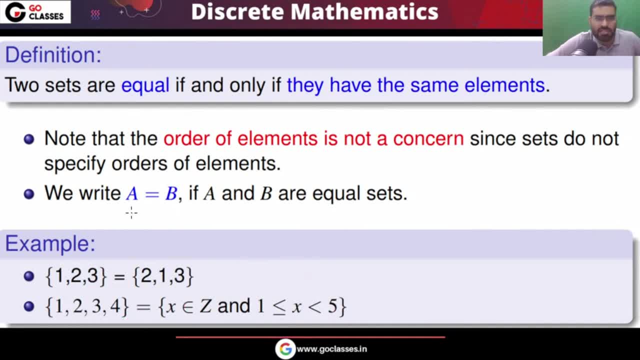 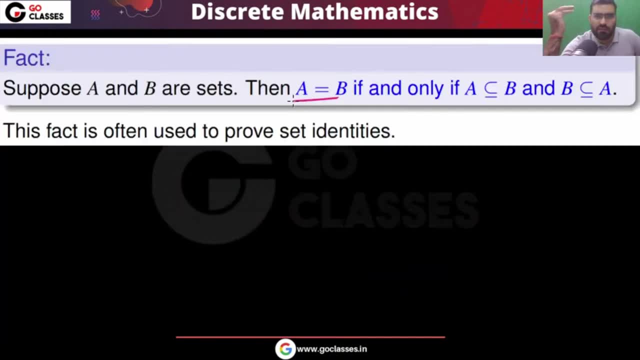 So these two set are basically same. They are equal. So I can say: A is equal to B if they are equal set. Now let's move on. So you can see that if A equal to B, if and only if A is subset of B, 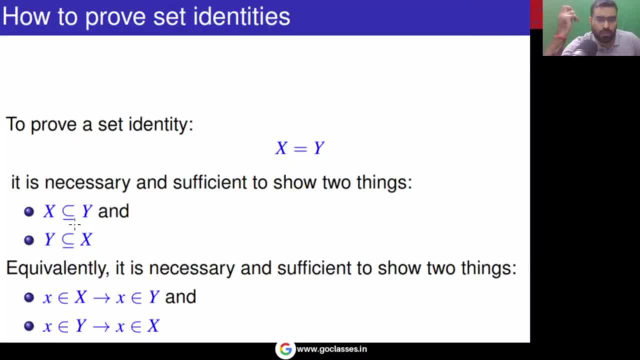 A must be subset of B and B must be subset of A. How can you prove that X is subset of Y? How can you prove this? To prove this, you have to prove that if X belongs to X, then X also belongs to Y. 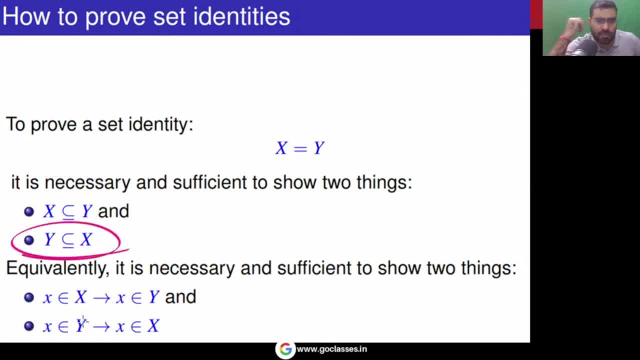 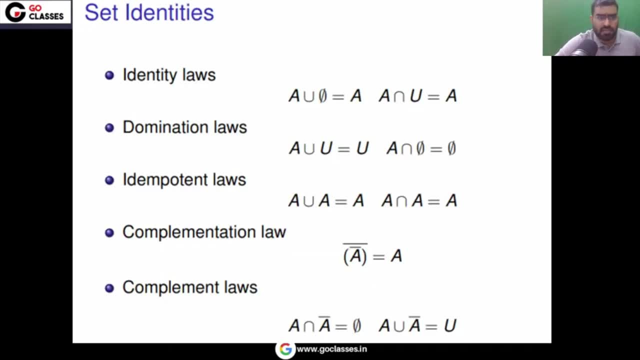 Okay, similarly, if you want to prove this, then you have to prove that if X belongs to Y, then X also belongs to X. So this is how you can do. Okay, now let's see some set identities. These are the laws. I will not give you the proof, but these are very, very, very important. 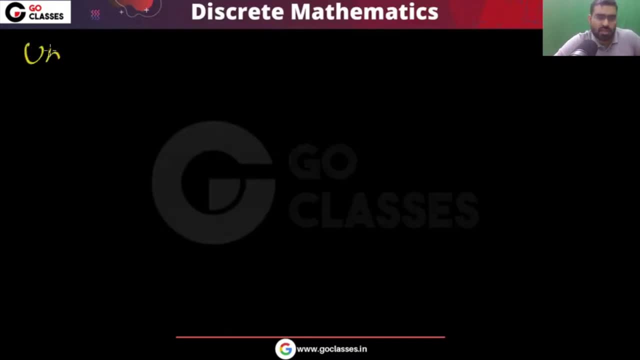 So, for example, if you have universal set- Universal set is M, Let's assume you have universal set M- Then some things will happen. If you have universal set M, then what will happen? This M contains every element. Okay, then, first of all, whatever set A you take, 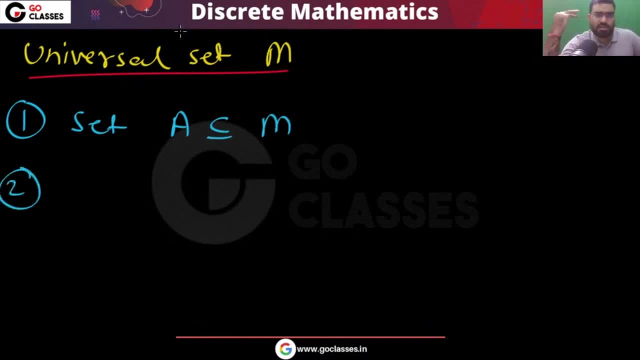 that will be subset of M. Okay, whatever, because this is universal set. It contains everything. This universal set contains all the elements. Every element under consideration is also there. So you can notice: whatever set you take, that set will be here. Whatever another set you take, 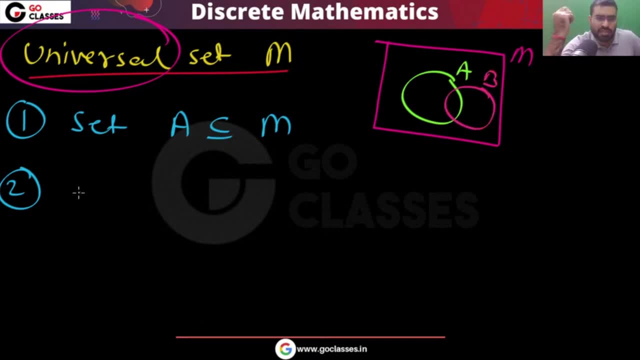 that will be here, So you can easily like this. Now, what is the second rule? The second rule is: if you take A subset of A intersection M, that will be very simple. That will be A, because A is subset of M. So A intersection M, the common part will be A. 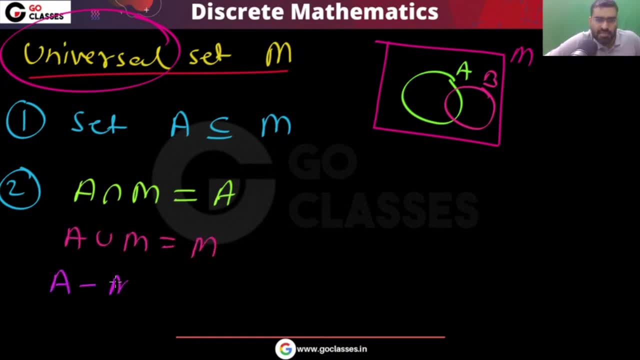 If you take A union M, that will be M, If you take A minus M, that will be phi, And if you take M minus A, because M is a universal set, so that will be A complement. Okay, very easily you can notice And remember what is M complement. 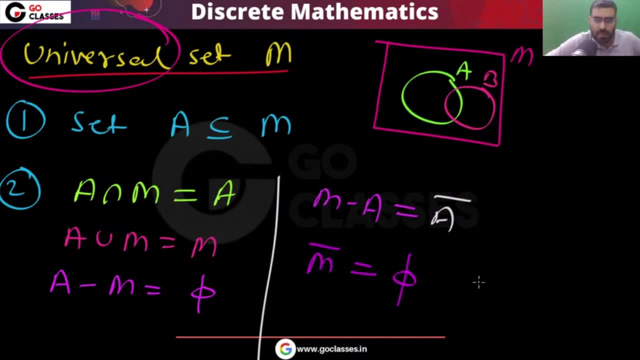 that will be phi, Because universal set complement, that will be phi, And what is phi complement? that will be universal set. So these are the some rules related to the universal set. Very simple, you can easily see. These are the rules, remember, related to the universal set. these are the rules. 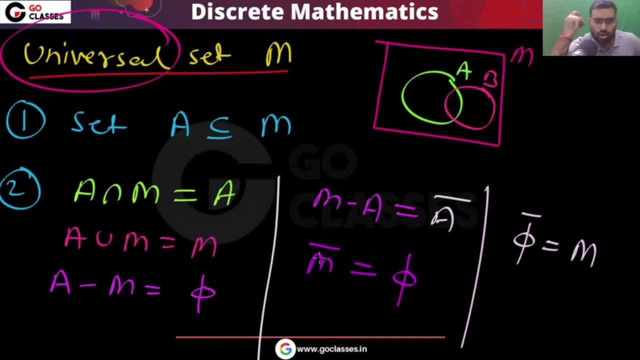 So if you do universal set complement, because universal set contains every element, So universal set complement will be phi And phi complement will be universal set. so these are the some rules, some more rules. you can see that if you do symmetric difference with m, so that will be m minus a, because a minus m that is phi. okay, so exclusive. or if you do: 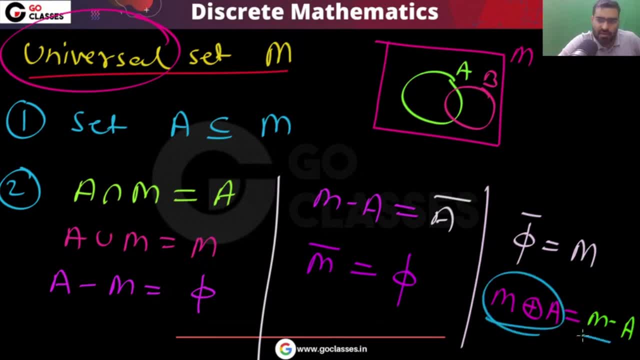 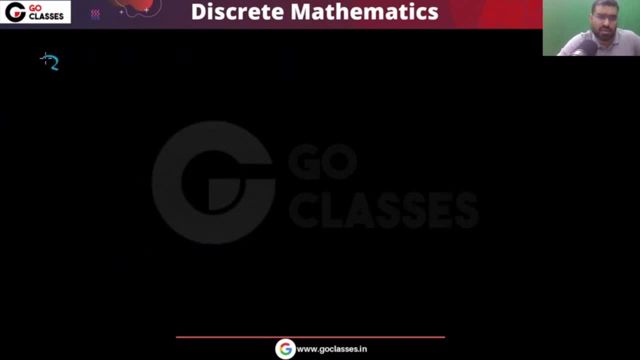 symmetric difference. if you do, then the exclusive elements are m minus a. these are the exclusive elements. now let's see some more rules. the second, the. the third rule. you can notice this associativity, this union, comma, intersection are associative. these are associative. what are what this associativity? 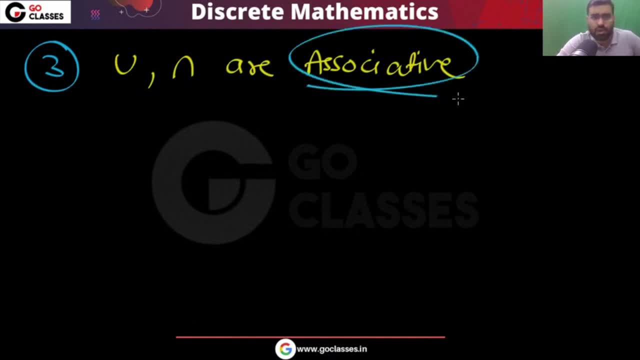 means associativity simply means that if you have three set, if you have a, b, c and you do their union, then okay, you have three set, a, b, c, you do their union. then it simply means that whether you do the union first, like this, or whether you do like this, they are same and we can simply say that: a 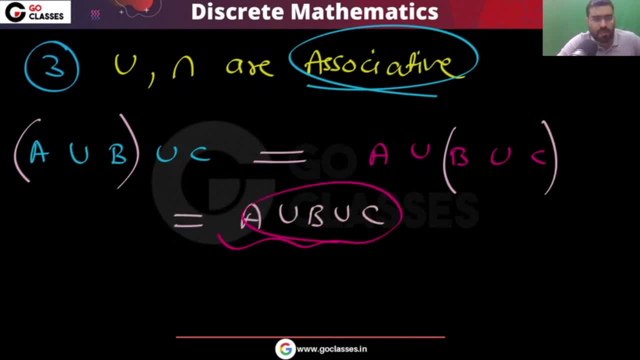 union is associative and a b c is associative and a b c is associative and a b c is associative. b union c means take all the elements of a comma b, comma c. okay, take all the elements. so very simple. similarly you can notice if you do intersection, if you have three a, three set and you do intersection. 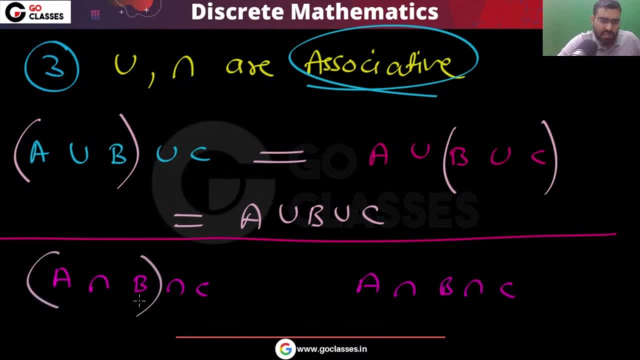 then you can see that whether you do the intersection of this a comma b fast and then you do intersection with c, or you do intersection of b comma c, then you do intersection with a, these are basically same and finally we will write it as a intersection b. intersection c means take: 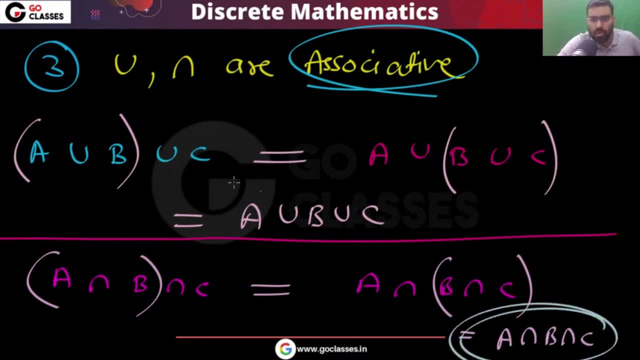 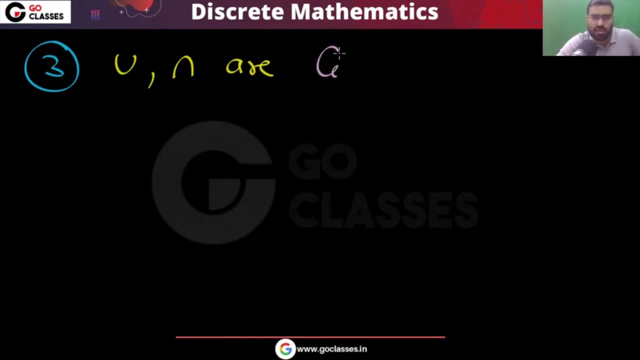 all the common elements of all the three. okay, common elements of all the three. so these are associative. next, you can see that they are commutative. okay, they are commutative. they are commutative. what it means: that if you do a union b, or whether you do b union a, these 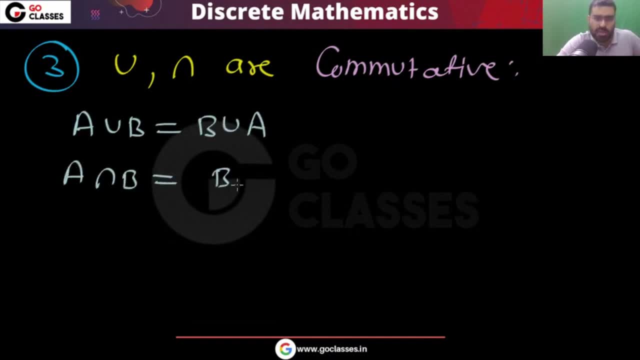 are same. if you do a intersection b, or you do b intersection a, they are same. okay, so these are important. what else are commutative? what else is a commutative? what other things are commutative? so let's say first of all, you tell me what? 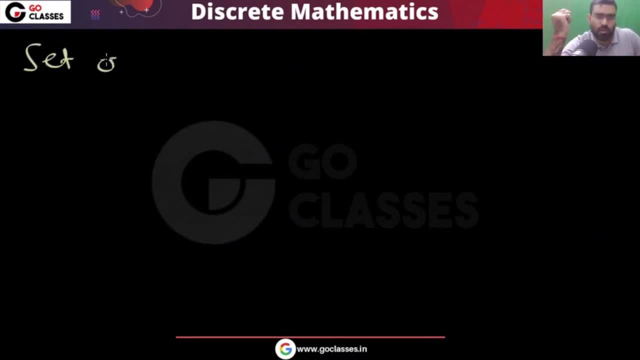 other things are commutative with set operations that are commutative, set operations, set operations which are commutative, sorry, set operations, associativity, whether they are associative or not, set operations that are associative or not. so some options. i'm giving you the first option. i'm giving you union. the second option: intersection. the third option i'm giving you. 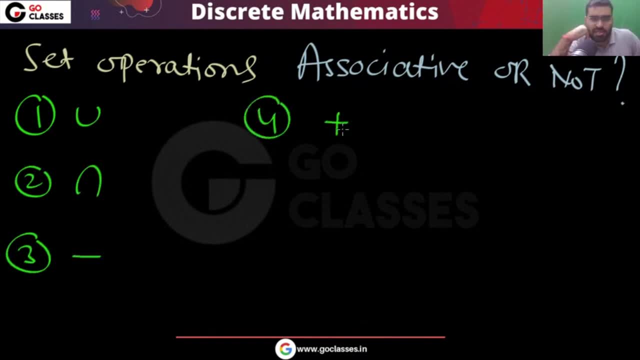 set difference. fourth option: i'm giving you symmetric difference. so these are the some options i'm giving you. tell me, are they associative or not? four options on your screen: which of them are associative, which of them are associative? so tell me, you can notice, union is associative, intersection is associative. 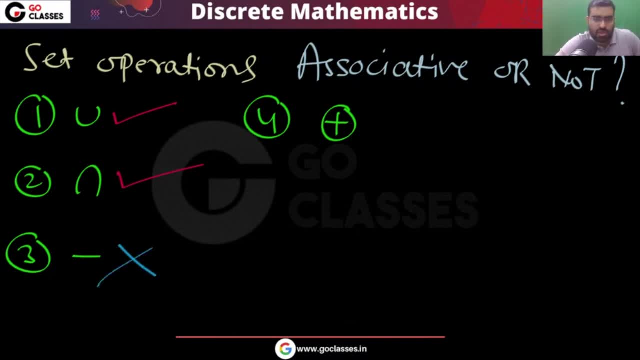 symmetric difference is not associative. and sorry, this is set difference. set difference is not associative. symmetric difference is associative. okay, this symmetric difference, this is a associative. so you can easily see that this, uh the proof i will not give you. if you, if you are interested in the proof, if you want to know the proof, then you can study the discrete mathematics course. 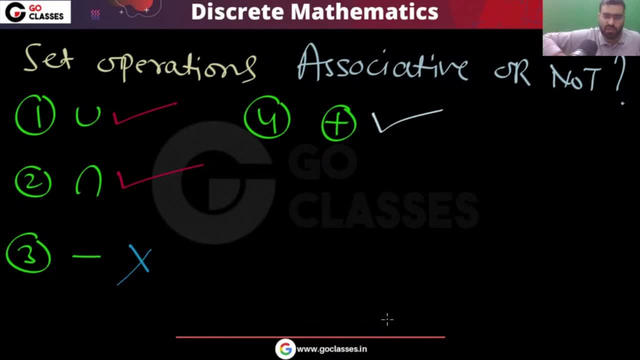 from the go classes website. complete discrete mathematics course is freely available for all the students on the go classes website. so if you want to study the proof, okay, i will not go into the proof, but if you want to study the proof of everything- why symmetric difference is associative- 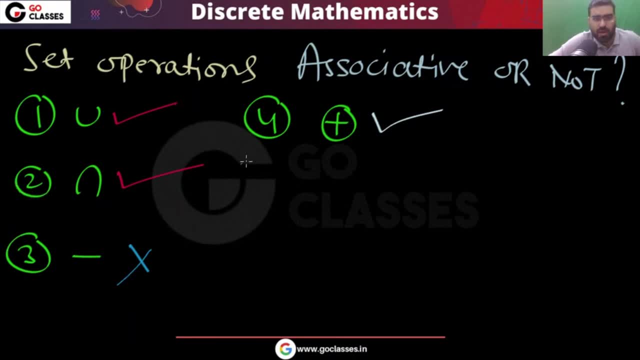 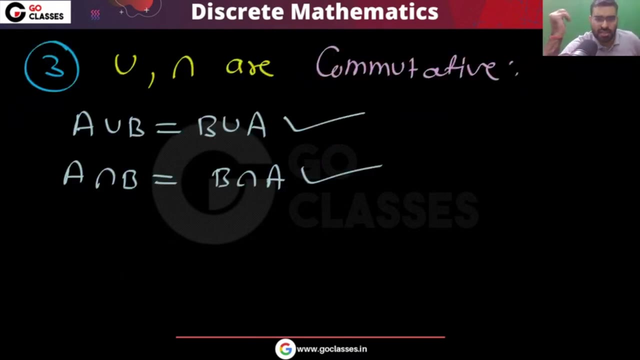 y set difference is not associative. why these are associative? okay, if you want to study the proof of every factor, then you can study the discrete mathematics course from the go classes website. so, anyway, so this. this is the point. now let's see the commutative. so what other operations are commutative? let me tell you these. 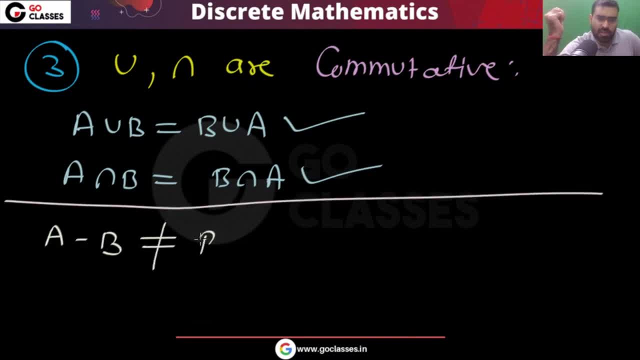 are commutative. now, a minus b, it may not be same as b minus a. they may or may not be different. a minus b may not be same as b minus a. okay, the next point is: symmetric difference is commutative. so if you have a symmetric difference b, that is same as b, symmetric difference a, so that is. 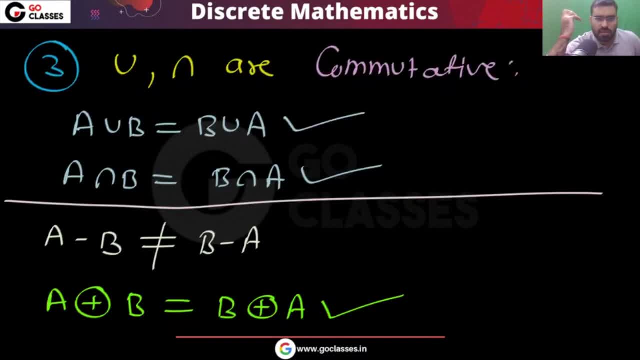 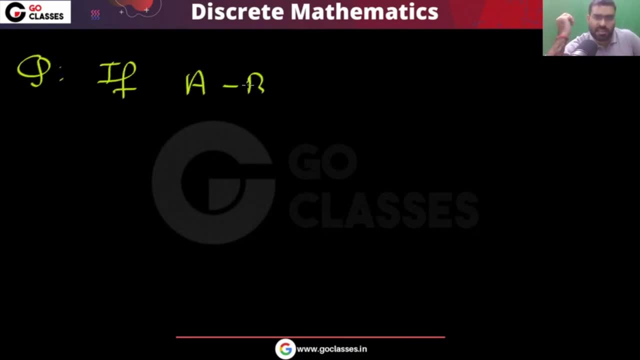 commutative. okay, simple. now some questions. i want to ask you. okay, tell me, if a minus b is same as b minus a, if this a minus b, this is same as b minus a, then what can you say about a comma b? then what can you say about a comma b? what will happen? tell me? can anyone tell me if a minus b? 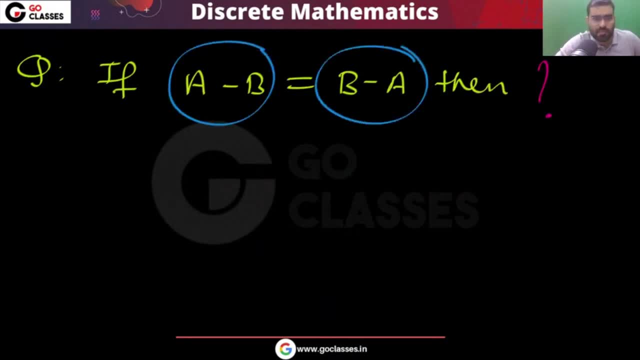 is same as b minus a. this, a minus b, that is same as b minus a. these are exactly same. then what, what? what can you say? what can you say that? what will happen? the elements which are only in a and these are the elements which are only in b, c understand very simple. these are the elements which are only 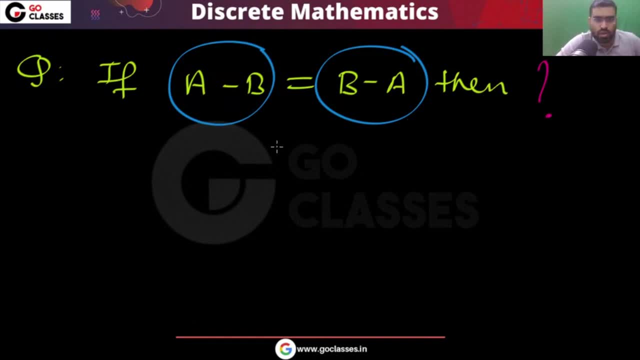 in a. these are the elements which are only in b. so if a minus b is b, b minus a, can i say: ava, A definitely will be equal to B. Can I say, can I say, in this situation, A definitely will be equal to B. 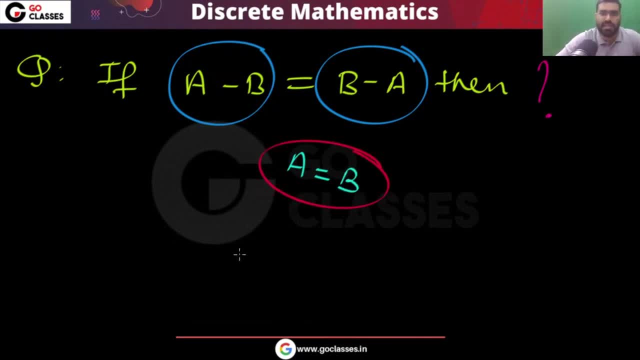 Can I say this? Tell me, can I say: A will definitely be equal to B, A will definitely be equal to B. The answer is yes, OK. So in this situation, if A, ah, then the answer will be this: OK. 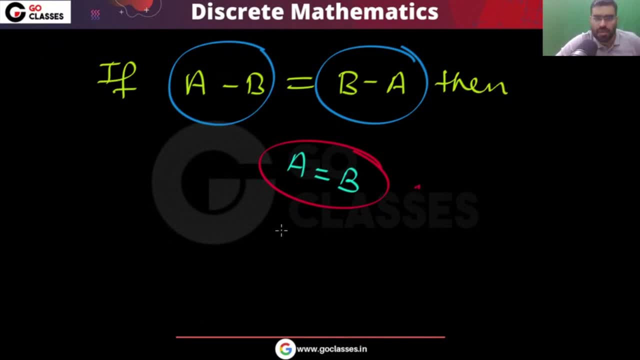 So you can easily see: definitely a will be equal to B. Why, what is the reason the? The reason you can easily see that, if you can easily see that if A is not equal to B, if A is not equal to B, if this happens, okay, then this will have those elements, which are: 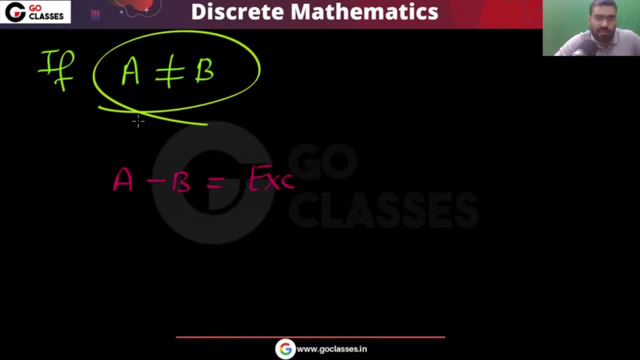 exclusive of A, which are exclusive elements in A right, These will have those elements which are exclusive in A and these will have those elements which are exclusive in B. So, of course, if they are not same, if these two set are not same, 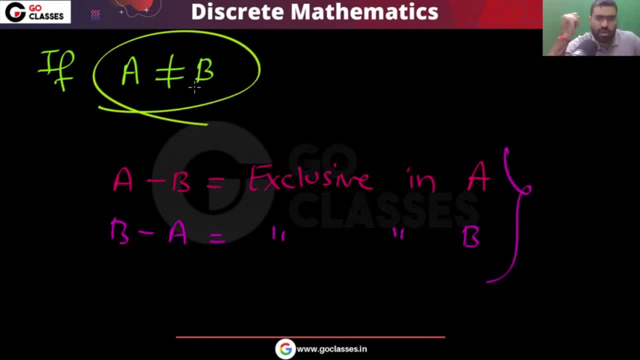 then definitely some exclusive element will be either in a or in B. Okay, So, in this situation, definitely these two cannot be same. Okay, So if this happens, then they cannot be same. They cannot be same, Right? Okay, Are you getting my point? If a is not equal to B, 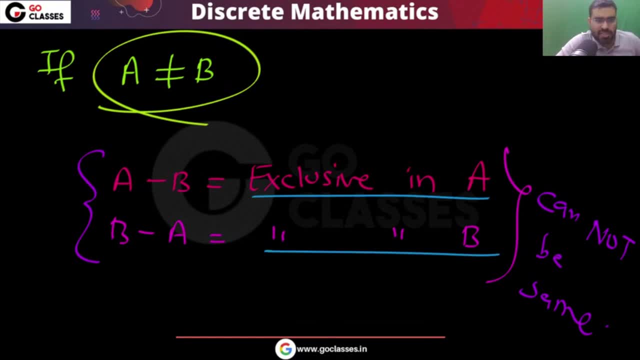 then these exclusive elements? these exclusive elements, they cannot be same because they are different. A is different from B. It means there is at least one exclusive element. Are you getting my point? Simple question of simple thing. I'm saying that. I'm saying that if 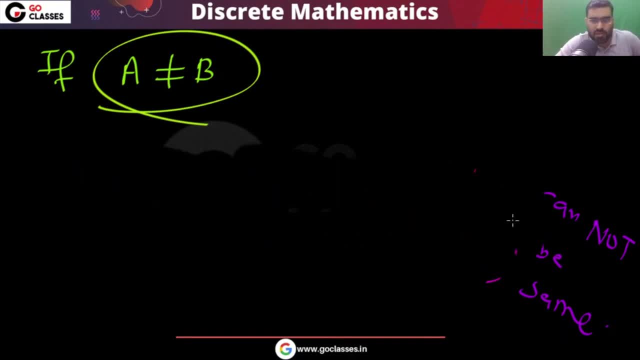 a is not equal to B, then there will be at least one exclusive element. Okay, In this situation, if a is not equal to B, then there will be at least one exclusive element. I can say: this will not be known. This will not be empty. There will be at least one exclusive. 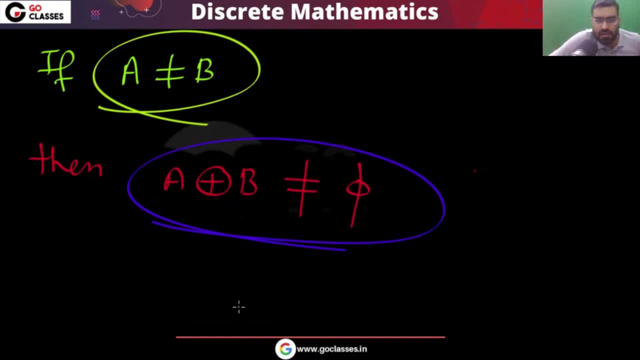 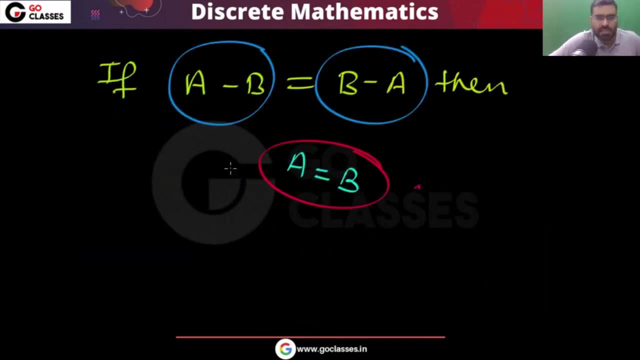 element. So you can easily see that. Uh, I can say so, these two will definitely be different. Okay, Let's move on. So you can see that this will happen and the and converse will also be true, and converse is also true. 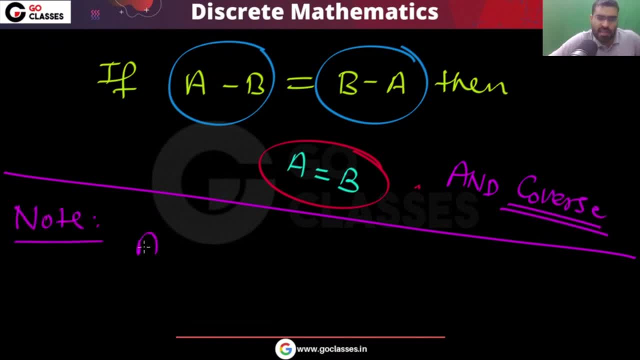 So this statement, I can say what I can say. I can say that a is equal to b if and only if, if and only if a minus b is equal to b minus a. Okay, I can say: a is equal to b if, and only if, a minus b is equal to b minus a. 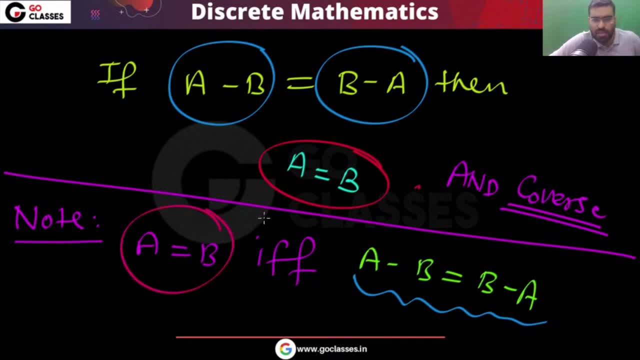 So this statement: we can say a minus a equal to b, if and only if so. if a is not equal to b, I can also say that if a is not equal to b, then a minus b is not equal to b minus a. a minus b. a is not equal to b, if, and only if, they are not different. 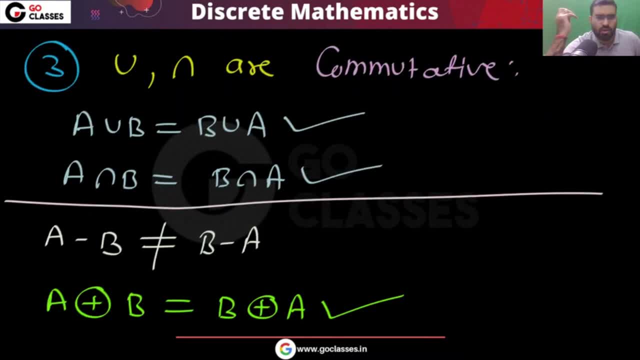 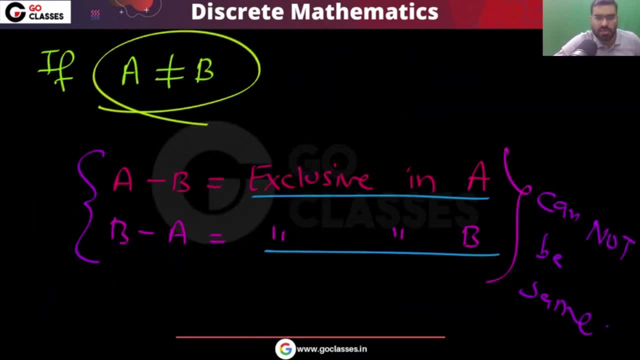 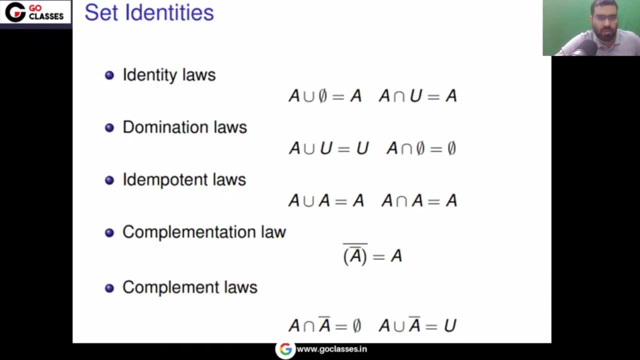 Okay, now let's see this. so here you can notice that symmetric, symmetric difference is commutative, but set difference is not commutative. Okay, this is one thing you can see. what is the next? So this, Some properties as we have seen. now let's see some more properties that, if you do, 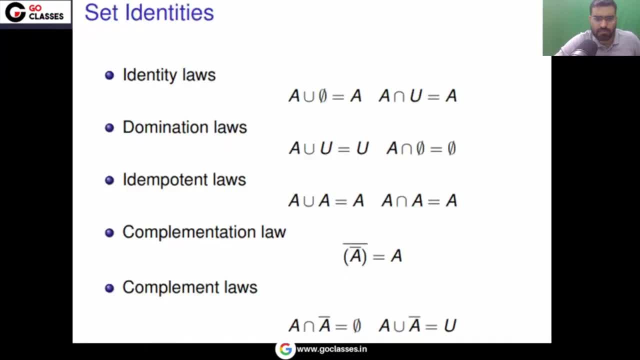 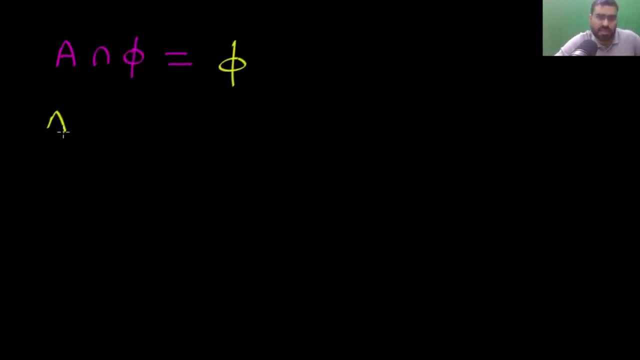 Yeah, OK, so some more properties. let's see Some more properties. if you do intersection with the file, if you do intersection with the empty set, then you will get empty set. if you do union with the file, then you will get a itself. If you remove empty set, then you will get a itself, because I'm removing empty set means you did not remove anything. 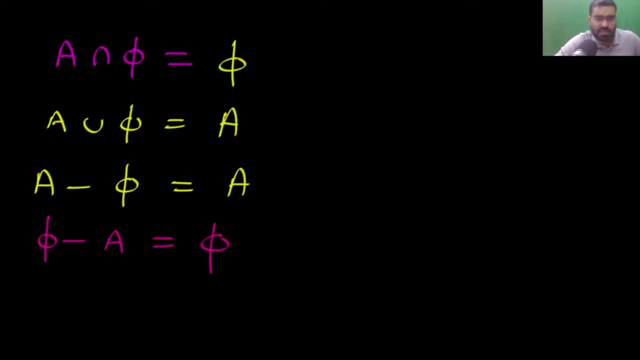 And if from empty set, if you remove set, then it will be empty. Okay, because the complete set you are removing. next, if you do symmetric difference with empty set, if you do symmetric difference with the empty set, that will be itself, because, because five is a subset of a. 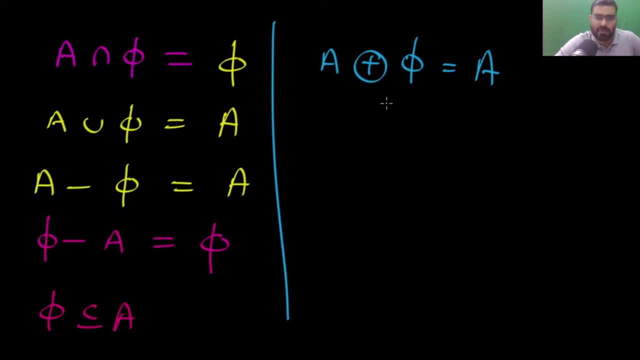 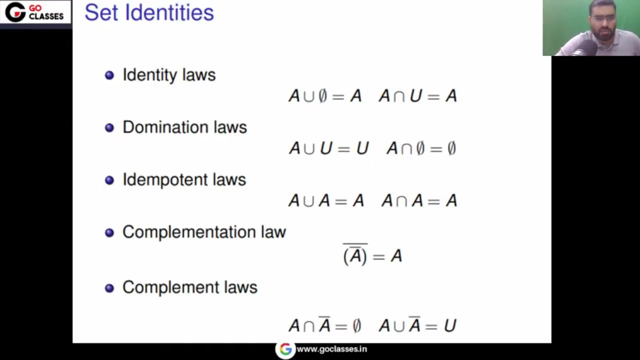 Okay. so that is the reason: the symmetric difference will be itself. so these things you can easily see And you already know that five compliments, five compliments that will be universal set, Okay, Okay. so these points you can see. now the next point also, I want to tell you that if 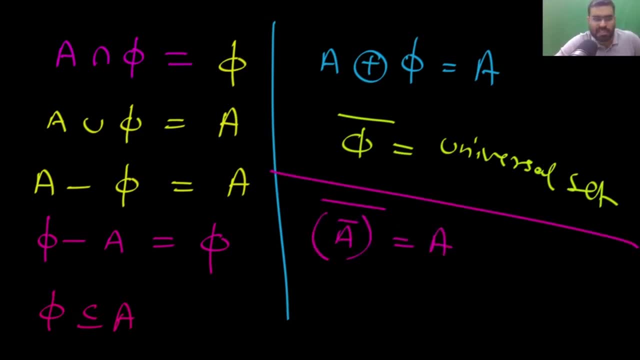 you do a complement, then you do again complement, then that will be same as a. this is called double complementation rule. and also, if you do a union a, that will not change anything. if you do a intersection a, that will not change anything but what is a minus a. so you can. 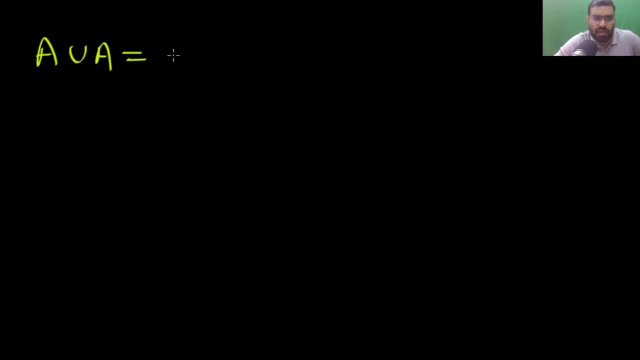 notice: a union, a. all the elements of a. all the elements of a. so that is all the elements of a intersection: a. all the common elements of a comma a, that is a. if you do a minus a, that will be five. if you do symmetric difference of a comma a, that also will be five, because 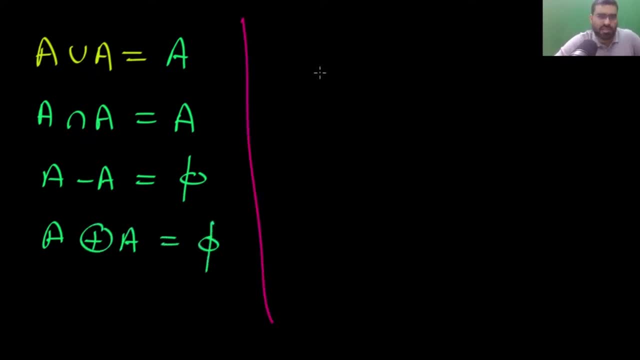 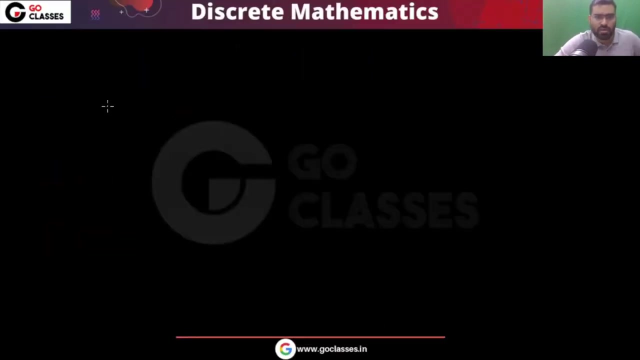 there is no exclusive element. okay, so very simple, these points. so all these points, I think we have seen double complementation rule and, yeah, also, if you do a intersection, a complement, remember they are designed okay. so they are simple. a simple question I am asking: Can I say that they are designed? 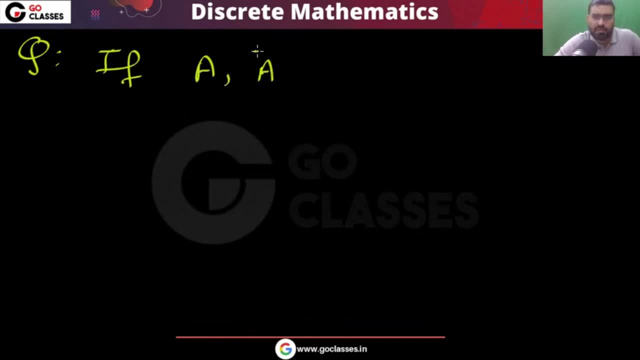 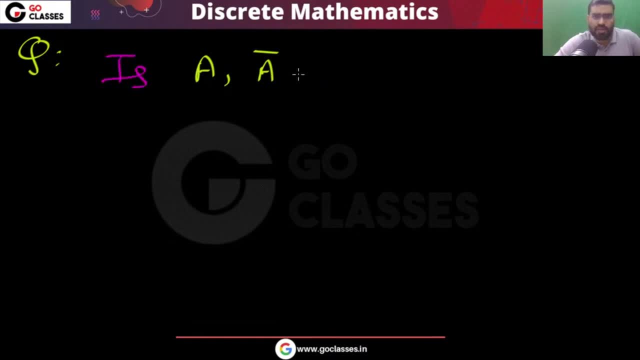 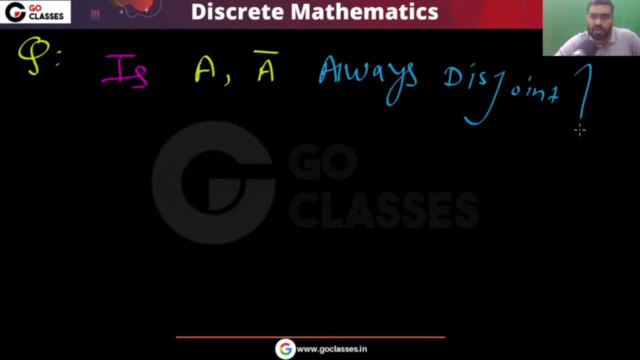 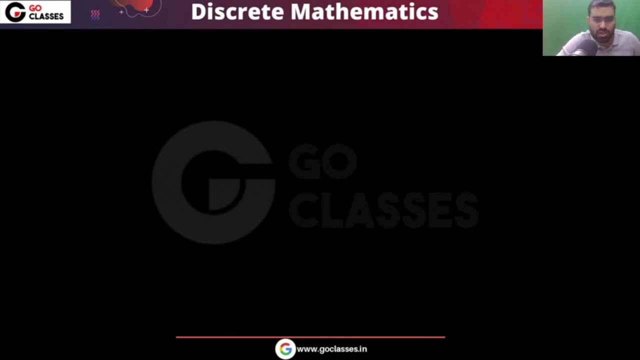 always be designed. can i say: can i guarantee that they will always be designed? can i guarantee they will always be designed? the answer is yes, because a intersection, a complement, will be phi. so they will always be designed, even if not, even if you take a equal to phi, if you take a equal to phi. 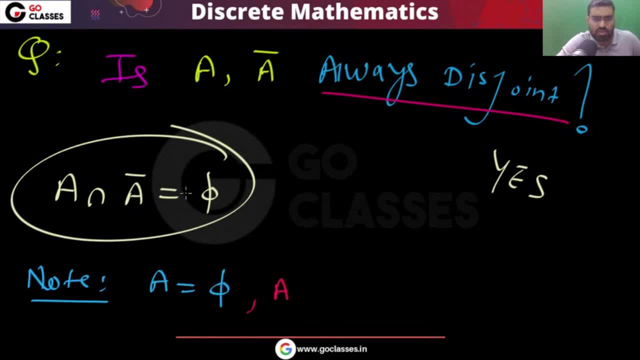 then also no problem. okay, then also in this situation, if you take a equal to phi and let's assume your universal set, uh, like, whatever you do, basically your a complement will be m minus a, where m is universal set. so whatever you do, they will always be. 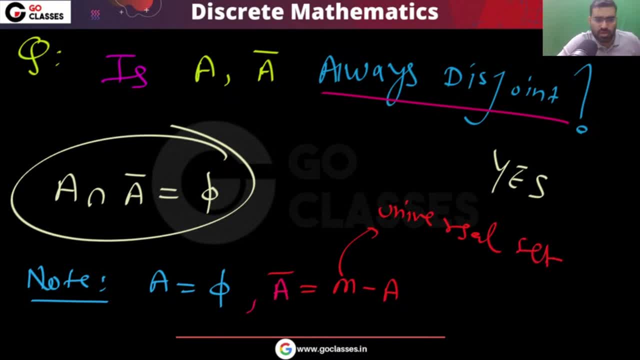 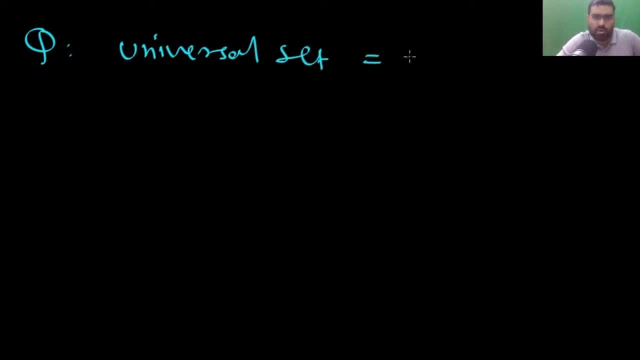 they will always be designed. now, for example, a question i am asking: let's assume universal set is also phi. let's assume universal set is also phi and your set is also phi. then can i say a, a complement, are they designed you? are they designed? tell me, if your universal set is also phi and your a is also phi, can i say they? 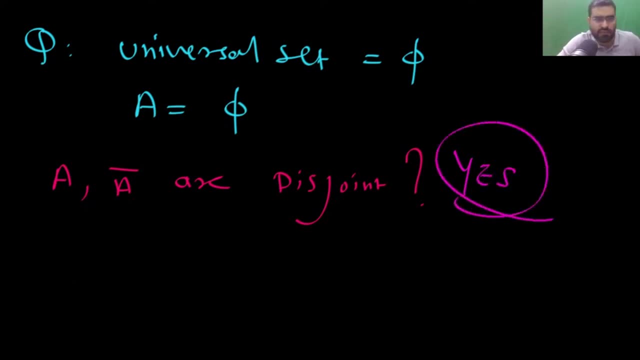 are designed. the answer again is yes. just use the definition of designed, because you can notice, in this situation, a is also phi, in this situation, a complement is also phi and you can see their intersection is phi. so they are designed. okay, so they are designed. so remember, just apply the. 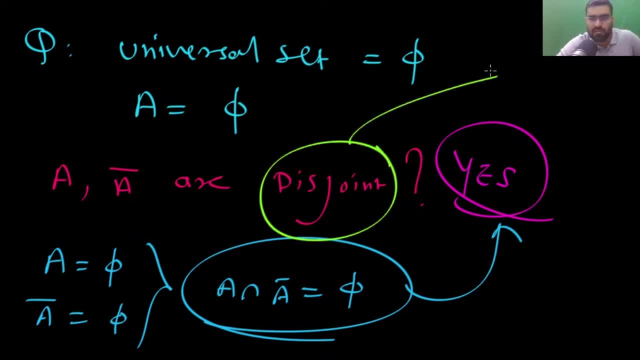 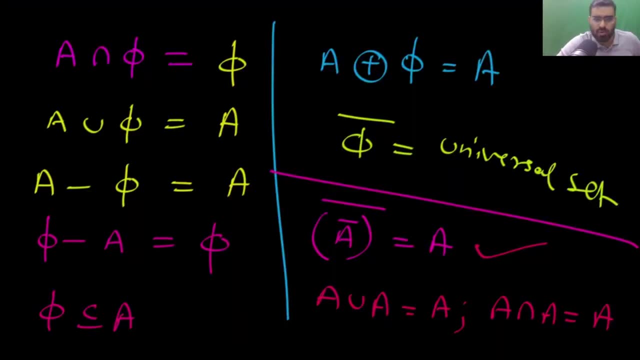 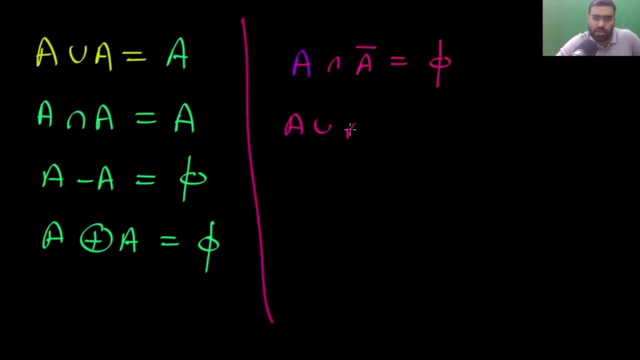 definition of designed. designed means when can i say? two things are designed when their intersection is phi. in this situation, you will say: they are designed. okay, let's move on. so you can easily see that if you have a intersection, a complement, that will be phi. if you take a union, a complement that 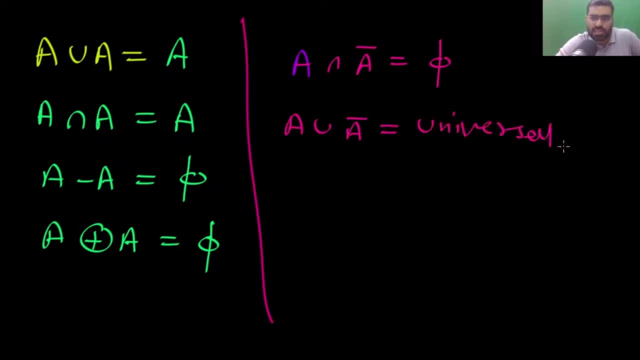 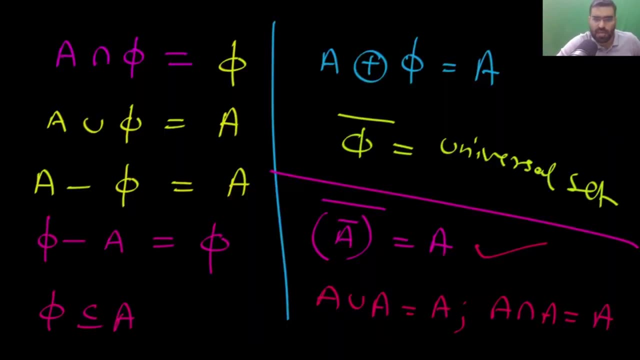 will be universal set. okay, that will be universal set because all the elements you will get a union, a complement. it will give you all the elements. okay, so all these properties we have already seen. arnab is asking a comma, a complement. what is their intersection? see arnab, look at this. 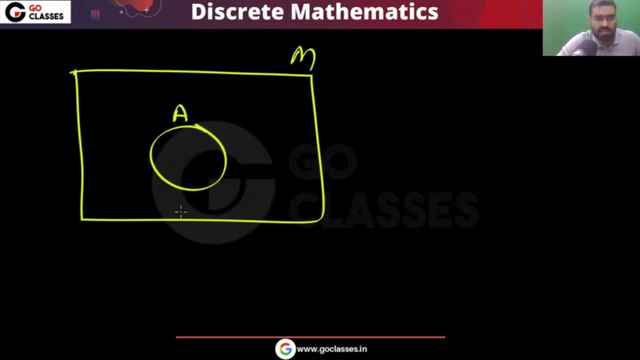 this is your universal set, this is your set a. then this is your a complement, right see, look at this. this is the area of a complement and this is the area of a. tell me what is a intersection, a complement. tell me what is the common, what is common. tell me what is the common, this, this out. 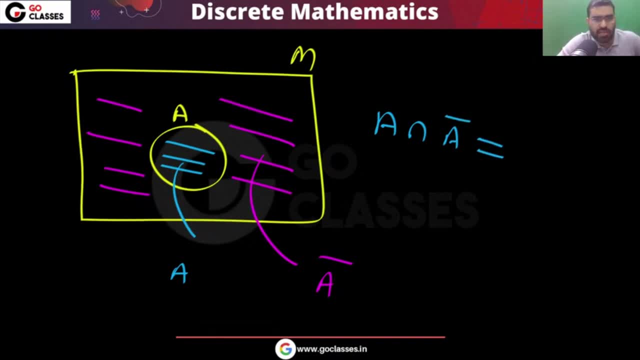 this is the area of a complement. what, what is not in a, that is a complement. what is not in a complement, that is a. so what is the common area? the common area is phi, and you can notice a union, a complement that is universal set. Okay, so very easy. 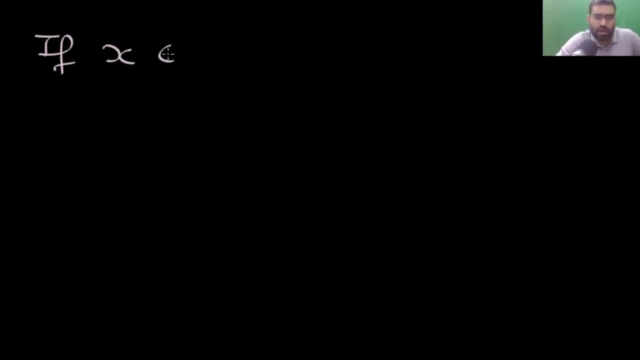 You can easily see that if x belongs to a, if x belongs to a, then x does not belong to a complement, Right? Similarly, if x belongs to a complement, then x does not belong to a. Similarly, if x belongs, if x does not belong. 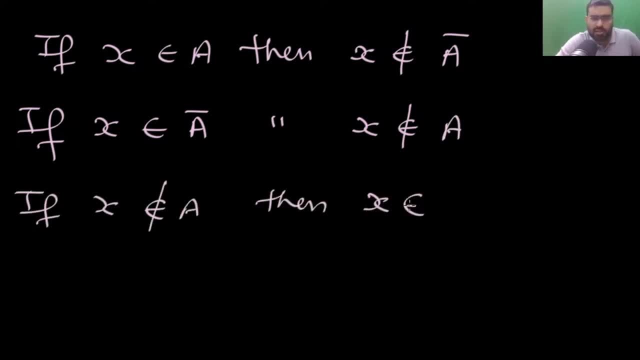 to a complement. sorry, a x does not belong to a, then x belongs to a complement. And if x does not belong to a complement, then definitely it will belong to a Right. That is the meaning of complement. This is the meaning of complement, Right. 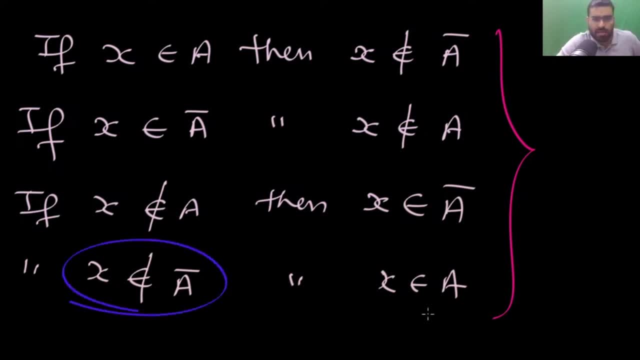 So you can easily see that if x does not belong to a complement, then definitely it will belong to a. Okay, if x does not belong to, if x belongs to a, it will. also it will not belong to a complement. So very simple Like this. this is the. 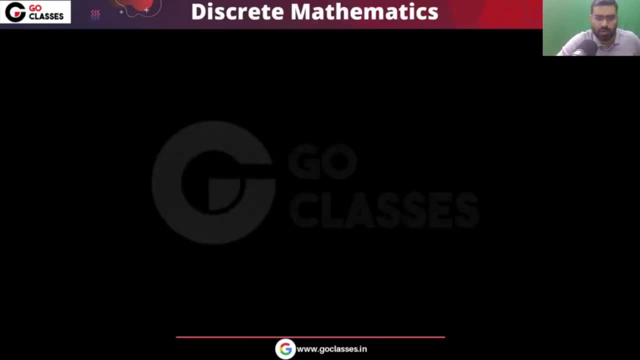 definition of complement. Now let's see the next. that is distributive law. So union is distributive, Union is distributive over intersection, Union is distributive over intersection And intersection is distributive over union. This intersection, this is distributive. 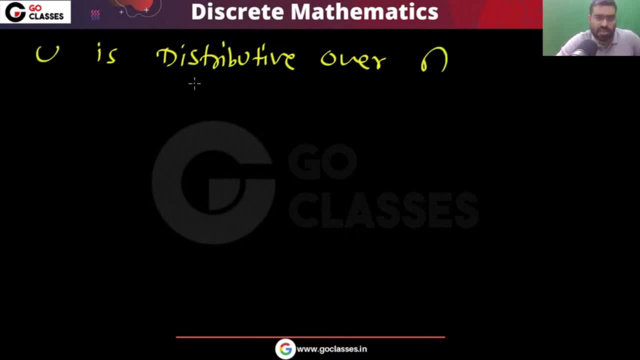 over union. So what this means: Union is distributive over intersection. It means, if you do union over intersection, Union over intersection, then what you will get: This union is distributed over intersection. This is distributed, You can distribute this union. 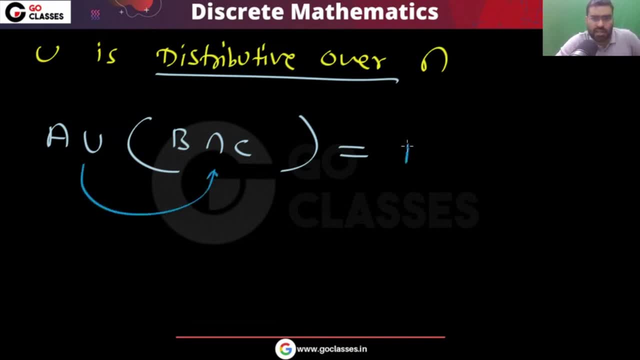 over intersection. So what you can write? you can write that a union B intersection a union C. Okay, So this is true, means union is distributed over intersection. It simply means that a union B intersection C, that is equal to a union B intersection, Sorry, a. 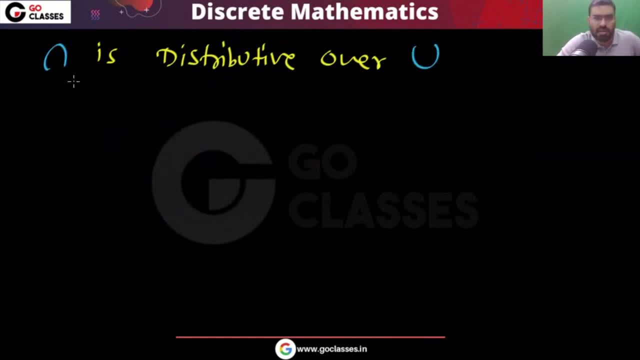 union B intersection, intersection a- union C. Similarly, intersection is distributed over union. so this intersection- this is distributive over union- means it will be a intersection b, union a, intersection c. again, i am not giving the proof. if you want the proof, if you, if you want to understand the proof, you can prove it. okay, you don't have to buy heart. 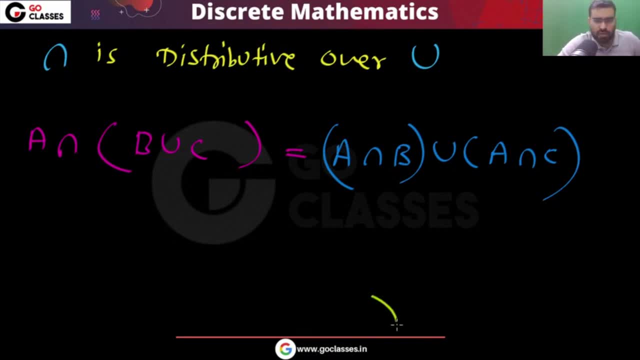 anything, you can prove everything. if you want to study the proof, then you can watch the go classes discrete mathematics course, in which everything, every statement, every theorem, every concept, every formula is taught with proof. so in the go classes discrete mathematics course, you will never buy heart anything. everything that you will study, you will study with proof. so this: 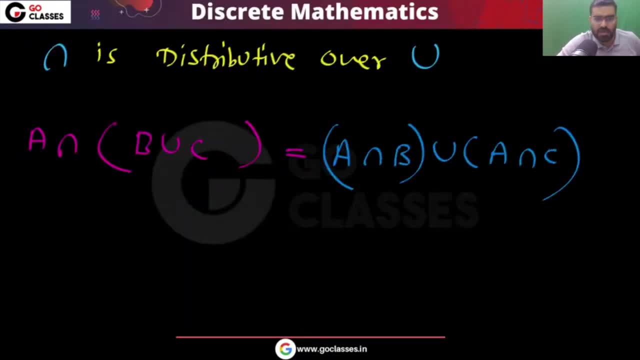 is the distributive property. now let's see d morgan property and absorption properties. this is, these are some important rules. okay, very important rules, very important rules. the first rule is d. morgan law means if you do a, intersection b and then you do the complement, that will be same as a complement union. 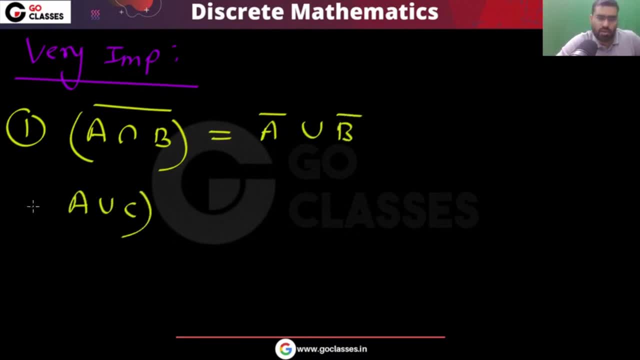 b complement. also, if you do a union b, then you do the complement, then that will be a complement, intersection, c complement. okay, so like this: this is the d morgan law means d morgan law says that if you do the complement of intersection, then what will happen? it will happen: union of complement of. 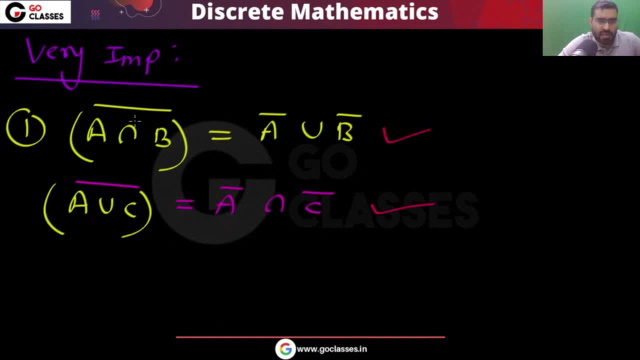 the set like a intersection, b, complement, that will be, this intersection will become union and this a will become a complement, b will become b complement. and if you have a union c Complement, that will be A complement, intersection, C, complement. Also, this is called absorption law. 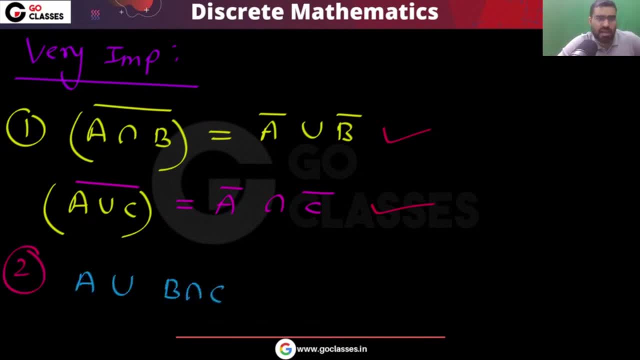 That if you do A union A intersection B, If you do this, Then that will be same as A. See, you can prove it, This absorption law, actually, you can easily prove if you forget A union A intersection B. So how can you prove it? 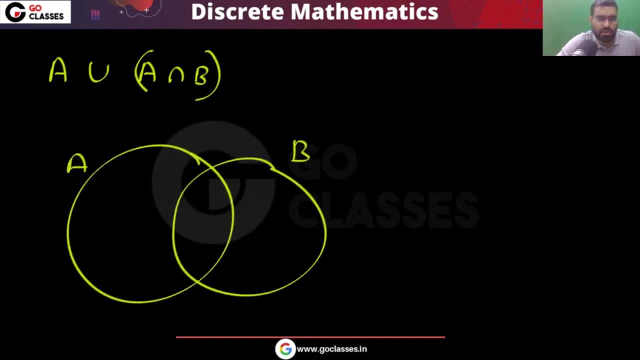 You can easily say that if this is A, If this is B, Then you can notice: what is this A intersection, This is A intersection B, This is A intersection B. Now you tell me what is A union, A intersection B? Please tell me quickly. 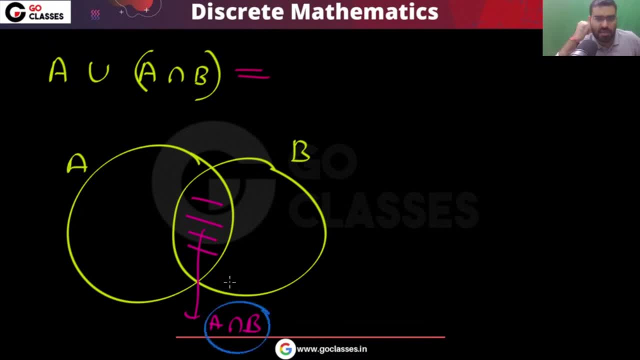 If this is A, this is B, Then this is A intersection B. Now you tell me, what is A union A intersection B? A union A intersection B, that is same as A Right. So very easily you can do Now the same thing. I can ask you: 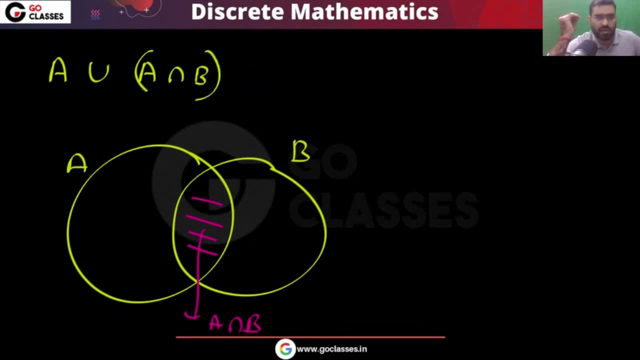 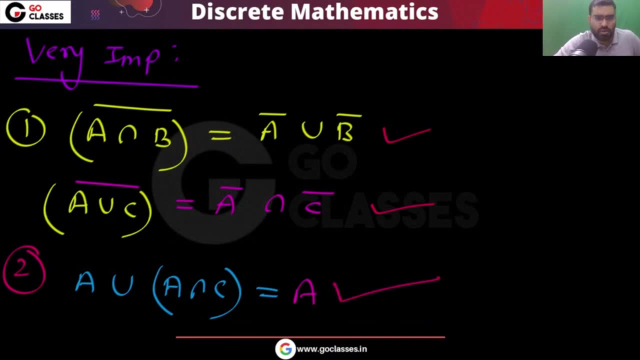 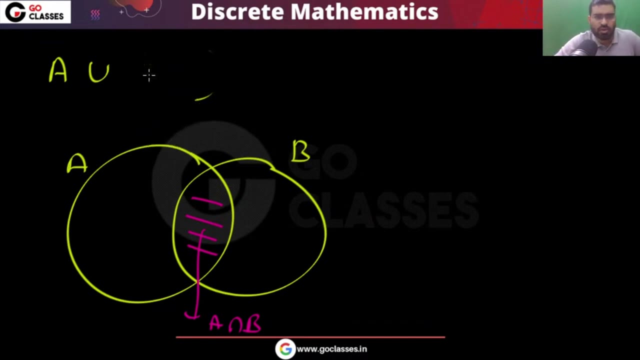 You tell me, if I ask you, A union A complement intersection B, Okay, so something. So this is interesting. like A union A, intersection C, That is A. Similarly, you can do Another question I am asking you, And that question is something like this: 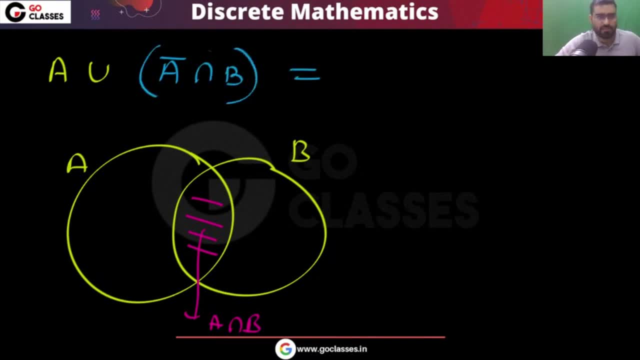 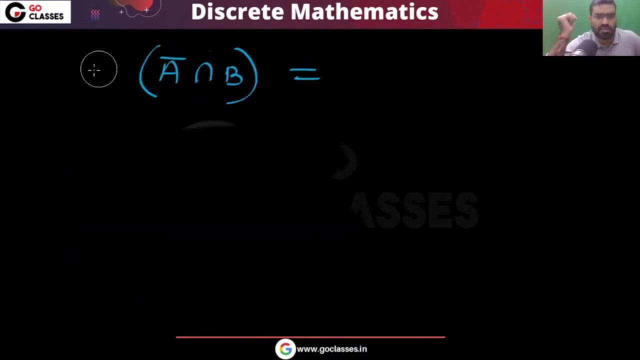 A union A complement, intersection B. Now, what is that? Okay, did you understand the question I am asking: A union, A union Before that. actually, Before we see this, Let's see what is this one Like. what is this? A intersection B, complement. 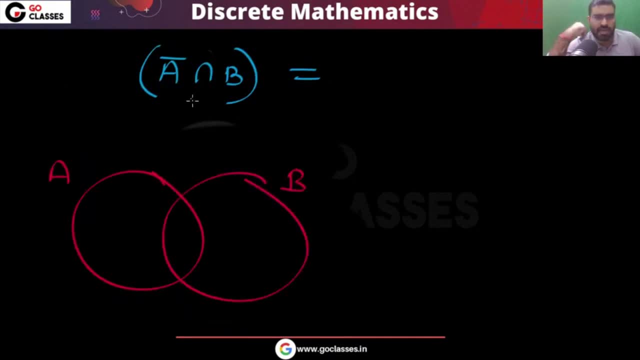 So if this is A, This is B, Then what is A complement intersection B? It simply means A complement, This is your, This is your A complement. A complement means this: This area is the A complement Intersection B Common part. 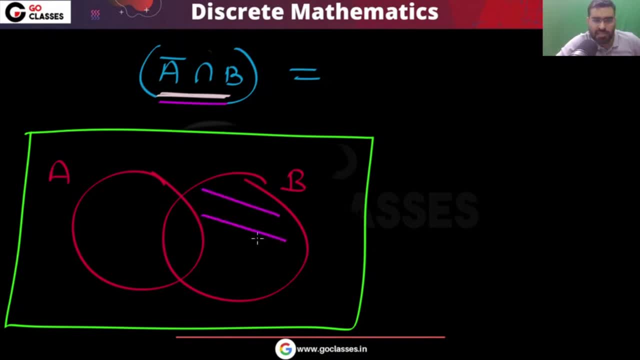 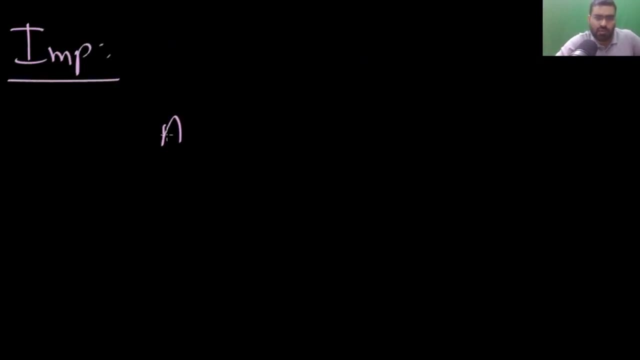 Intersection means common part. Common part in B comma A intersection. Common part in B comma A intersection. your b in b: this is b intersection, a complement, so that is same as b minus a. so this is a important point actually. okay, this is a very important point that if you have a minus b, 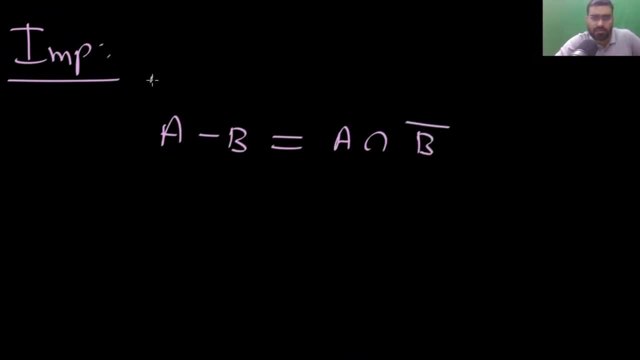 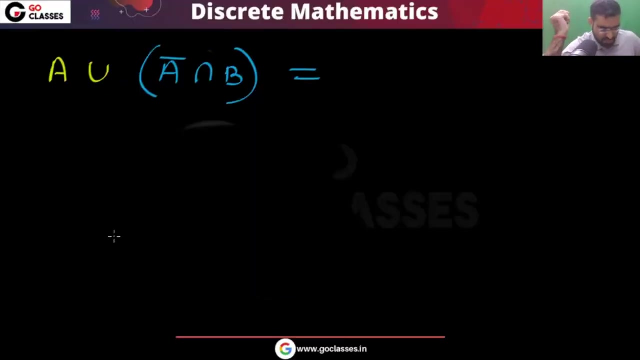 you can write it: a intersection b complement. okay, if you have b minus a, you can write it b intersection a complement. so this is a important point now. let's see this. now tell me the answer for this one. can you tell me the answer for this one? a union, a complement, intersection b. 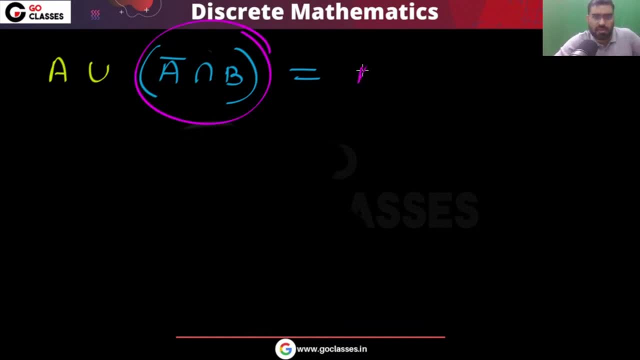 we already know that this is same, as we already know, this is same as b minus a. so this is set a, this is set b. then what is a union? b minus a? remember, this is b minus a, this is b minus a, and you cannot. this is a, this is a. so what is a union? b minus a? 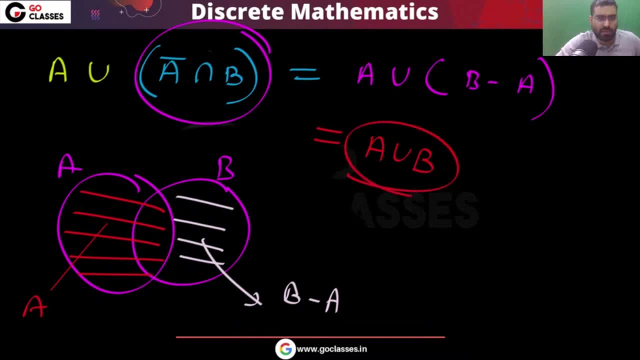 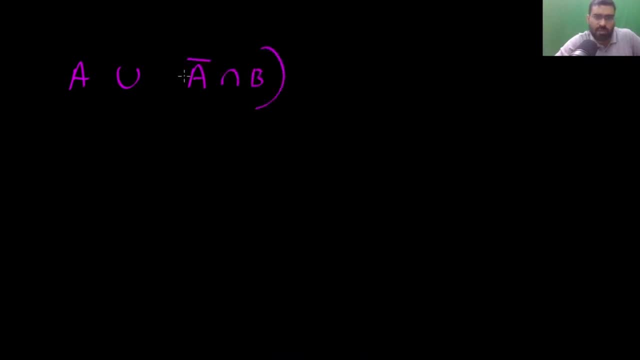 that we will be A union B. okay, that will be A union B, very simple. so this is the point. I want to tell you that A union A complement intersection B. you can easily see that that is same as A union B. actually, this is very similar to the propositional logic if you study in the 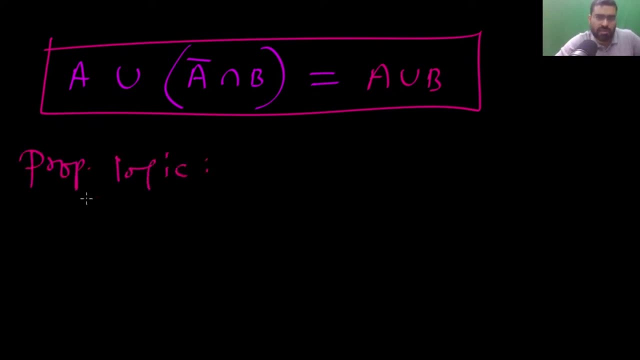 propositional logic. there is a rule in the Boolean algebra in the propositional logic, this is the set. this is the rule in the set theory. now in the propositional logic, similar rule you have where you have like P or P bar Q, that is same as P or Q. very similar rules. 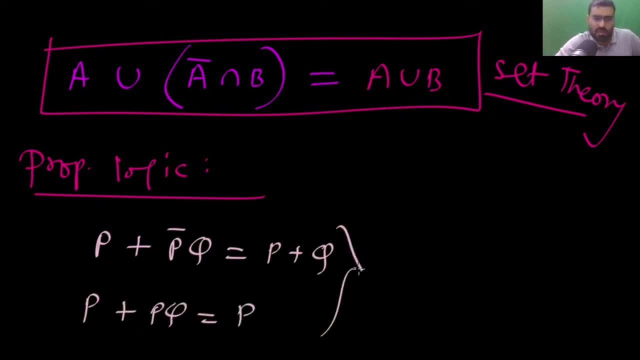 you have like P or PQ, that is same as P. So these are the rules in the propositional logic and these are the rules in the set theory. In the set theory, what will happen? I can see A union. I can see A union, A bar intersection B- that will be same as A union. 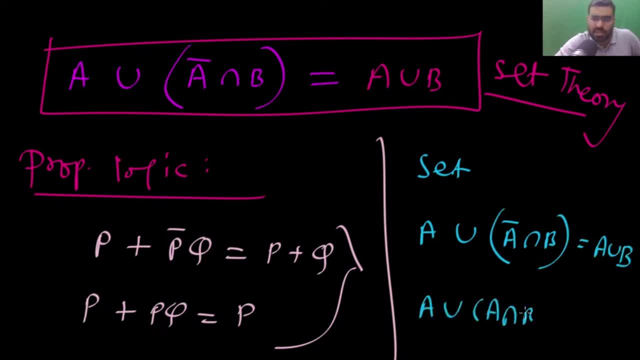 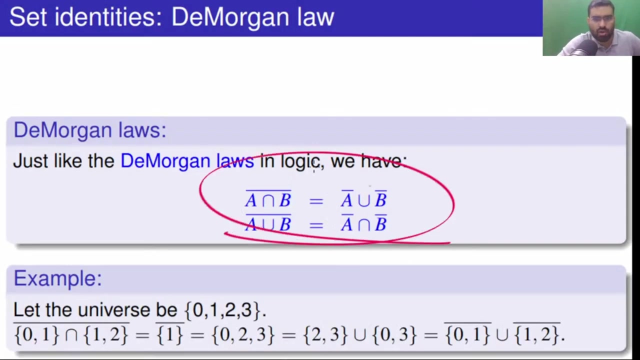 B and similarly A union A, intersection B, that will be same as a. okay, so, like this, all these rules that you have in the propositional logic, similar rules, very similar rules. you have in the set theory also. so all the rules we have seen. i hope you understood this is a d morgan law. you can apply the d morgan law here like you have: 0, 1. 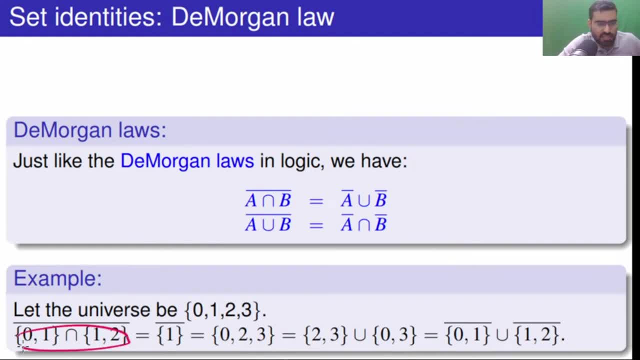 uh, see: 0, 1, intersection 1, 2. the intersection will be: the intersection will be 1, the complement of 1 will be 0 to 3. okay, so like this, anyway, you can check it out. so these all these rules we have seen. 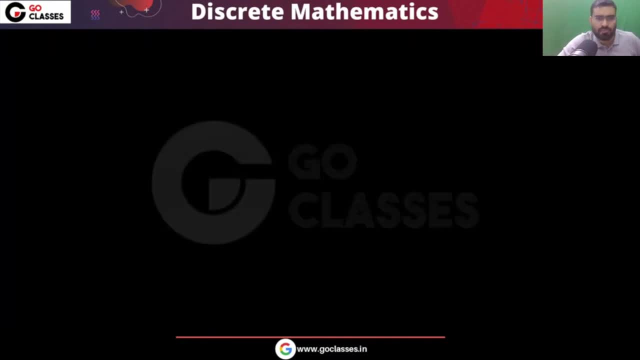 every rule. now let's move on. so, uh, these are important rules. as i told you, a set difference, b. okay, because, uh, this is an important rule. like this is a, this is b, then what will be a? uh, what will be a minus b? this, this is a minus b. you can see, this is a minus b. a minus b is same as 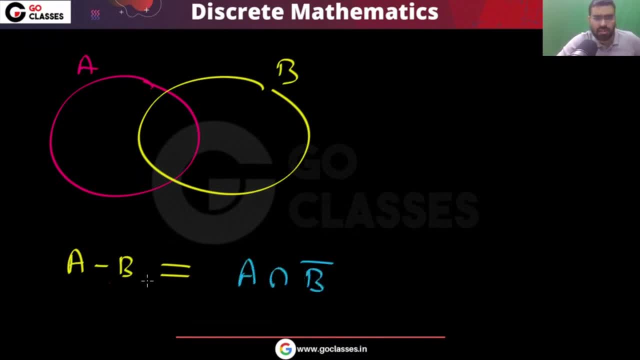 a intersection with b complement. okay, they are basically same, because what is a intersection, b complement? that is common area of a comma, b complement. okay, those elements which are in a and not in b. okay, so you can see, this is the area of a intersection b complement. so this is: 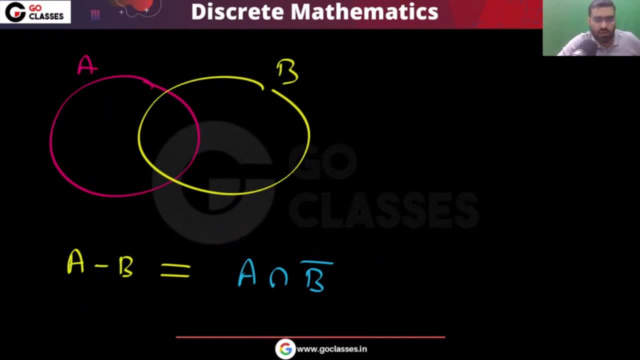 very important rule that this happens. okay, one more thing that happens is if you see the symmetric difference, if you see this symmetric difference. symmetry difference means this area, union, this area. this is the symmetric difference. that means a minus b, union, b minus a. now, that is also same as. 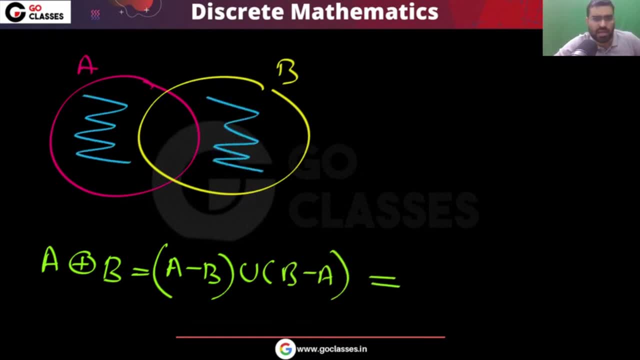 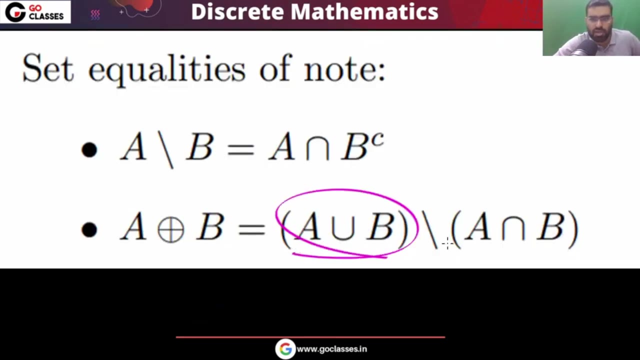 remember. basically, this is your symmetric difference. what i can do. i can say that from the union, you are removing the intersection. right from the union, you are removing the intersection. okay, from the union, you have removed the intersection, so this is the point from the union you are removing. this is the set difference. you are removing the intersection, so this is your. 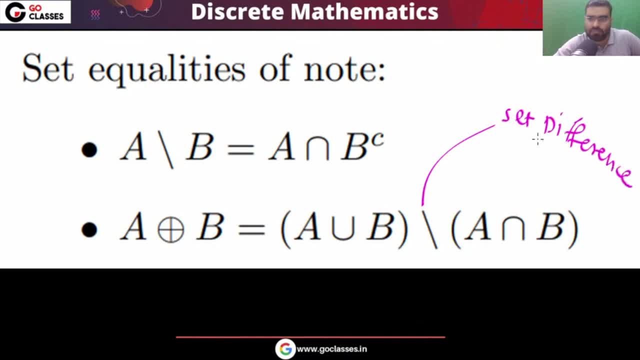 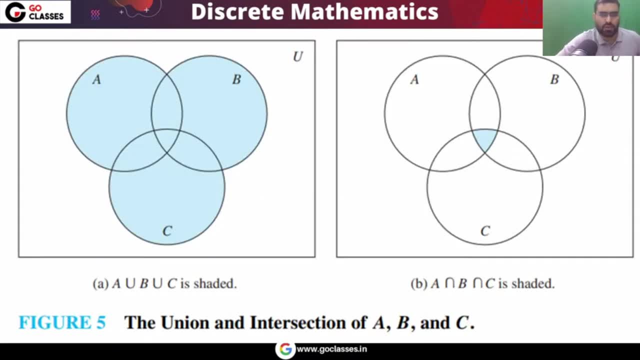 difference. so these are some important rules that we have seen. i hope you understood. and if you have three set, if you have like a, b, c, three set, then also you can create the venn diagram. you can create the venn diagram like this, like this is the union of a comma, b, comma, c. 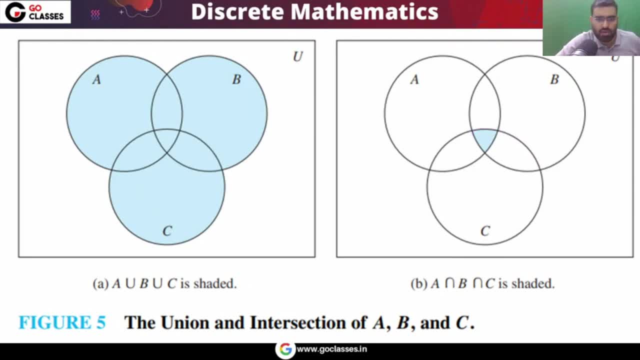 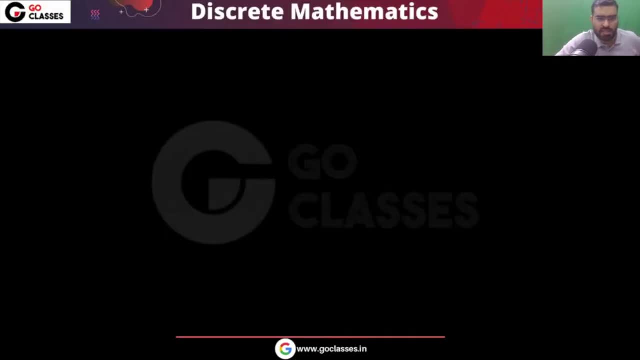 this is the intersection of a, comma b, comma c and so on. so if you have more than three set, then also you can create the venn diagram. so this is the complete revision. this is the complete summary of set theory. so ultimately i want to tell you some. 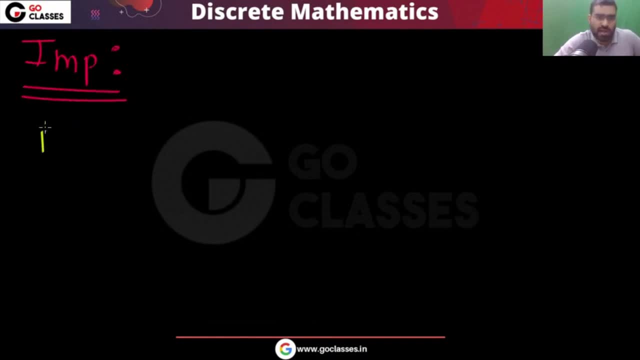 important, some very important, useful rules. as i told you, like a minus b, that is same as a intersection b- complement this rule. you understand the first thing: here a comma b are set. so here set is a comma b. this rule is very important. another rule that is very important is this: a. 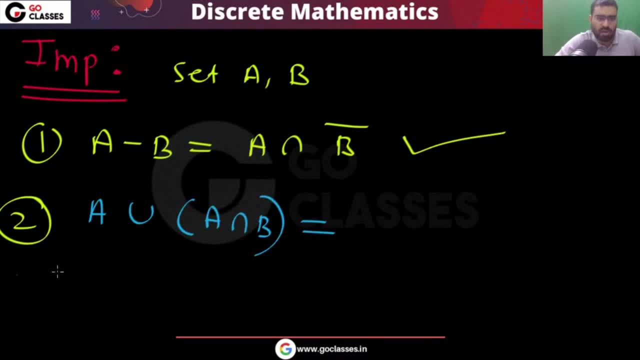 union a intersection b. this is your absorption rule, that is your a. you don't have to buy heart because you can easily, you can easily, uh, prove it okay. so you, there is no need to buy heart. like this is a, this is b, you can easily see that this is a intersection. 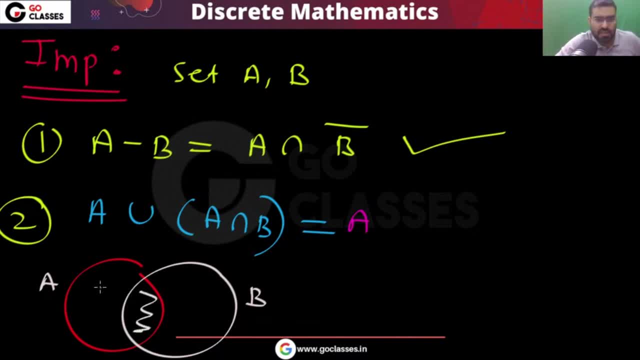 b. okay, so this is a intersection b, union with a. that will be a. so this is the rule. you can see the third rule, that is, a union a, intersection b, a intersection a, complement intersection b, that will be same as a union b. this also you can prove using the venn diagram. 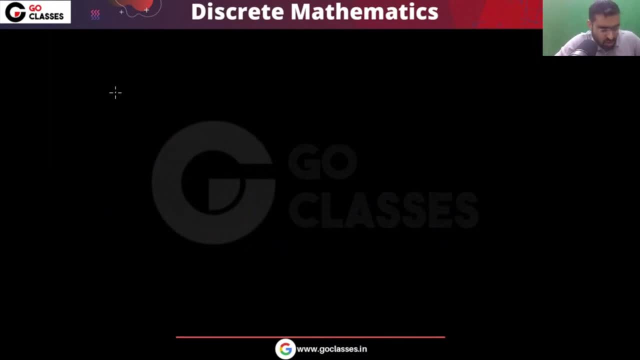 understand that venn diagram is very important. many question you can solve using the venn diagram in the set, in the, whenever you study the set for many questions, okay, for many questions, what you can do for many questions, you can apply the venn diagram. venn diagram is the best and efficient. 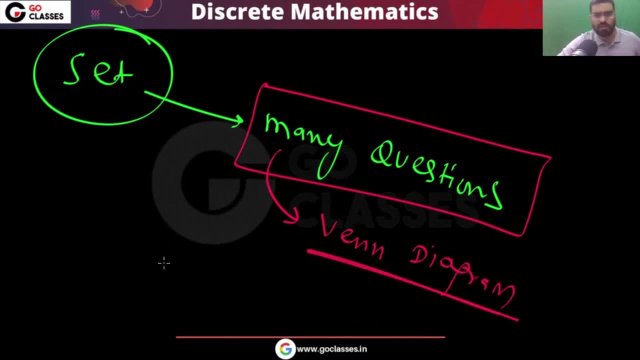 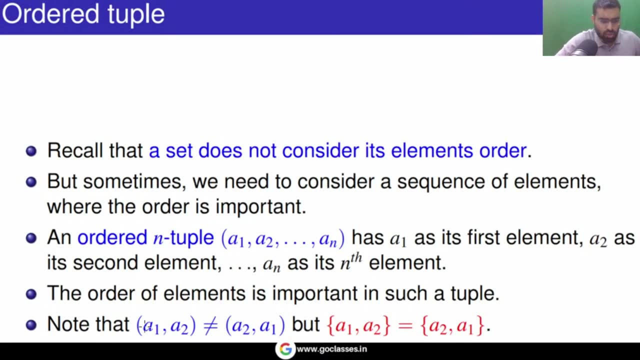 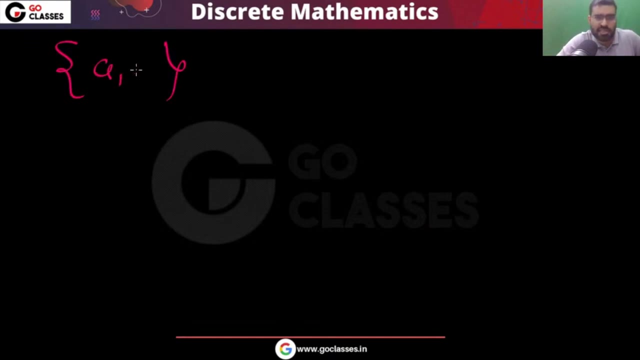 method. this is the most efficient method if you use the venn diagram. okay, most efficient for many questions. let's move on the last topic. the last thing that is see, you can notice that set is uh, settle. we represent the set like this: yes or no, and order does not matter. set is a collection of unordered 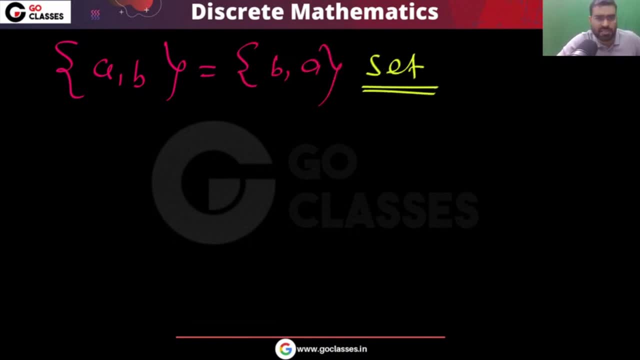 elements. so this type of thing is called set. set is a collection. set is a structure in which order does not matter. remember, set is a structure in which order does not matter and also repetition does not matter. so set is a collection of unordered, distinct elements. this type of structure. 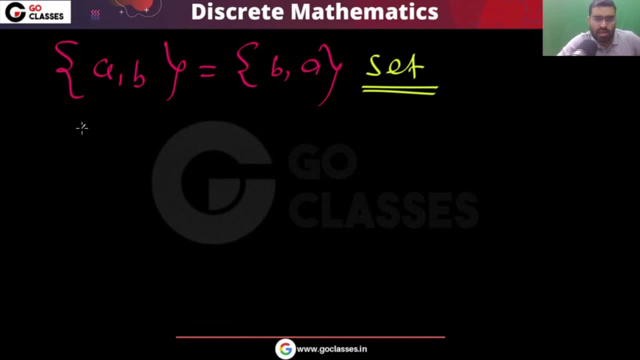 is called set, in which order does not matter, and also in a set this does not matter, like a, b, a, a comma b, comma a that is same as b, comma a that is same as a comma b. that, okay. so this is the definition of set. so set is a structure in which repetition does not matter. set is a collection of 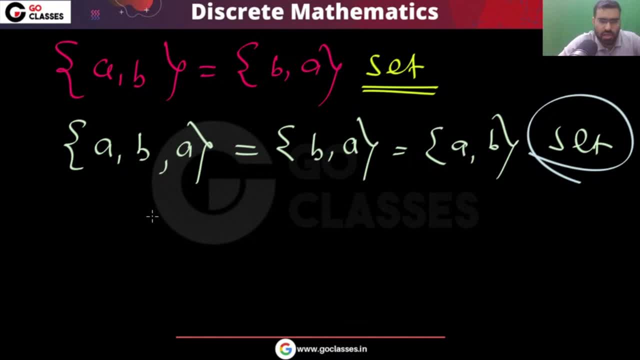 distinct elements. okay, you can ignore the repetition, you can remove the repetition. so, and also, order does not matter. so this is this type of structure is called set. now there is something called, there is a something called sequence. in sequence, order matters, repetition also matters and order matters. so in a sequence, 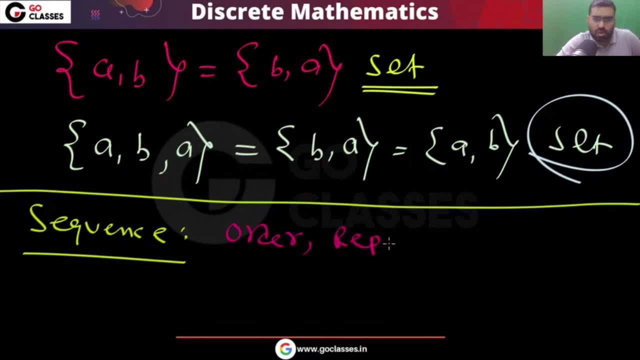 order comma, repetition, both matters. there is something called sequence, this concept of sequence, order comma, repetition- both matter. okay, both of these things matter. what it means? sequence simply means, for example, if you have one, one, two, two, this sequence is different from one one. two, this sequence is different from two one, one: this sequence is different from one one. 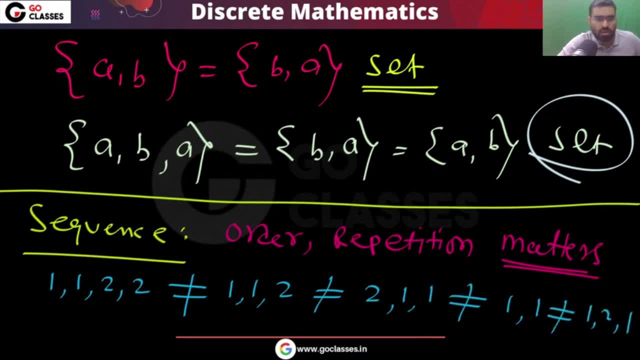 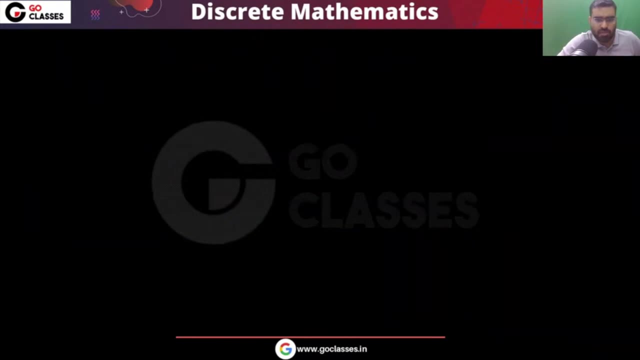 this sequence is different from one, two, one. so all these sequences are different. remember: this sequence is different from this sequence, this sequence is different from this, this sequence, okay, all these sequences are basically different. so in a sequence, order also matters, repetition also matters. this is an important point: the definition of sequence. so please understand that, if you have, 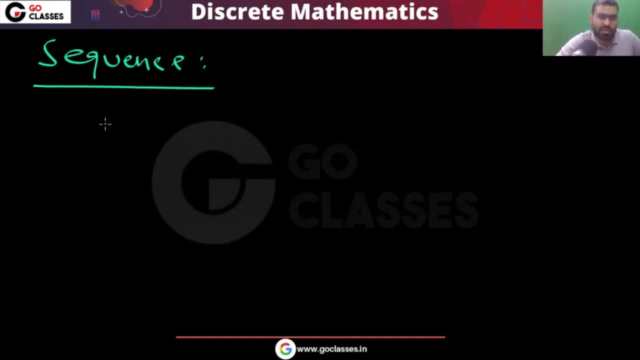 this sequence. if i say sequence, like, as i told you, this sequence, look at this sequence: a, b, c. this sequence is not same as b a c. this sequence is not same as b comma, b comma, a comma c. so these in a sequence. all these things matter. okay, now, once you understand the sequence, what are the sequence sequence? uh, in the sequence. 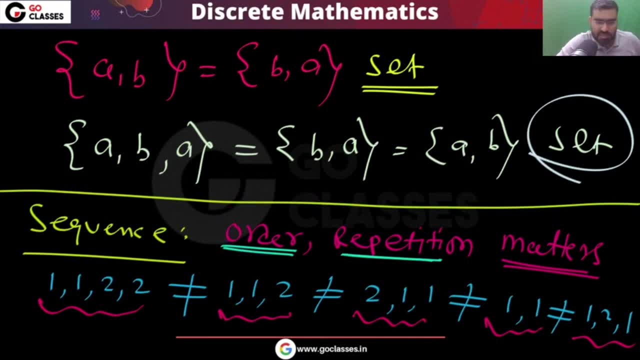 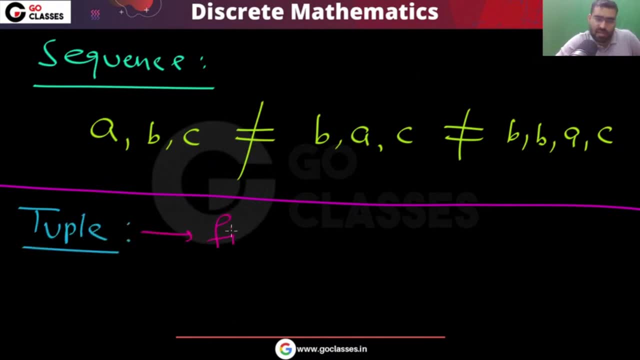 order matters and repetition matters. both the things matter in a sequence. now let's see the next concept, that is tuple, tuple, tuple is basically a finite sequence. what is a tuple tuple is a finite sequence. this sequence can be finite or infinite. see, this sequence can be finite. 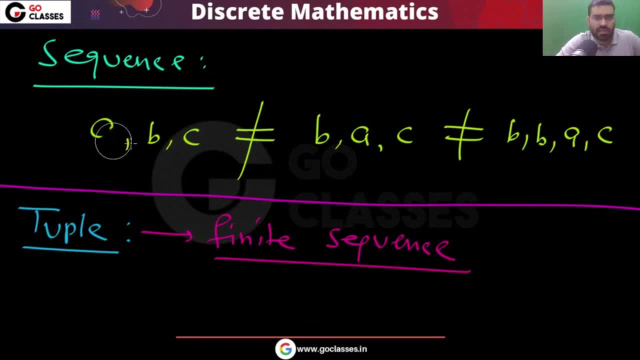 or infinite, as i told you, for example, you can, you can take another example. let me give another example. like: this is a sequence: one, two, three and so on. this is the sequence of natural number. okay, so this is a sequence, remember. so in a sequence, in a sequence order. 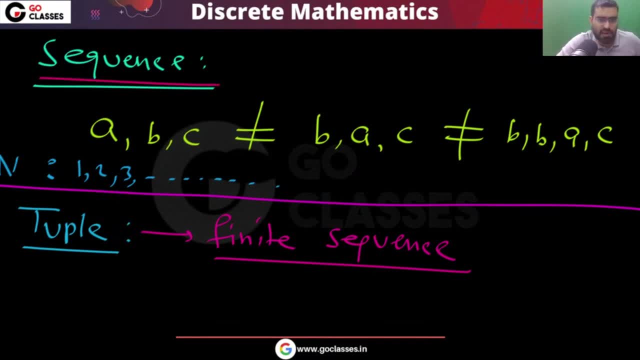 matters, repetition matters, so sequence can be finite or infinite. what is a tuple? tuple is a finite sequence. okay, this is called tuple. like, for example, if i give you this 1 comma 1, or i can say this 1 comma 2, this is a fine, this is a tuple. this is different from 2 comma. 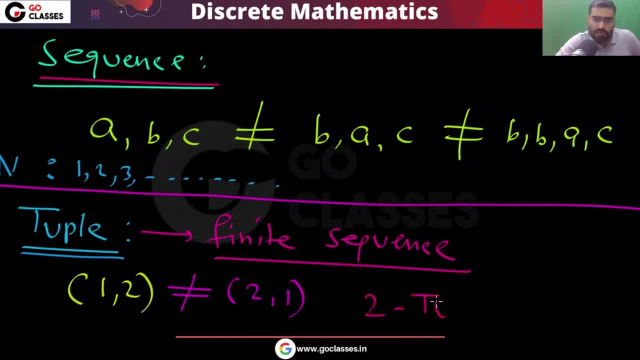 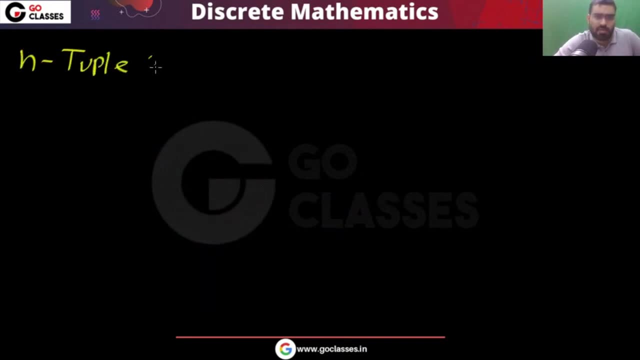 1. okay, this is called 2 tuple because there are in this tuple, there are two elements, so this is called 2 tuple. like, for example, what is n tuple, what is n tuple? n tuple is something like this: you have total n elements, you have total n elements. remember, they can be same. 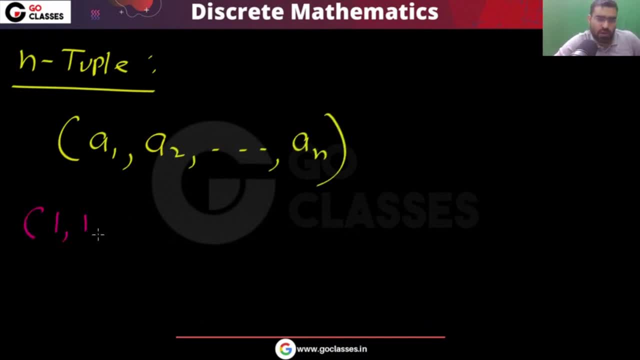 or different. for example, you can notice that if you have 1, 1, 2, this is a different from 1 comma 2. remember, this is different from 1 comma 2 comma 1. remember, this is 3 tuple. this is a 3 tuple. this is a 2 tuple. this is a 3 tuple. 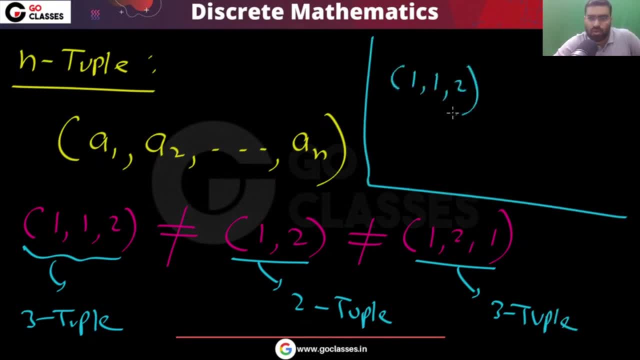 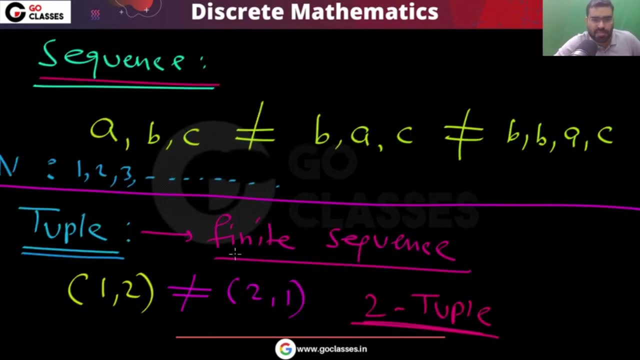 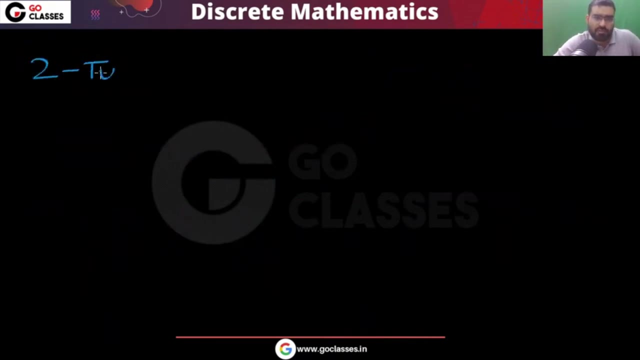 also also this one, one, two. this is different from one to one. okay, these are different because order matters. so remember, tuple is just nothing but finite sequence. finite sequence is called a tuple, very simple point. now. this two tuple is called ordered pair. this two tuple is called what we. 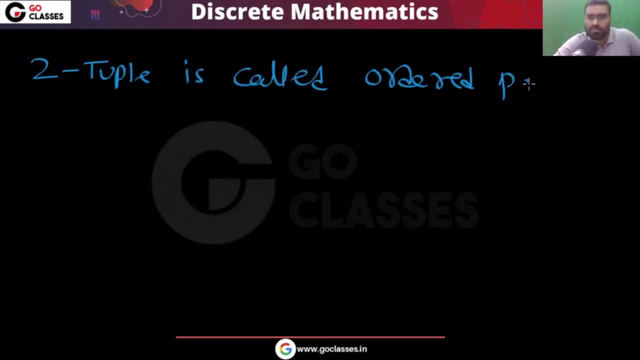 call it, we call it ordered pair. this is called ordered pair. so what is the ordered pair? what is this ordered pair? ordered pair is simply i can say like, for example, a comma b, this is a ordered pair and remember, this is different from b comma a. for example, i can say this: 2 comma 1. 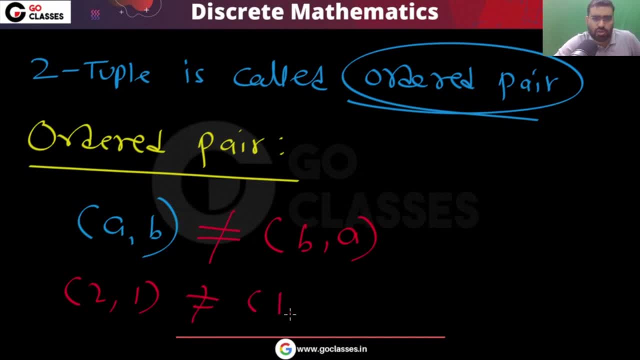 this is different from 1 comma 2, okay, so ordered pair. ordered pair means two elements, so you can see this is also ordered pair. this is also ordered pair. okay, so these are ordered pairs. remember: this ordered pair is different from so here. this is two tuple, this is one tuple, so these are different. i hope all. 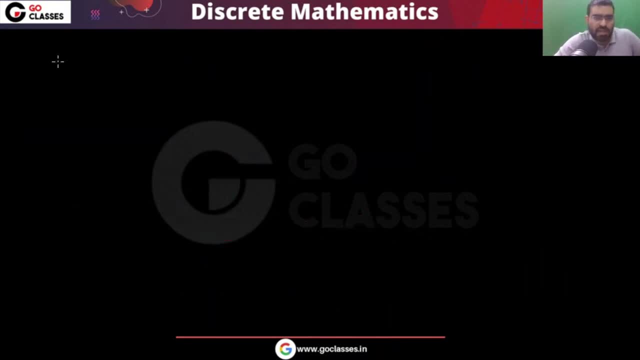 these points are clear. so what is the ordered pair now? when can i say two ordered pairs are same? a simple question i am asking: tell me, if a comma b is same as b comma a, then what? what it means? if a comma b is, then what can you say then? what do you? what you can say, tell me, if two things. 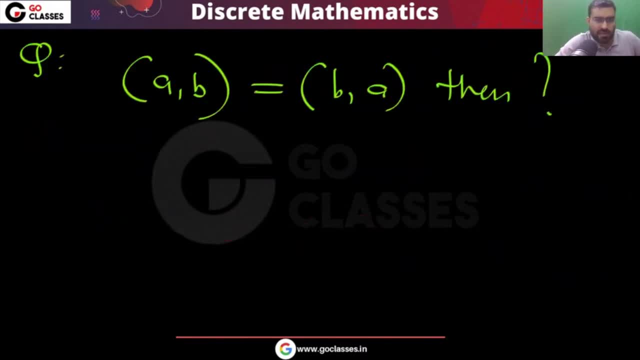 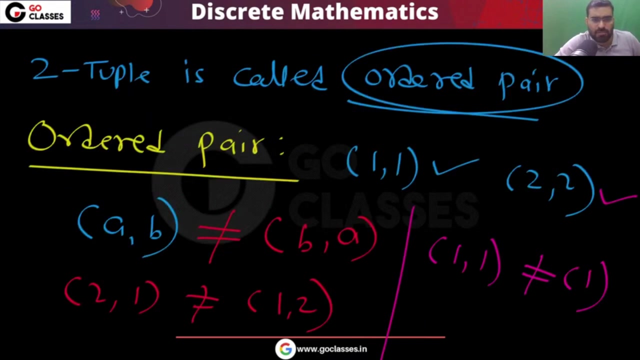 are same, like a comma b, this ordered pair is same as b comma a. then you can notice that this a must be same as b and this b must be same as a. right then, or this would happen: that a must be same as b and b is must be same as a. so then i can say that a will be equal to b. okay, in this situation, 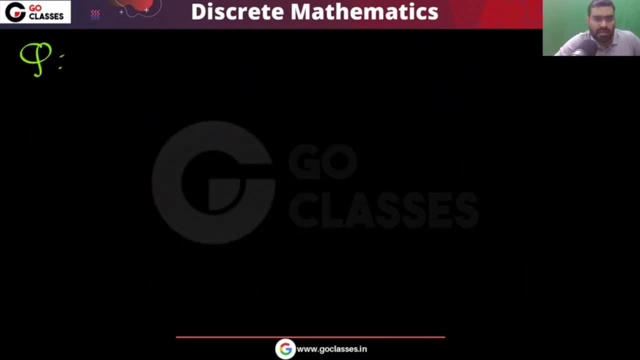 a will be equal to b. similarly, if you have- for example, if you have- a comma b comma c that is equal to d comma e, comma f, then what will? then what will happen? if you have a comma b comma c that is equal to d, comma e, comma f, then what will? 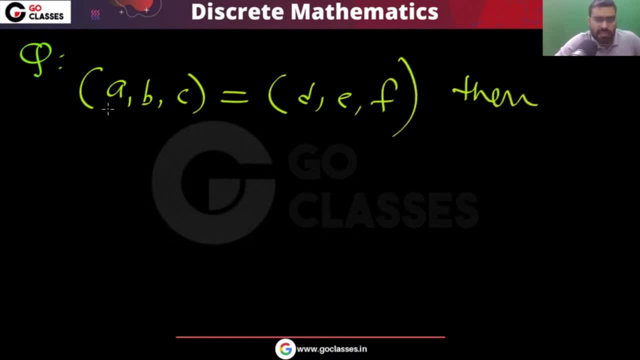 then what will happen? if you have a comma b, comma c that is equal to d, comma e, comma f, then what will then? what will happen if you have a comma b, comma c that is equal to d, comma e, comma f? then what will then then? what it means then? it means that it simply means a is equal to d, b is equal. 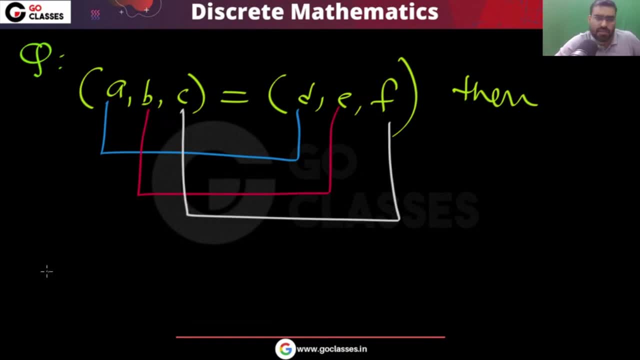 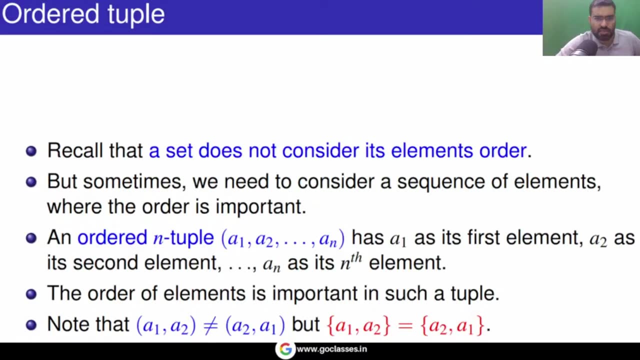 to e and this c is equal to f. right, so it simply means that a is equal to d, this b is equal to e and this c is equal to f. so this is. these are some points that you can very easily understand. so what is this? in a set order does not matter. set in a set order does. 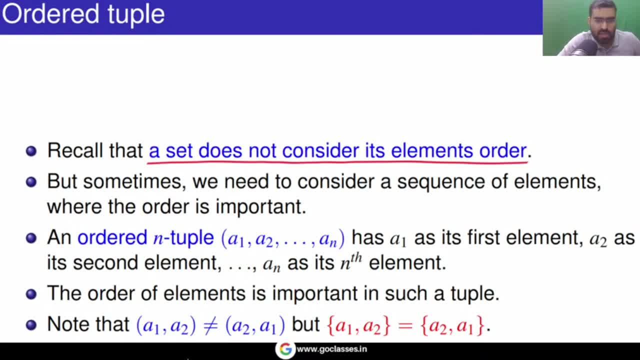 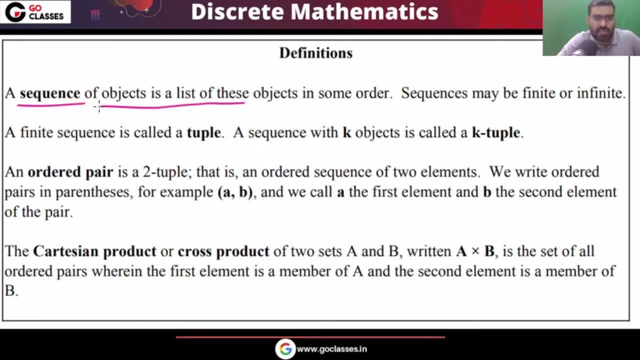 not matter, but but remember, in a sequence order matters sequence. sequence can be finite or infinite. finite sequence is called tuples, so you cannot. sequence of objects is a list is a list, okay, of objects. this may be finite or infinite. what is a tuple? tuple is a finite. 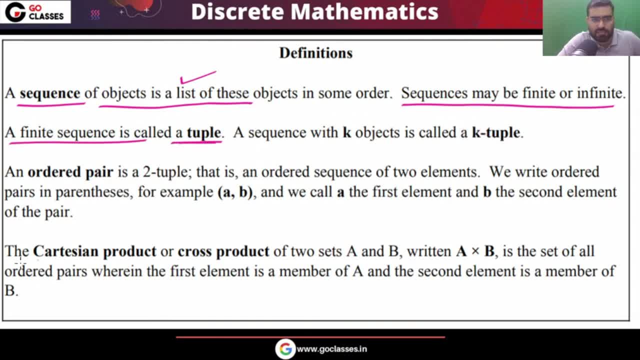 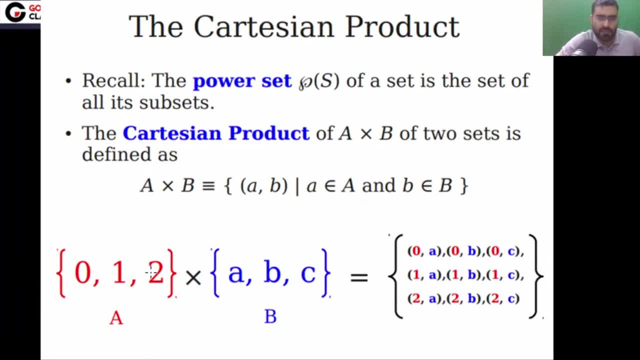 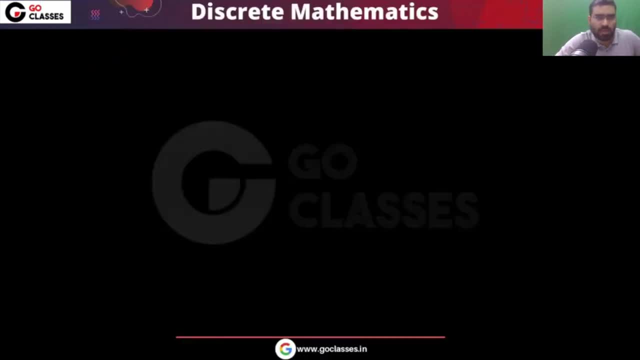 sequence. so, for example, k tuple means k elements. they can be same or different. okay, now the last operation on set is cartesian product. if you have two set, zero, one, two, a, b, c, one is the product. so if you have two set, this is the last topic. the last topic is cartesian. 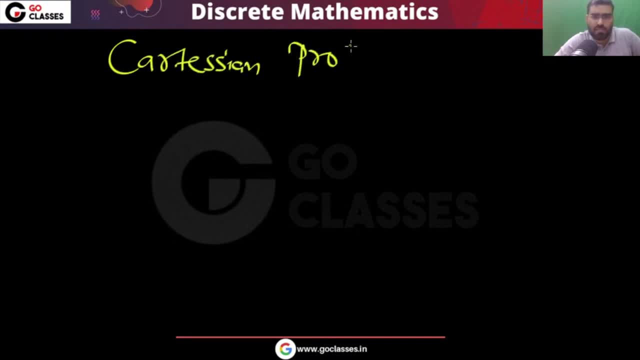 product, cartesian product of two sets. it is also called cross product. you can also call it cross product. so what is cross product of two set? if you have set a, set b- these are two set- then what their cross product will be, cross product will be a set. remember set. the cross product also will be a set. it all it will also be. 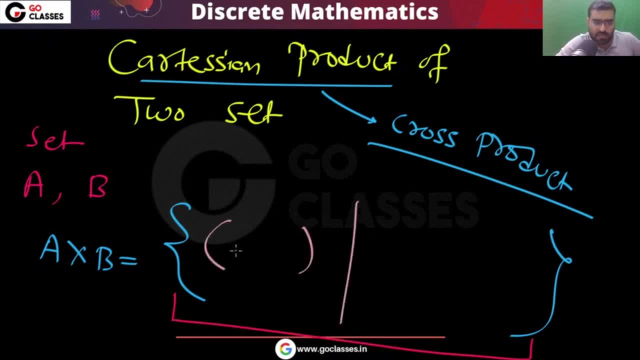 a set in which you will have ordered pairs. the first element will come from a, the second element will come from b, because you are doing a cross b, so first element will come from a and the second element will come from b. this is the cross product. for example, if you 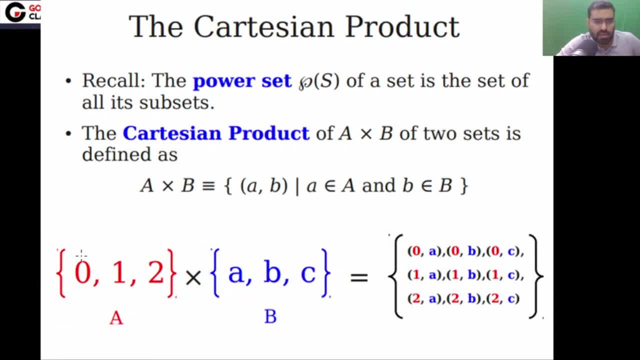 if you have 0, 1, 2 cross product a, b, c, then you will have ordered pairs 0 comma a. this ordered pair 0 comma b. this ordered pair 0 comma c. this ordered pair 1 comma a. this ordered pair 1 comma b. this ordered pair 1 comma c. this ordered pair then 2 comma a: 2. 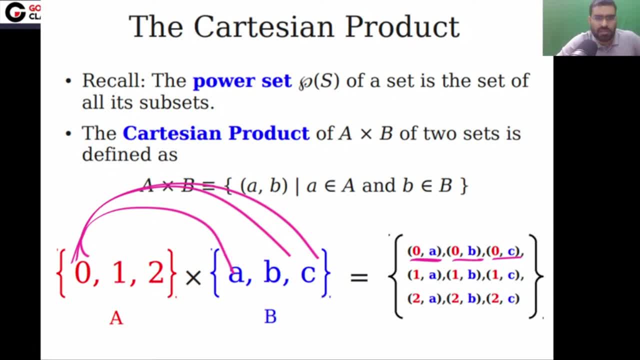 comma b, 2 comma c. so you can notice that very simple. this is the definition of cross product. so if you do, if you have two set, a comma b, their cross product will be set of ordered pairs. remember the cross product also will be a set in which you have ordered pairs where 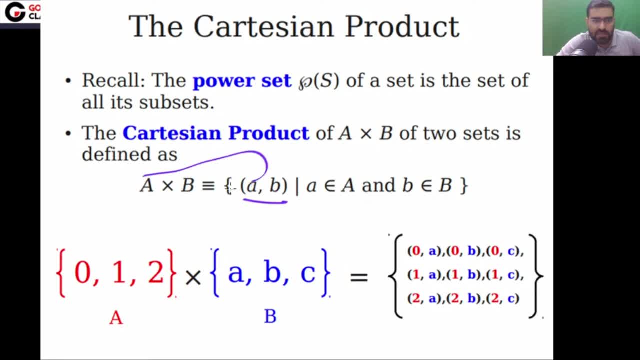 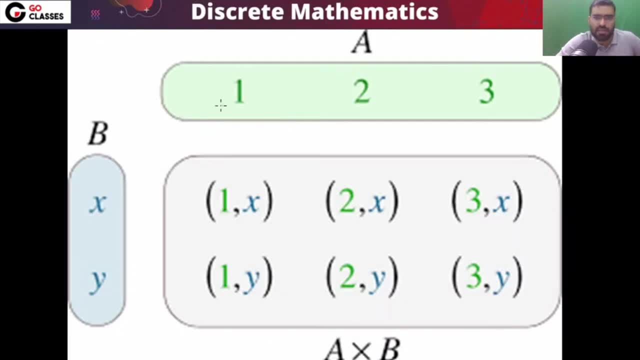 the first element in in the ordered pair. the first element is coming from a and the second, The second element is coming from A, the second element is coming from B. so this is your Cartesian product. You can easily see here: you have a set A, you have a set B. then what is the cross product? 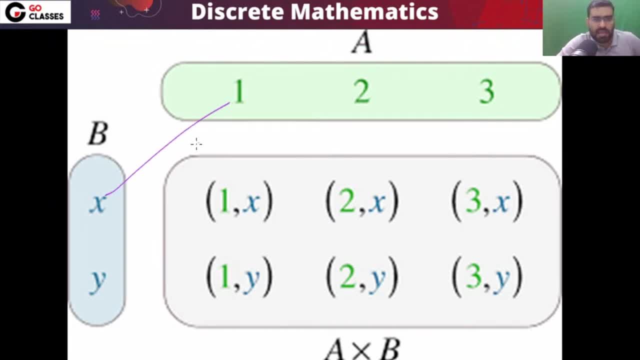 A cross B. A cross B means every element of A pair with every element of B, Every element of A pair with every element of B. So you can notice 2x 2y And every element of A pair with every element of B. 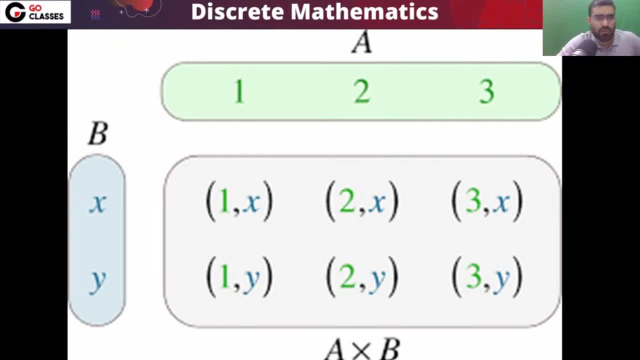 This is called. this is your A cross B. What is B cross A? If I ask you what will be B cross A, So B cross A? if I ask you that, then what that will be. So if I ask B cross A, B cross A means now every element of B will pair with every element of A. 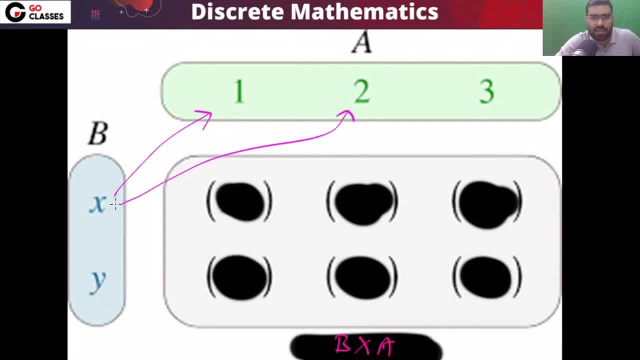 Okay, every element of B that will pair with every element of A, So it will be something like this: You will have x comma 1, x comma 2, x comma 3, y comma 1, y comma 2.. 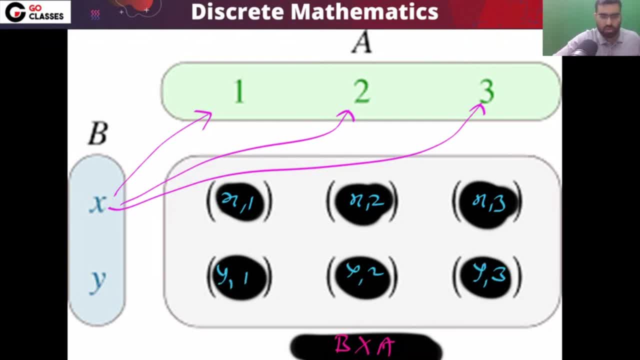 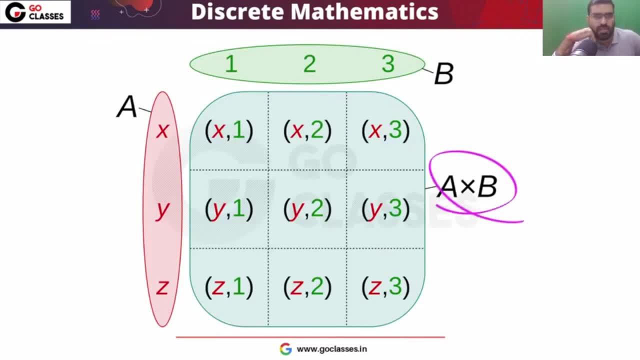 y comma 2, y comma 3.. Okay, so this will be your B cross A. So this is the definition of Cartesian product. If you have A comma B, A is xyz, B is 1 to 3. Then A cross B, that will be like: 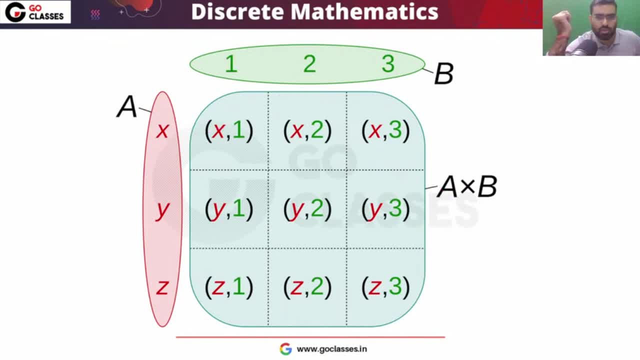 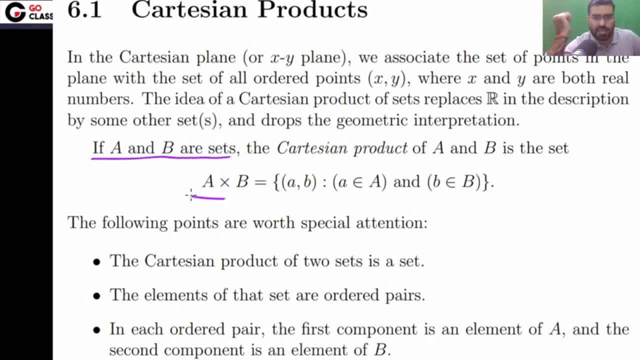 x1, x2, x3, y1, y2, y3, z1, z2, z3.. This is the definition of cross product. So what is cross product of 2 set? If A comma B are set, then cross product is also a set. 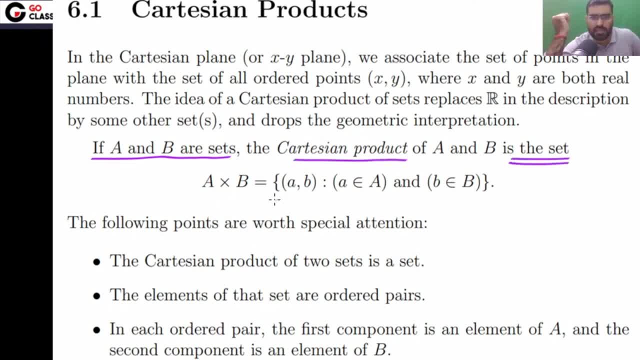 The cross product, the Cartesian product, is also a set. It is also a set. Okay, it is also a set Which contains ordered pairs. The first element is coming from A. the second element is coming from B. Okay, so it contains ordered pairs. 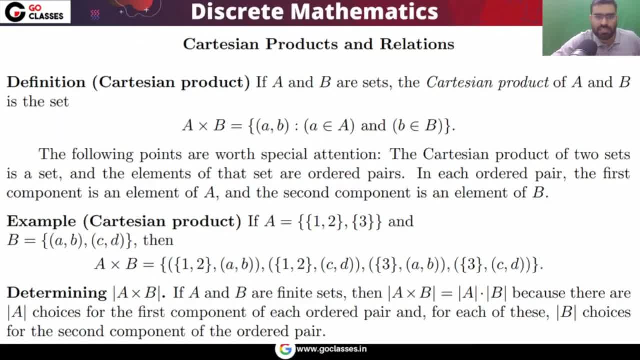 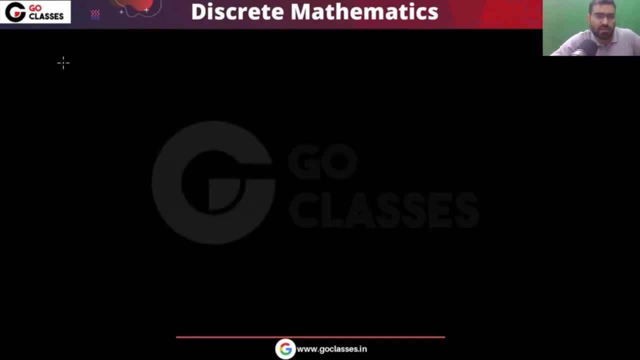 Very simple. So this is the complete summary of our set chapter. And simple thing. finally, what is the if you have 2 set A note, If A comma B, if A cardinality is n and B cardinality is m. 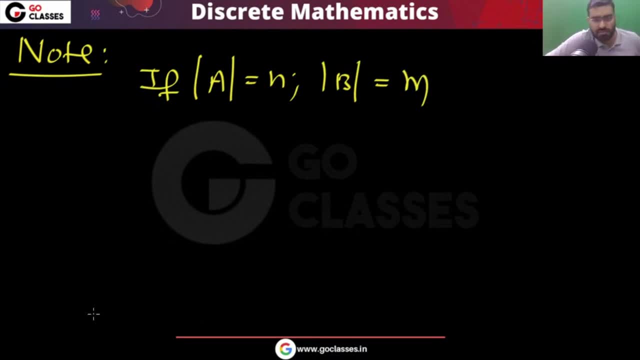 then tell me how many ordered pairs you can create. Tell me how many ordered pairs Means what is the cardinality of A cross B? The cardinality of A cross B, what that will be. Remember the cardinality of A cross B. 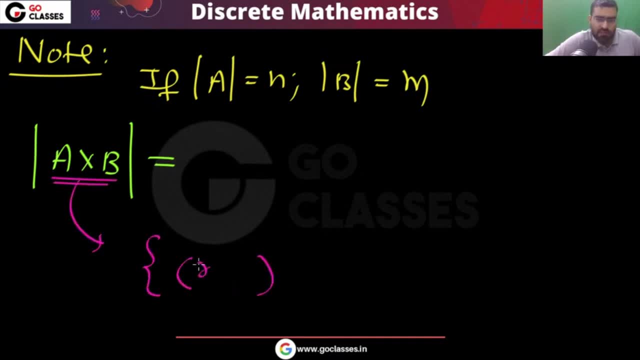 if you notice this, A cross B has ordered pairs Where the first element will come from A, the second element will come from B. This first element will come from A and second element will come from B. Okay, this second element will come from B. 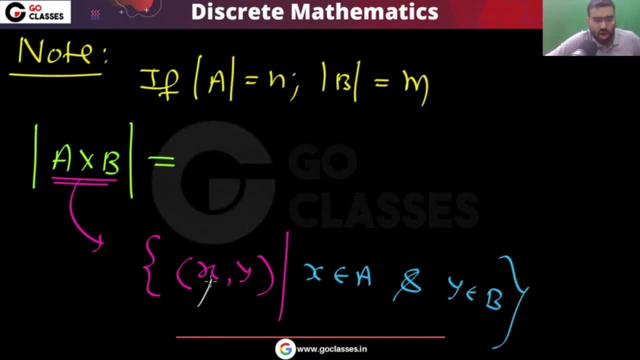 So for this first element, how many choices we have we have. this first element will come from a. so for this we have n choices. for the first element, there are n choices. for the second element, there are m choices because the second element is coming from b. okay, so first element is coming from a, second element is coming from b. so finally, how? 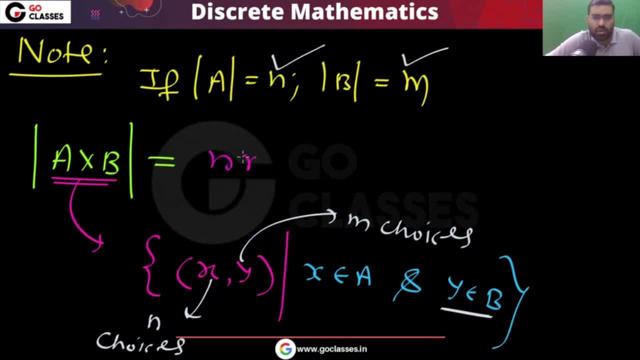 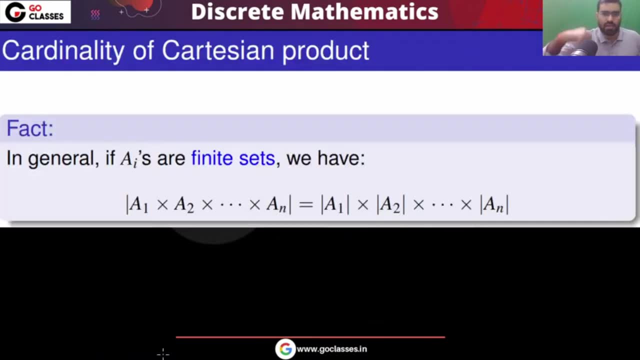 many ordered pairs you can create, that will be n into m, so your answer will be n m. okay, i can say n multiplied by m. so if you, if i ask you what is the cardinality of a cross- a1, cross a2, cross n, so that will be cardinality of a1 into cardinality of a2, cardinality of a3 and so on. so basically,